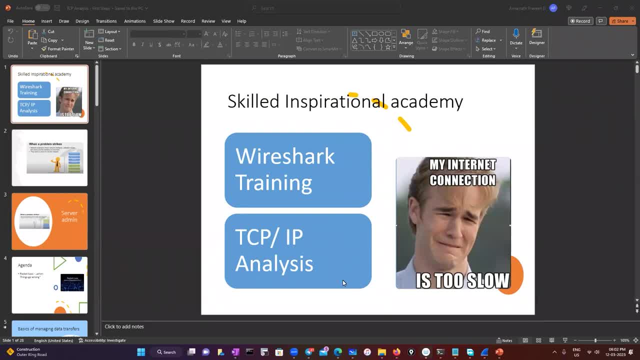 of this class would be. once you finish this demo session, you would have a solid understanding of what is TCP and what exactly. you know what is inside the TCP packet, because we heard of a TCP But we know very few people, So They might, you know, peel out every TCP flags and TCP parameters. that, so many parameters. 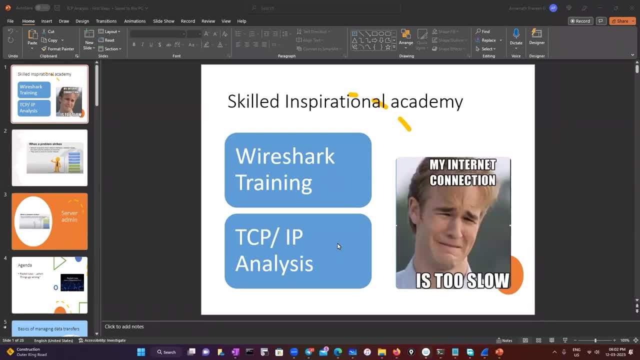 that may be. you know for few people that they may not heard about this TCP flags and TCP parameters before. So this particular class, the biggest takeaway is you would get you know a complete understanding of how TCP IP works with every parameters and why those parameters are used. 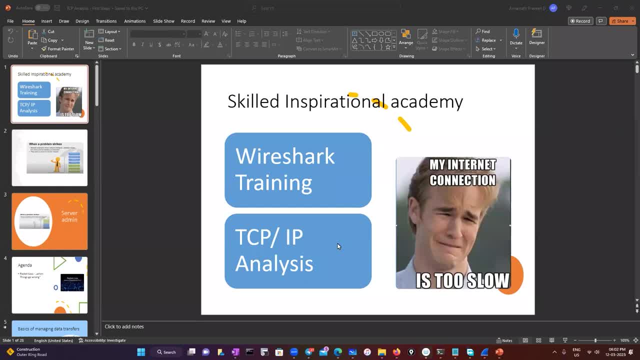 And in the modern communication why this TCP is so important for the, especially for network troubleshooting. Yeah, this is all about the biggest takeaway of this class. So once we finish this class you will be so confident and you will understand better about TCP IP analysis. I hope everybody. 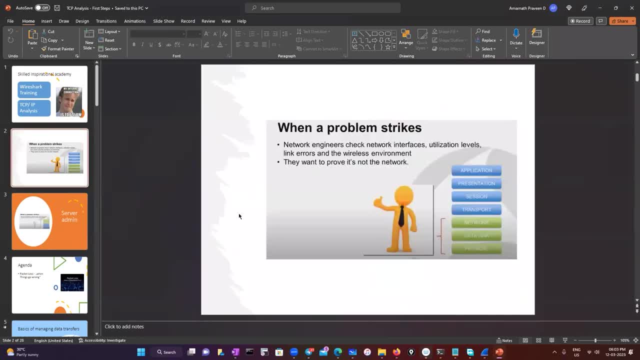 will start enjoying this class. So before start with, let me explain a scenario. we usually encounter this issue. Okay, Networking is the one common backbone where all all the teams you know they keep barking about this problem. They always complain the networking team for this, any kind of you know, performance issue. 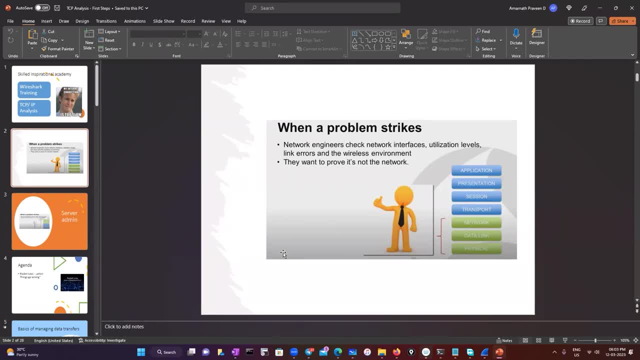 It can be a application issue as well. So people might have might have come from a different background and I want to give you an overview of OSI model. So we all know the OSI model. it got you know seven layers, So the main, the core layer, what we are going to look at here is transport layer. 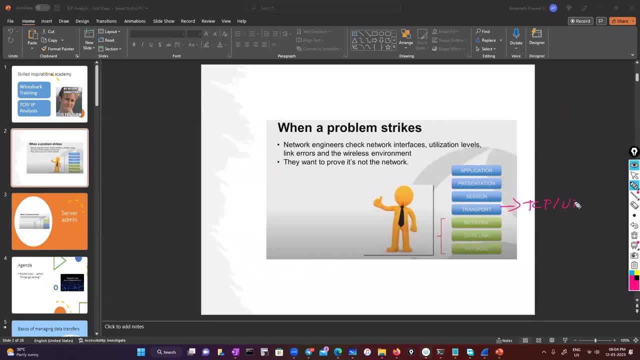 So here works this TCP and UDP and we all know about that. 10. We say TCP is very TCP connection oriented and this is very reliable protocol. Why is that? what is the mechanism That's, you know, outstanding when compared to UDP? Why TCP is so reliable. 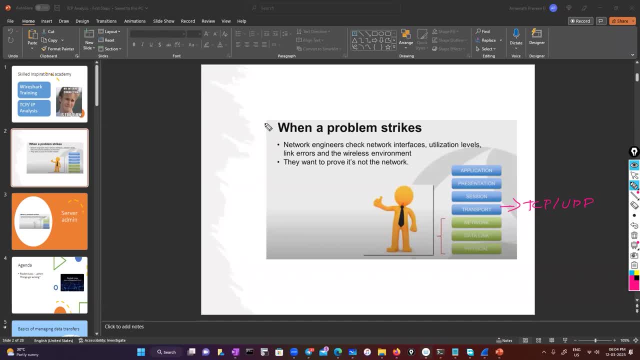 Why white people call it as so reliable connection. What is the meaning of it? So when there is a problem generally, what the network engineers they have the maximum possibility to look around for an issue, What is the cause of an issue, How do they start with and how they come to a conclusion that 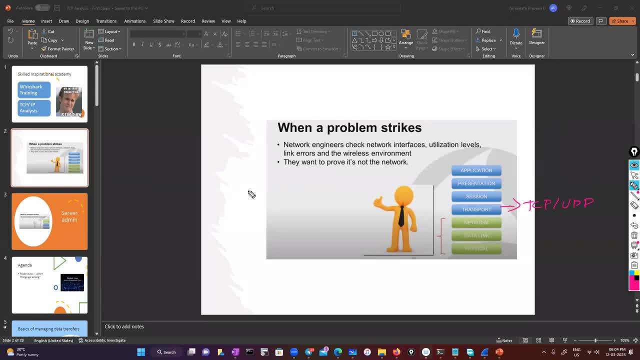 okay, this particular problem is not with the network, It is a problem with application. So to get a complete insight about a problem, I don't think with a router, CLIs and firewalls. definitely we would see the TCP SYNAC. That's a stateful device, right? 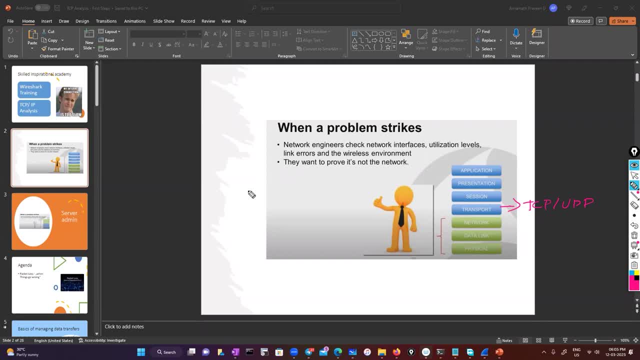 So it maintains a TCP session, That's for sure. Firewall is capable of it. But to peel out what is inside every TCP parameter, So here comes the wireshark. So you cannot do that, So in the firewall to the maximum. 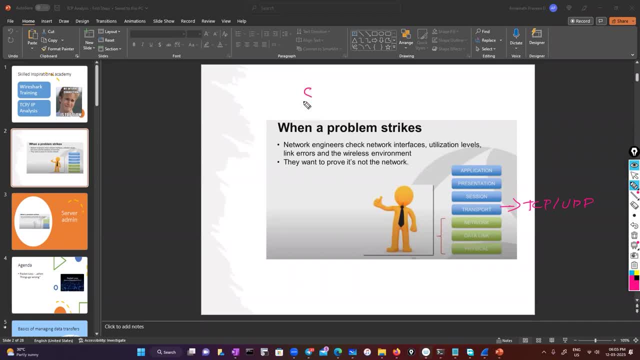 what you can do is: okay if a connection is established between your source to destination, So we can say it is a TCP or UDP And firewall will give you more control of. okay, this is a stateful connection And you can see the TCP connection establishment. 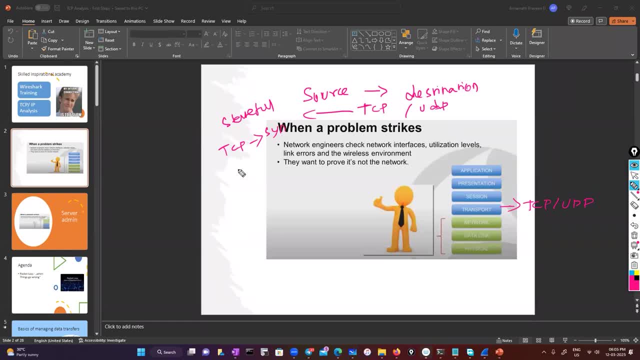 We call this as TCP SYN And TCP SYNAC. right, Once these two connection established, then we can say, okay, this is an established TCP connection. So this is a maximum, you know, control we have with firewall, But with the help of wireshark. 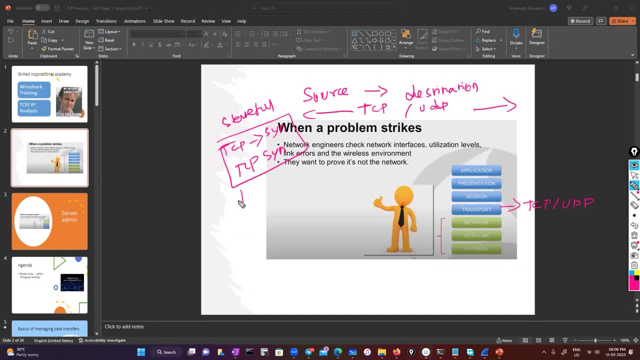 what we can do is: okay what is inside the TCP packet. So it is something like you peel out every parameter in the TCP and you will see what exactly happened. So if there is a slowness issue, there can be a multiple problems, right? 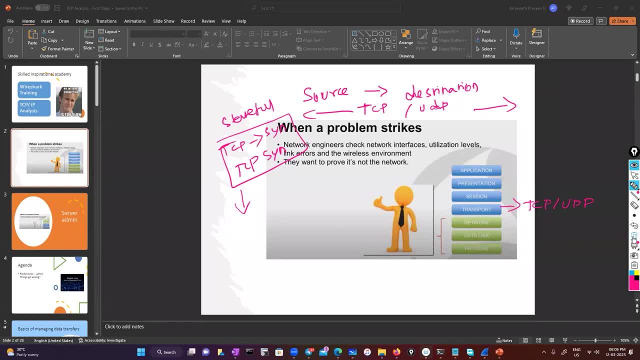 So, but to figure out all that, the primary is very key thing here. So you cannot just blame: it is because of an application. So to prove that, you have to do some basic checks, as you have to. example, you got your. 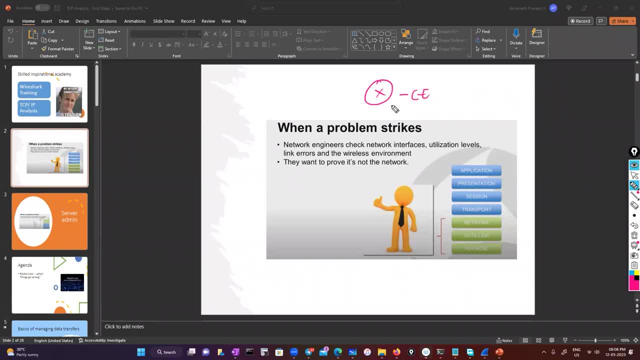 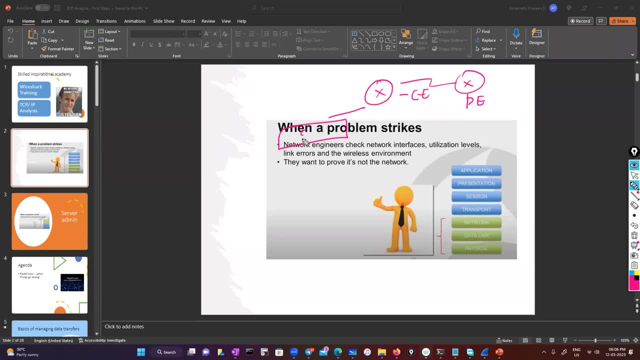 And you have a BGP peering with your provider. And you have a BGP peering with your provider And you got your core switch Very simple design here. So we got a couple of pieces connected And when the traffic is initiated from the client. 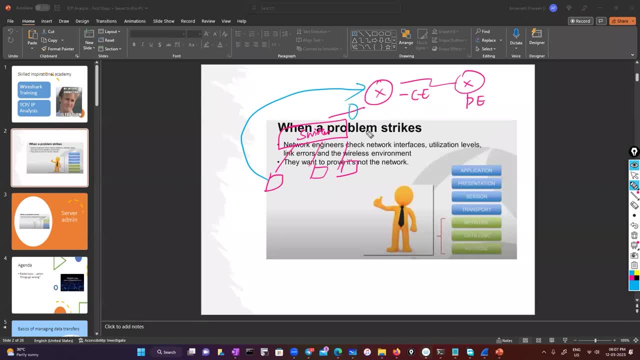 So you have to check here right, Even though your bandwidth is too good. you've got your hundred Mbps link- It's a fat pipe- and you've got, you know, a good bandwidth connection. that's in your office, but still people are complaining about this slowness. 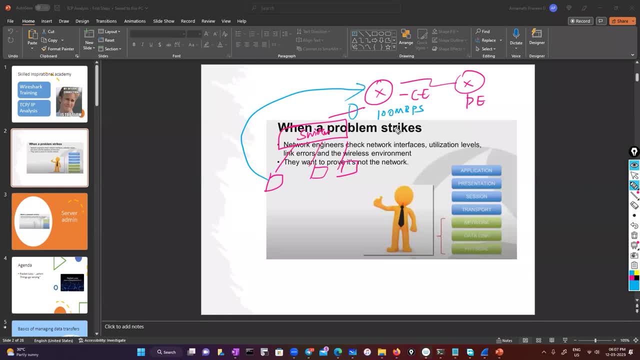 Issue so you can check the utilization. There are many monitoring tools to do that, So one we use as a SolarWinds, where we can find the utilization of a particular link So you can see this internet link is choked and how to find all that. 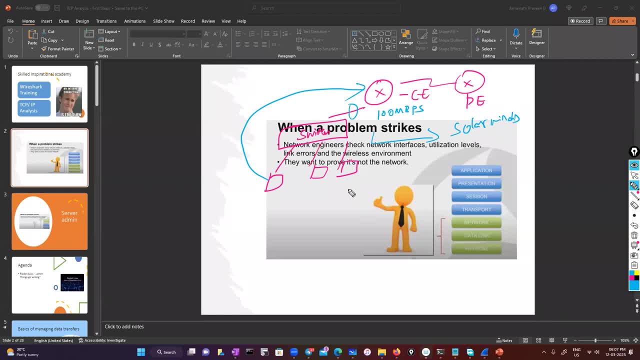 Right. So to prevent this in most of the enterprise design what they do, they use, you know, QS techniques. Uh, so we'll see where exactly the QS marking happens and how we can find out in, But I'm just giving an overview about QS. QS is quality of service. 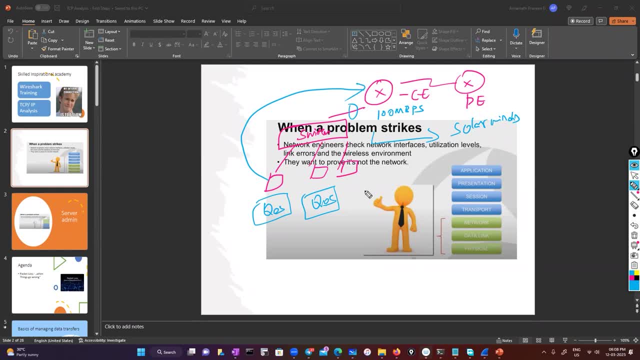 That is something like you are prioritizing your traffic. So, uh, maybe a few people they may heard of this, but again, the quick overview is: inside the IP header You can do a marking That is something called as IP precedence value. 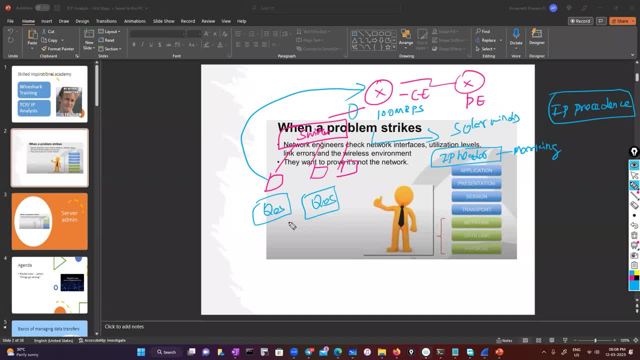 That is, you are prioritizing the traffic. That's the main objective. So you are marking your traffic Right, You are prioritizing your traffic. So if from the switch level, if you do uh QS, that should be visible under the layer two. 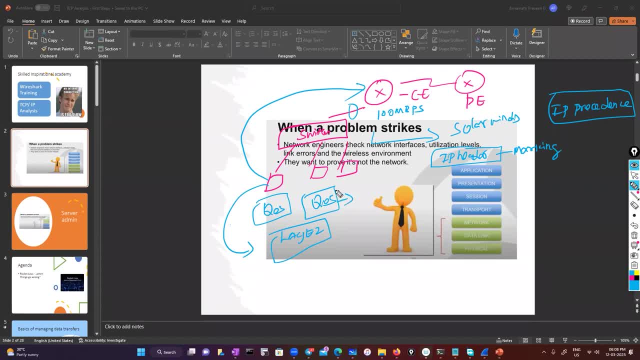 So what is the quality of service you are using and how you are prioritizing your traffic? example, your priorities in your traffic, something like this, the priorities in your voice- and you are prioritizing your uh data. traffic says just an overview. 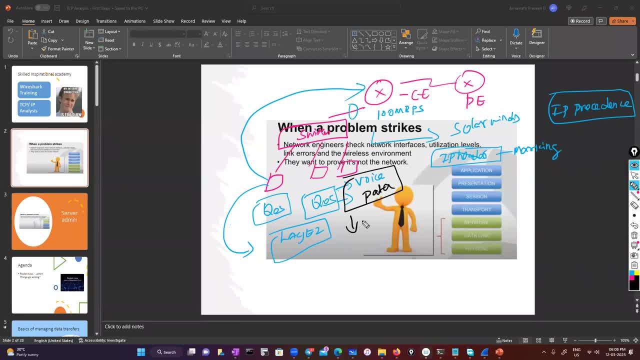 This is not much with networking to you know. we'll look deeper inside the Wireshark, So I want to give a glimpse about all this. So I'll mark the packets and I'll give a priority for it. For example, for priority, I'm giving a priority 10, and for data, I'm giving priority five, because voice traffic is very crucial. 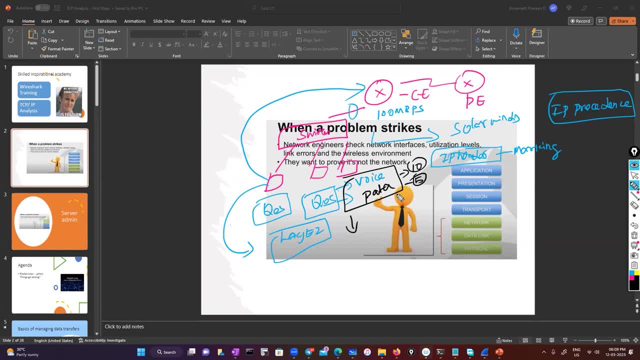 And that is vital for the network. So people should not be disconnected when they are on phones, when they are using their teams. So the priority is higher for voice. So you can peel out all your QS information inside the wire Shark and you can see, even though, if you applied a specific policy to this switch, this L2 switch, but still, if you can see from the Wireshark, if you take a capture from your PC and if you, you know, do a packet for capture from the switch and if you offload all your traffic back to the client PC, you will come to know whether the traffic is actually. you know the all your packets are being marked with your QS marking. 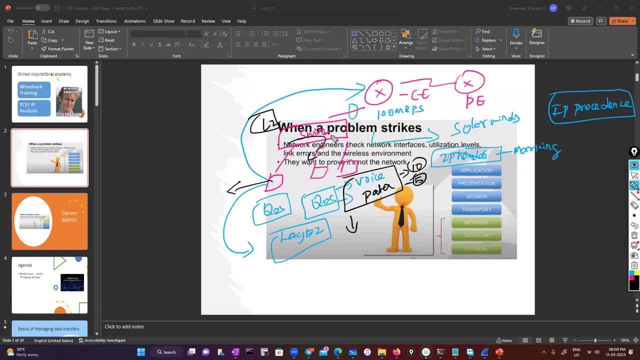 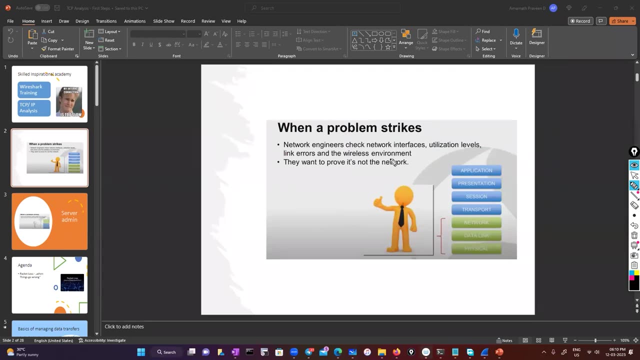 That's exactly configured on your switch. That's been applied to The specific interface, So you'll get all that kind of you know deep insights about that using the Wireshark. Okay, That's fine. So now I did my um. I know basic checks, something like I checked my uh internet link and the utilization levels, right. 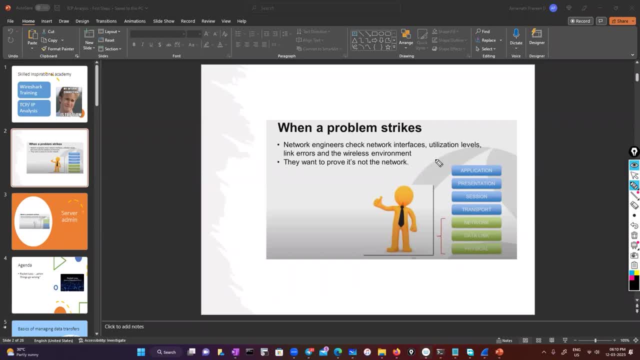 It can be either from from your switch or it can be from your van. That is the only possibility, right? So if you've got your route or something like this and it is connected to a switch and you've got your PC, 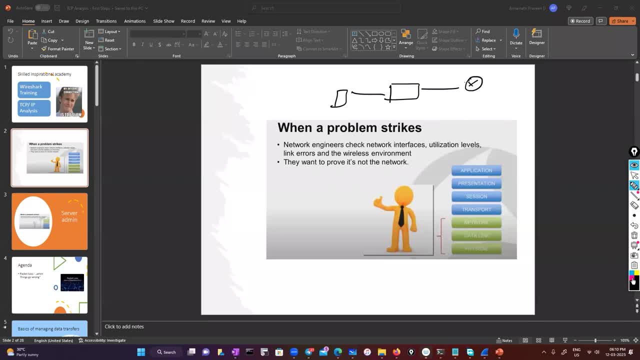 This is connected here, So it it can. it could be either this end or this end or this end, right, So these, because this is connected to ISP, you'll you'll check all these three ends and you'll look for interface errors, utilization levels, right. 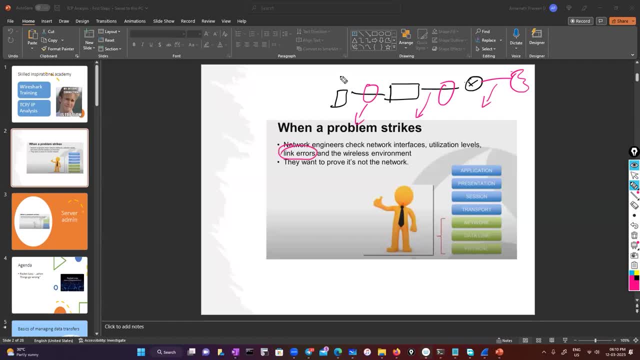 If there is any errors- there's something like a physical issue- You will see the CRC errors keep increasing And, um, if you see any kind of utilization here, it's your bandwidth is choking. So if you're looking for 75%, you'll get to know about all this with your monitoring tool. 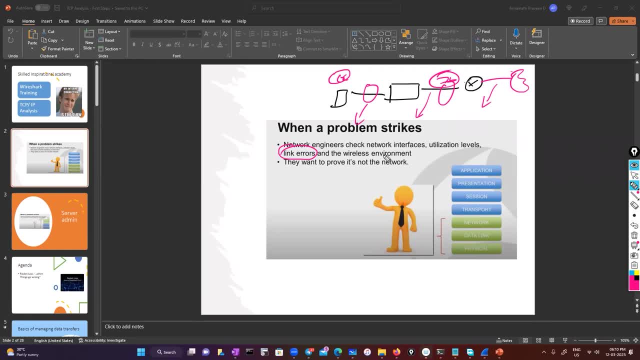 That's fine. So I have checked everything. Now the scenario is I have checked every single possibilities, what I have, but I couldn't figure out where the problem is. So now I am concluded that, okay, all my layer, all this below three layers, my physical layer is good. 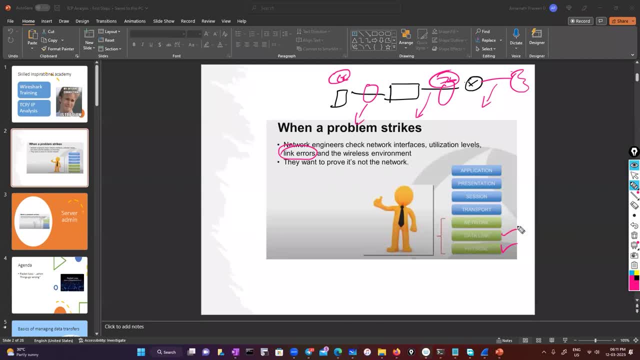 My data link layer is good, My switches actually forwarding all the frames- That's no problem with the switches- And my network layer is also clean. There is Quite normal And there is no CPU utilization on my router or no CPU utilization on my switch, as well as my PCs. 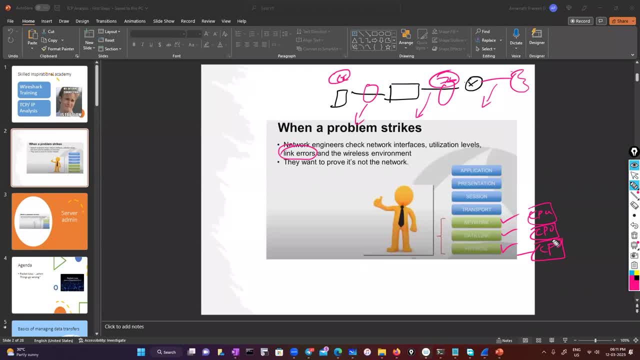 Right, So all the basic checks you have to do. that is very important, because network is just like an highway, So if there is a congestion here, then apparently your application will be dropped. Agree, So that's how it works. So my highway is clean. 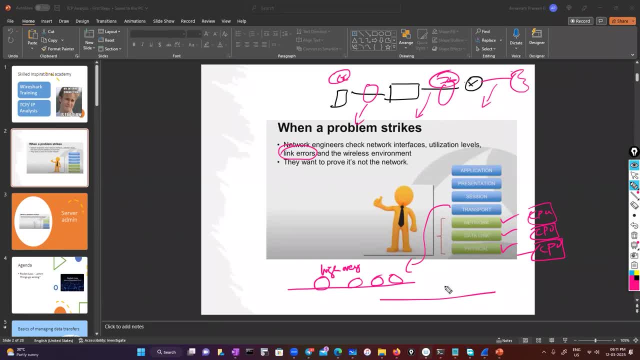 My cabling is fine, My switches, My router is fine, Your PlayStation is fine, There is no problem from the network perspective at all. but how do you say, or how, how do you convince? I would say it is a convincing- how do you prove exactly that? 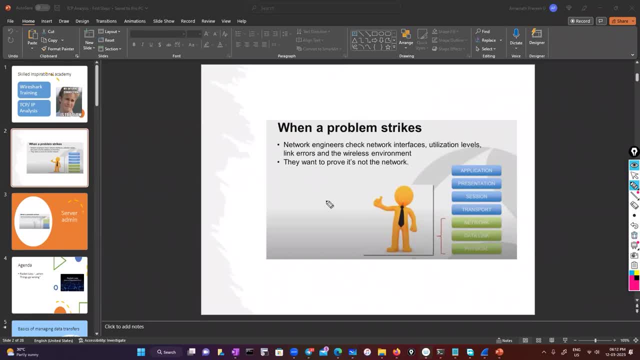 Okay, This is not my networking issue, that that's a problem, right, Because people they say okay for all good, then why still my connection is bad? Why? why I'm dropping my packets? Why why in the communication is not so healthy and faster? 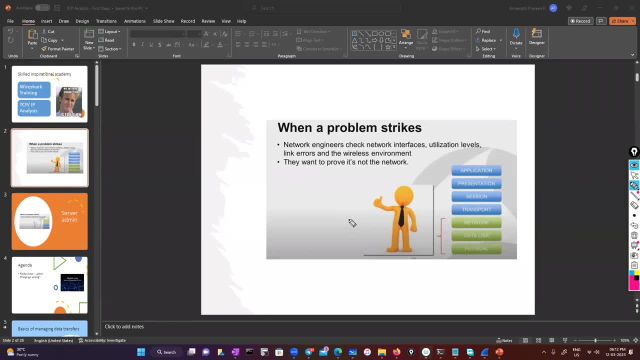 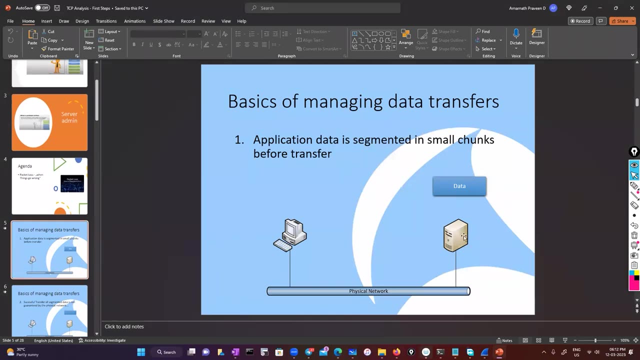 So it's, it's pretty slow. So this is all the application slowness, Generally the people. they complain about this. So how, how do I overcome this problem? to know about that, I have to give an overview again about the TCP. 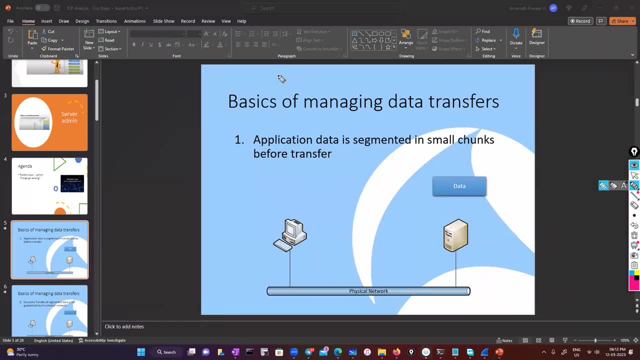 So it is not that if I'm saying if I send a packet from one source to destination, I'm not pushing the packets without any mechanism. So how I? I know how I can guarantee all the packets. Okay, I know how the packet has been delivered to the destination, how I can be confident enough for about this packet delivery process. 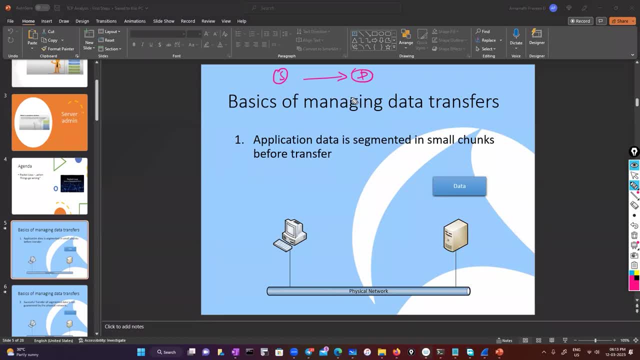 So, um, to rule out this issue, they have a protocol called TCP, that is called transmission control protocol. We say: but what exactly does so? for every packet it has its own database, is something like it. it make note of every packet that it sends. 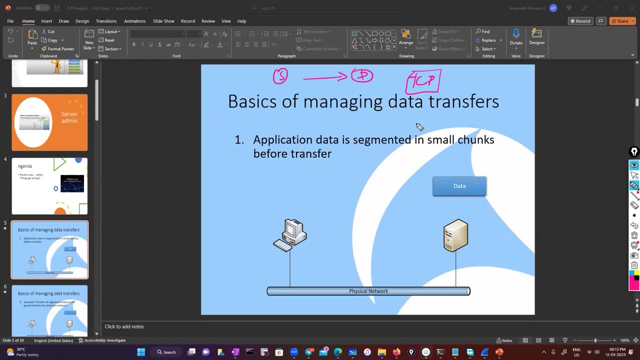 So how this mechanism exactly works. Yeah, this how the TCP parameters helps us. Uh, so, if I got a big data, so once one big data example. it is a 64 bytes data, but I cannot send send us a one single packet. 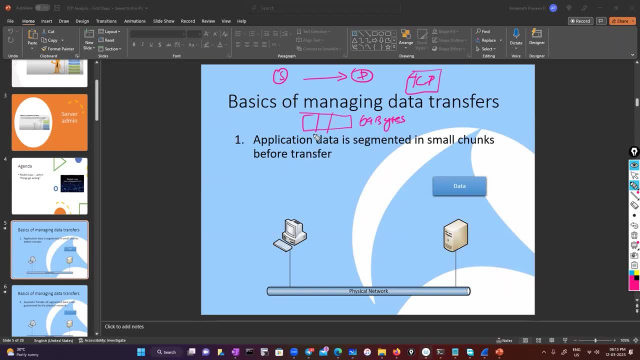 So I'm going to chunk this packet into small sizes. So for every packet I'm going to, you know, identify every packet using the sequence number. Why it is used. I'll show you there, but I'll give you an again an overview about that. 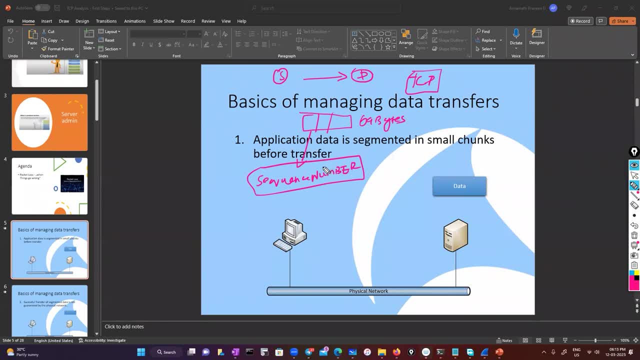 So sequence number. with the help of sequence number, I can track every single packet that's been sent from my source. example: This is a sequence number one and I'm going to send the second packet here. So my second packet is something like the sequence number two. 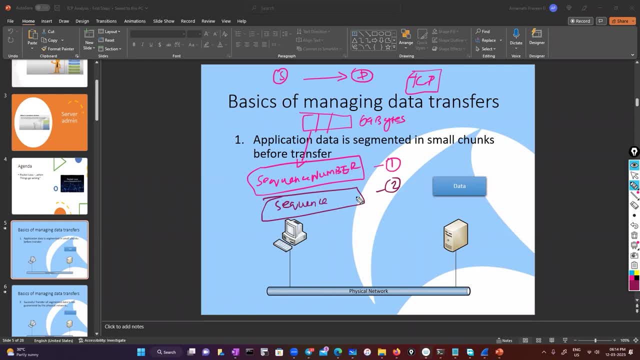 It's for justification For the demonstration purpose. the real sequence number is different. So this is the sequence number And before that, actually, if you do a capture, uh, using the wireshark and any any you know um analyzing tool, um, but one key thing you should understand about the: this wireshark will use a sequence number called us relative sequence number. 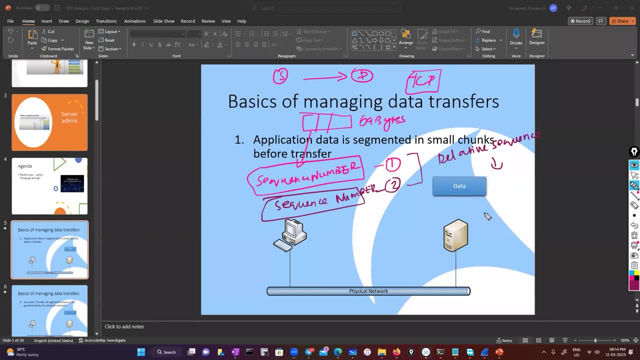 Why this is used relative sequence number is It's for, it's for um, very you know um. the administration is very simple. example: If you use your raw sequence number, it's very hard to follow the Packets. but if you use a relative sequence number, that is something you. it gives more control. 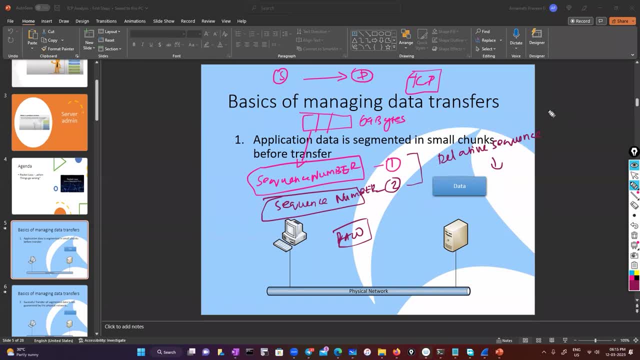 You. you can actually track down that something starts similar to two, double one and it's an increment of one, two, one, three, two and four, two and five, something like that. So it is And sequential approach. it gives more control to track down your packets. 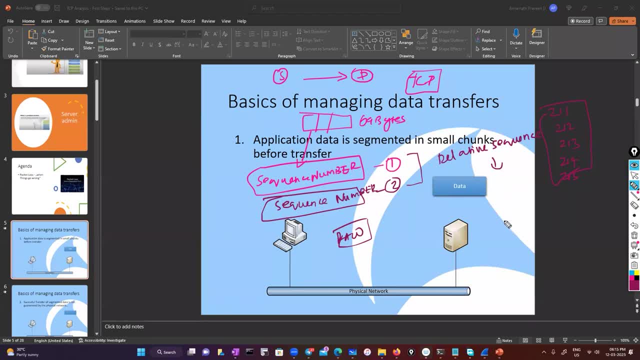 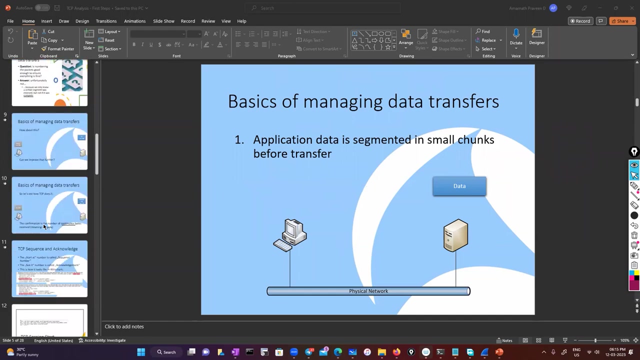 How many packets has been sent and received the raw sequence number. I mean, uh, it's. it's again a very big challenge for us to track the packet. So make to make it simpler and for the- you know, tracking purpose, they have introduced the relative sequence number option in the wireshark where, if you want, you can enable it- and I would hardly, you know, suggest you to always keep it, enabling the 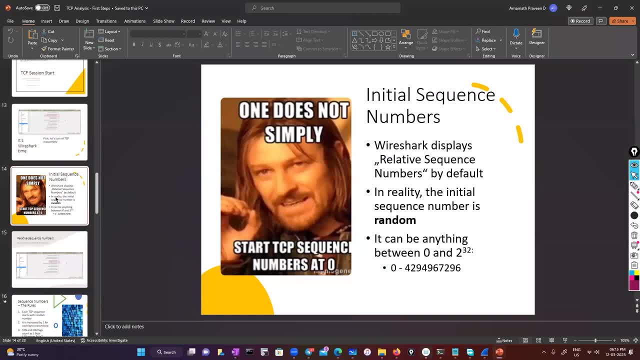 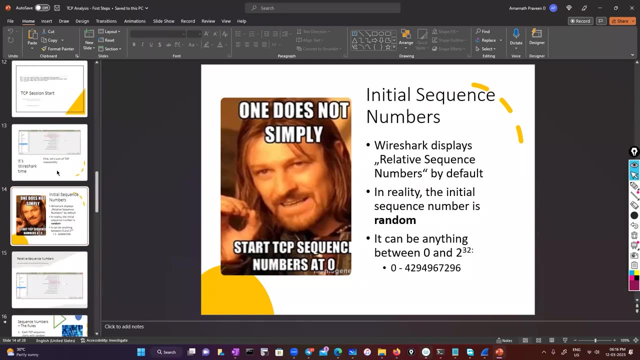 Relative Sequence number. So why shark is place a relative sequence number by default? in reality, the initial sequence number is zero and it can be anything between zero to this many values. It's two to the power of 32.. That is a maximum value that that it can use. 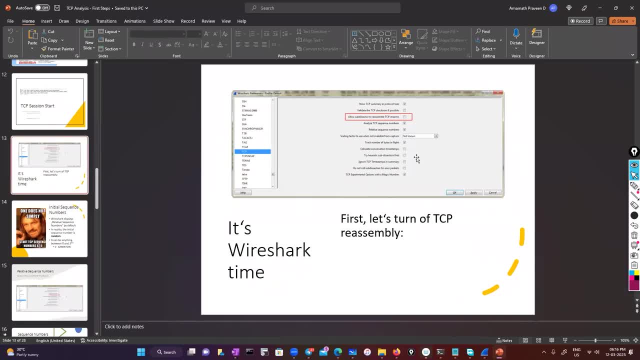 So if you want, you can disable the you know uh sequence number. If you see an option here that is a relative sequence number, that's enabled by default. I I hardly did suggest and everybody, they use this by default. 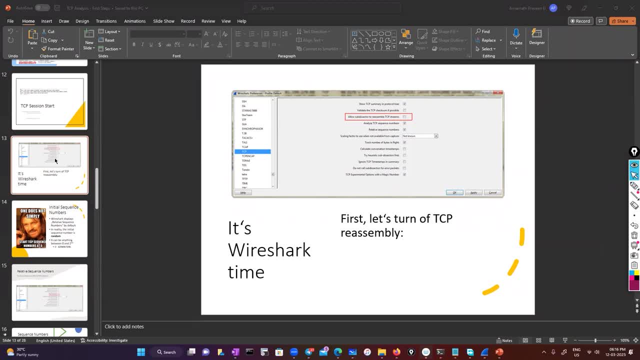 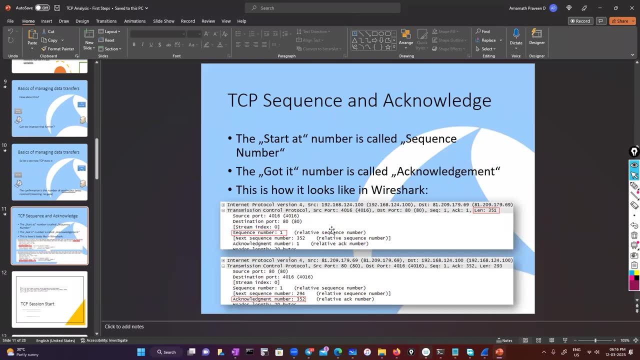 So this is the use of relative sequence number in wireshark. So, coming back to the TCP process, So this is a quick overview about the sequence number and acknowledgement number And when we talk about TCP, TCP is a three-tuple connection. 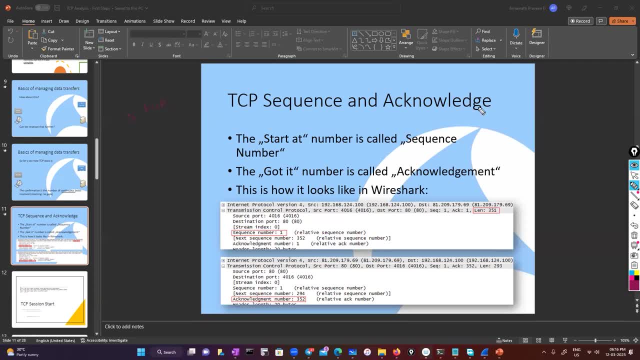 It's a no three. Sorry for that. Let me write a little bigger. here It's: we call this as a three-tuple connection. Why it is called as a three-tuple connection. So to do that, let me open up my whiteboard. 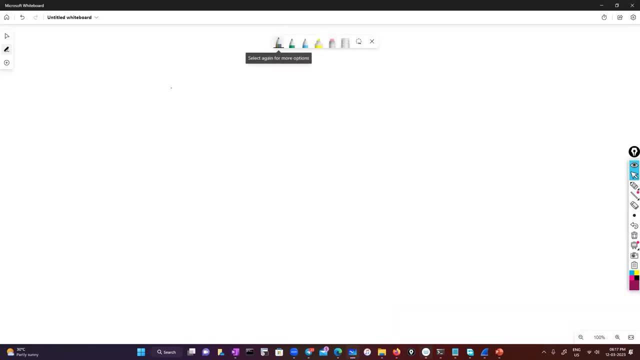 Okay, So if this is example, this is a source and this is third destination. So this is my PC here And this is my server. It can be not my server. It can be a public server And, uh, I'm trying to access a HTTP request time. 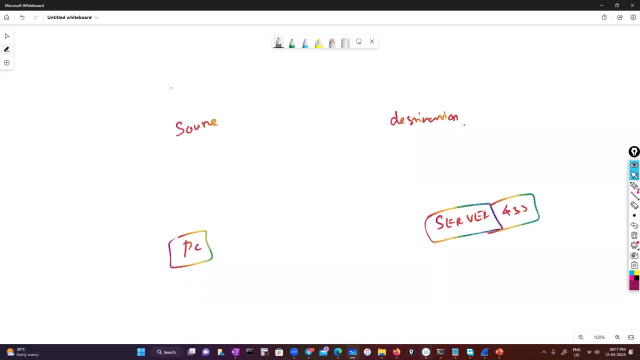 I'm going to generate a HTTP. Okay, So I'm going to generate a HTTP get request here. Uh, I'm, I have opened a web browser here and I'm initiating a HTTP get request. So this party, if you see the OSI reference model, the application layer is a layer where exactly we got our payload, or payload is the application layer. 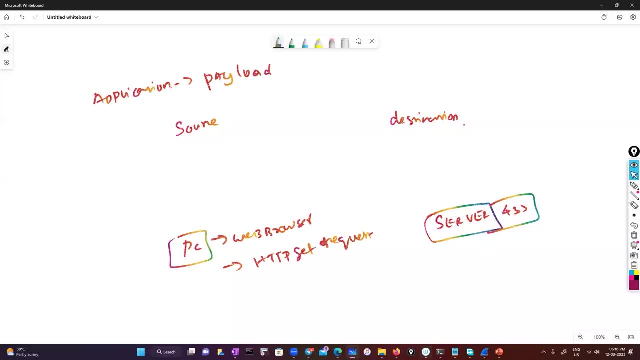 So we'll just look about okay application layer here. So we'll just look about okay application layer here. So how did sequentially happens? Um, so we'll just look about okay application layer here. So I have opened a web browser and here works my layer seven. 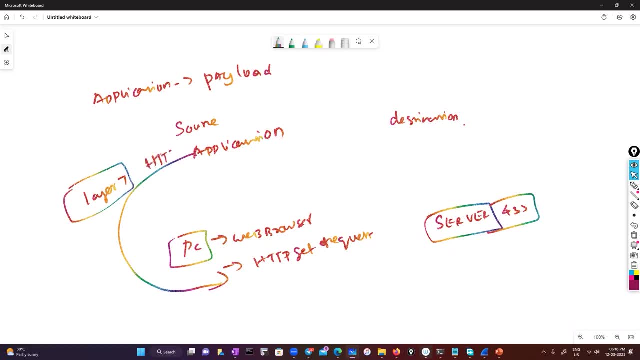 And what is the protocol I'm using here? It is HTTPS. We call this as an HTTPS SS, TCP Over TLS. All the connection was secured. It's all encrypted, So the data is keep on. you know, encrypting for every layer. 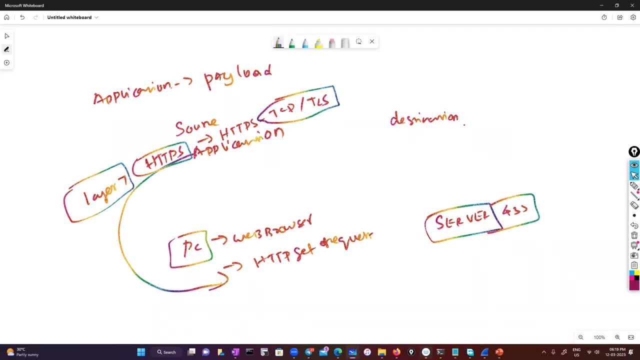 It keeps incrementing the you know, sorry, in every layer it keeps encapsulating the data. So this is presentation layer And you got your session and you got your transport layer And we got the network layer here and we got the data link layer. 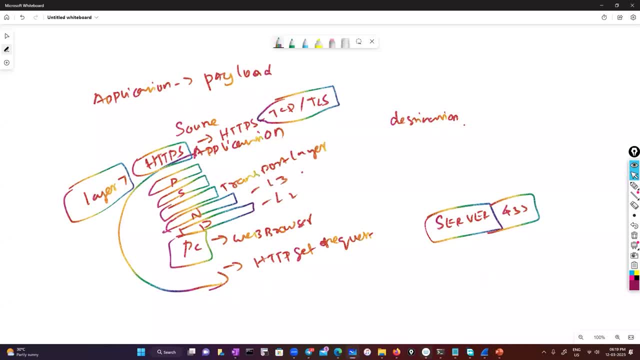 This is layer two. One. this is layer three. So my packet is keep on encapsulating right. So visually how it looks, my packet is something like: see from here: this is layer seven And what is the payload? That is a size TTPs. 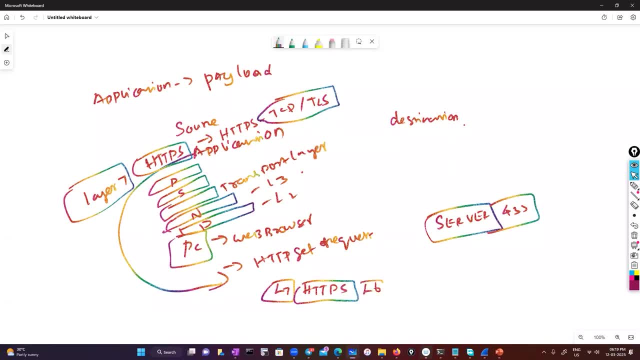 And it will be sent to the layer six, presentation layer. All this data formats will be happening here. And then it comes to transport layer, the key things we are looking here. So inside the transport layer. so it's going to decide I'm going to use TCP or UDP. 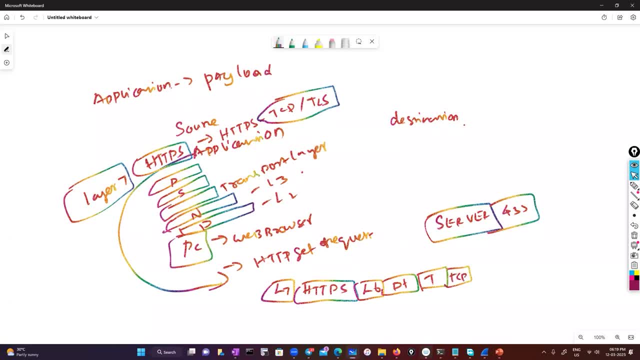 So I'm going to use TCP here. right Inside the TCP you've got multiple flag values. We'll discuss about that, but an overview inside the TCP. Okay, So I'm using TLS. then in the network layer it's going to specify the source, IP and destination. 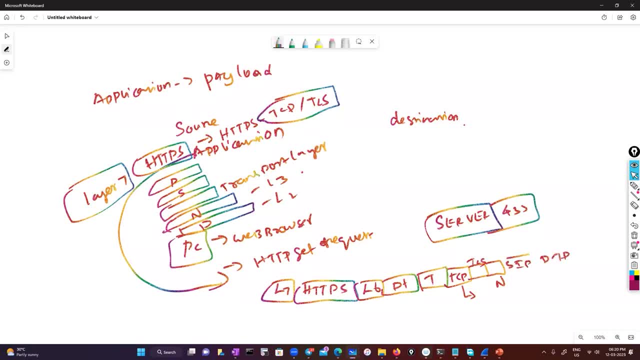 IP Details and finally the layer two. it has source Mac, destination Mac and all this back gets us and is in a one single package And if you look at, if you tear down this TCP packet here, actually your payload will. 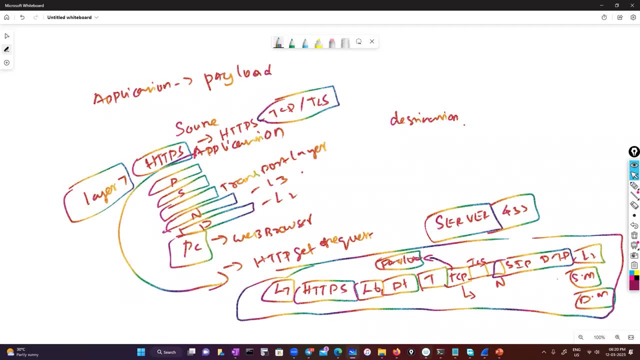 be in in encapsulated right. So my actual payload of this is on the web traffic. This Particular payload, it's keep, you know, upended until it reaches a TCP and from the TCP it will do, it will check. 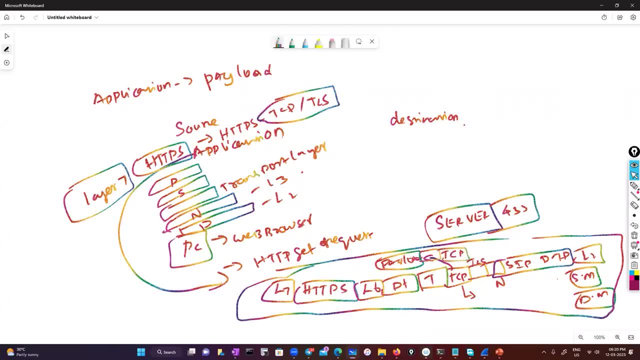 Is it a TCP or UDP? and along with the payload and it will send to the IP layer, then layer two. So this encapsulation keep happening until it reaches a layer two from PC. So all signals it doesn't understand about anything. So whole thing is a pack, is a package. 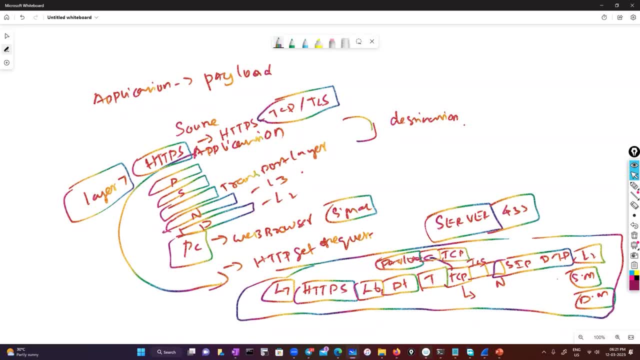 So it's going to push this packet back to the destination And this is a no. So I call this as a top-down approach from the sender and it is a bottom to top approach. So it keep decapsulating, right. So my router is only interested in the IP packets. 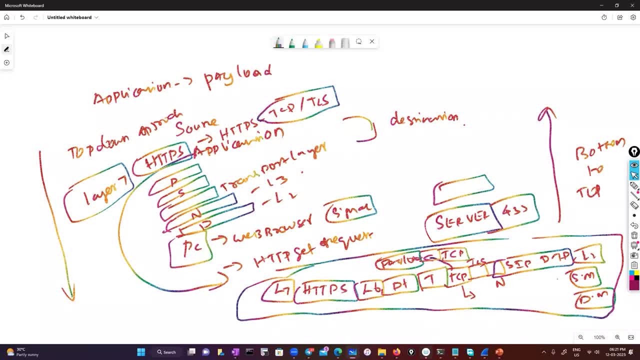 I'm not interested in layer two. So in the same way, switches it will just look for the Mac address and if it needed it will look. It will do all this. you know the router, it will do. Okay, So this particular IP is in my network, but I don't know the Mac address. 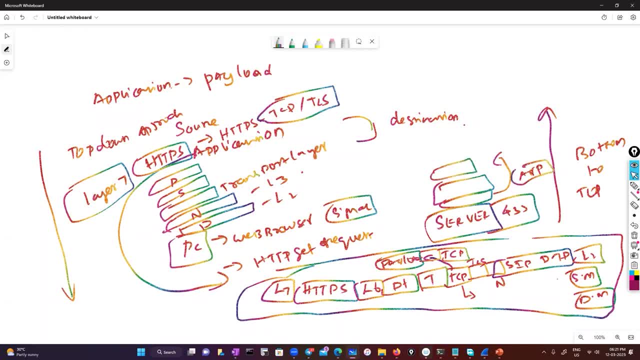 So here comes an R, So this packet is keep on encapsulated until this TCP and it will open up, and it's it. it would see, right, And this is a peer to peer connection, It's an end to end connection. 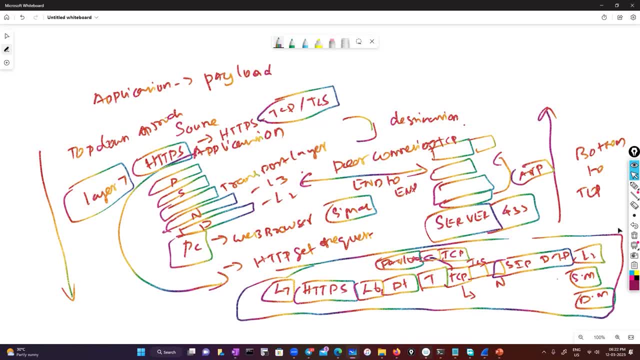 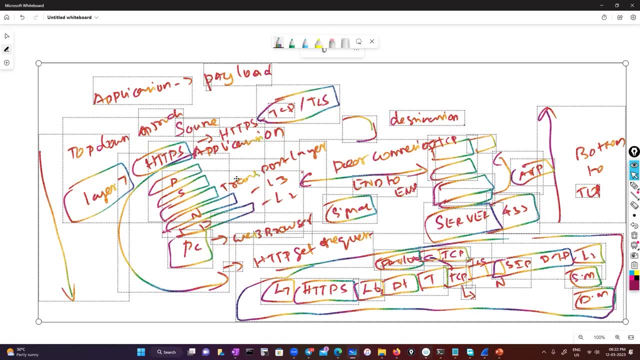 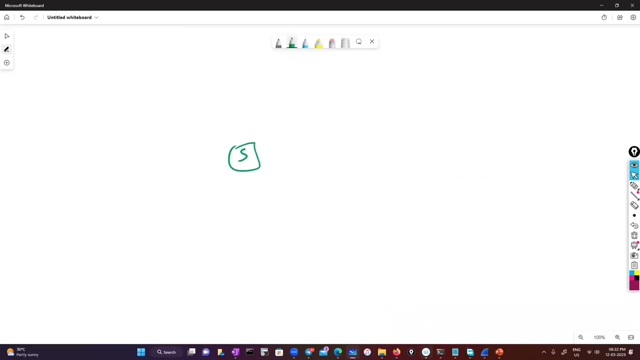 So this is about an overview of how this Packets are encapsulated and decapsulated. When it comes to specific, about TCP connection establishment, it comes to TCP connection establishment. This is my source and this is my destination. So I have encapsulated all the packets now. 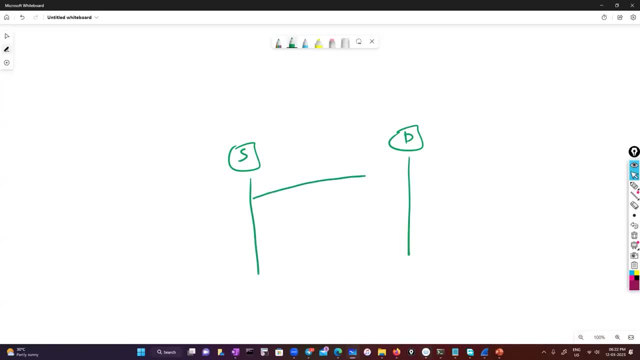 Now what happens? It will send us sin packet. That is something like: Hey, I want to establish a connection with you. Can you respond me back? Okay, But here comes the question. So, inside the TCP sync, what are the information it would send? 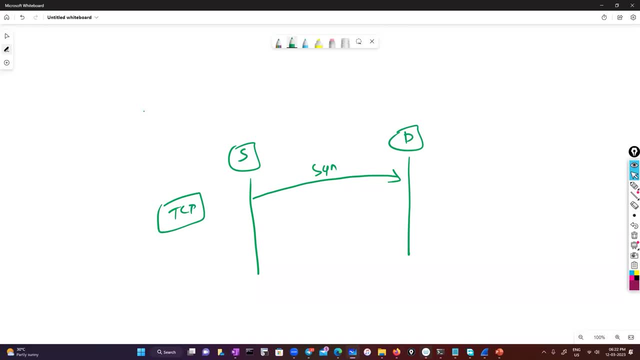 That is important, right? Okay, Let's see. Now this is. I said this is a three tuple connection and I have sent a sin. for this sin It's going to see sin act. for your sin I'm- I'm acknowledged. 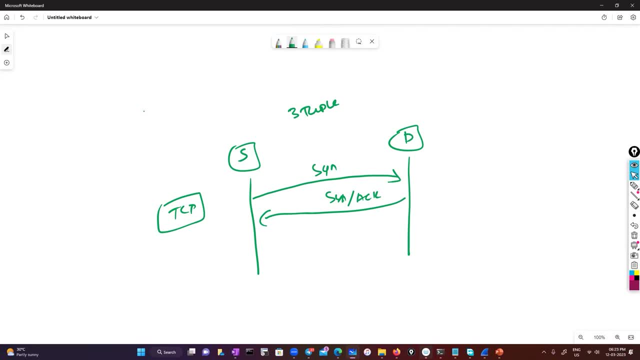 I'm okay to establish a connection now for your sin. I sent and sin act, So that's kind of an agreement. Okay, I am also okay to receive your traffic So far For this sin act. it's going to send an act and here the connection established until. 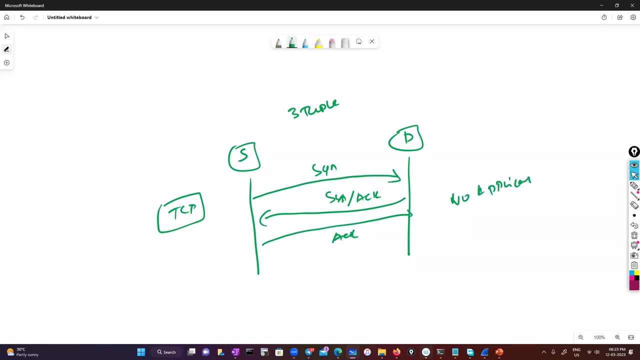 this point: no application data, no payload. So here we say: it is in a ghost bites The sequence number, something like it. it is just for identity purpose. It just marks it as a. my sequence number is one And I'm sending this to you. 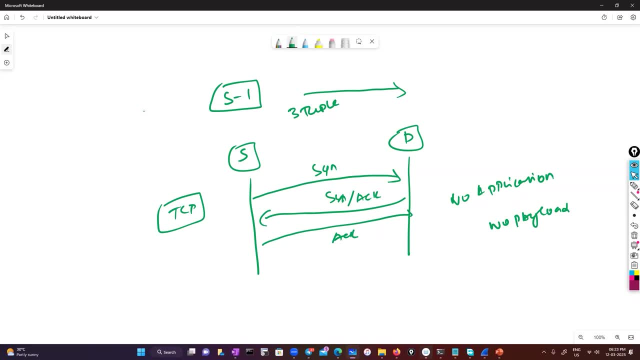 If you got my sin packet, you have to, you know, update, Okay, You know- acknowledge this back. So it's going to say: okay, I received your packet, So I'm going to acknowledge, and my acknowledge bit does set. 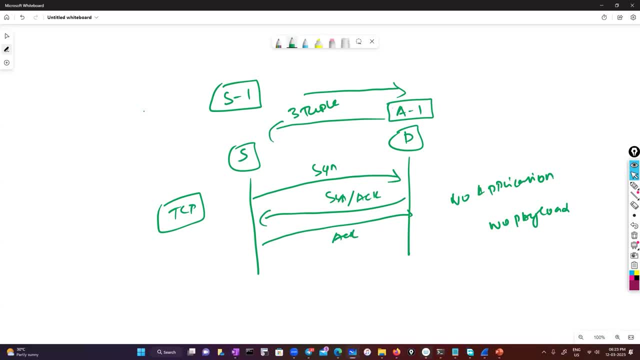 And it's going to send this back. So inside this TCP, if we peel out the TCP packets and parameters so you can see what is sin flag, If it is a sin flag set, then it is a sin packet. If it is a reset packet, so it is a reset set. 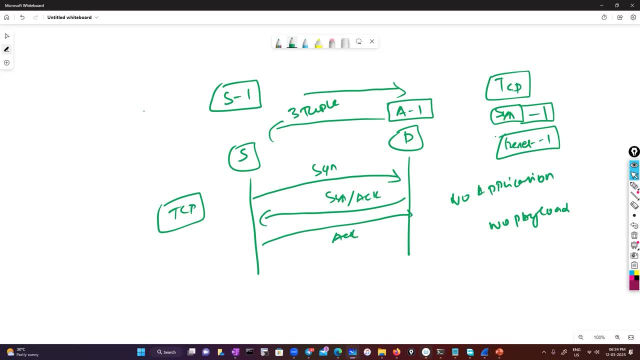 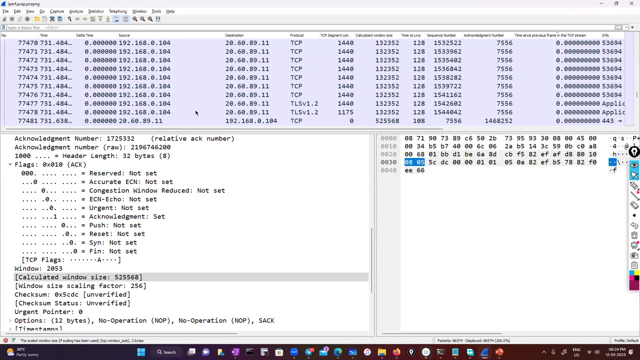 So reset happened here. So this is how the connection establishment happens. Then comes your actual payload. So now let's see how we can see all this information with a complete visual in Vireshark. So to do that, let me open up this capture. 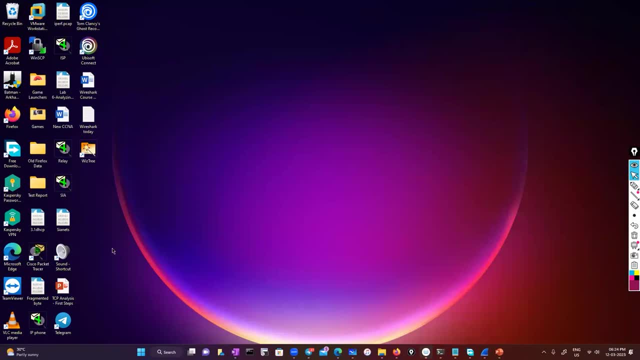 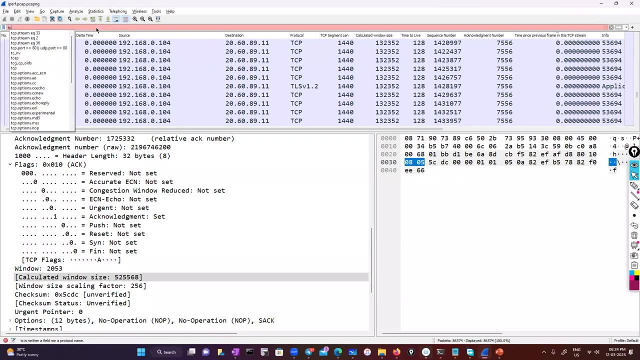 Let me go to TCP capture. Okay, Okay, Okay, Okay, Let me take this IP of capture. So let me give TCP. So this is the filter we use in the Vireshark. So let me give you a glimpse about the options. 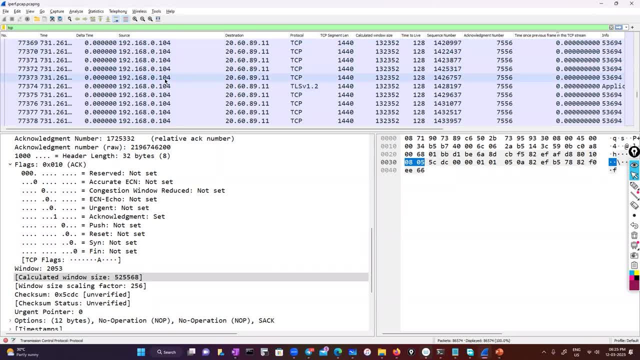 What tells we have solved the customized template, what I have created to have more insights on the fly. Okay, Okay, Okay. So this is the time when exactly the connection happened. This is the column where it defines about the time here. 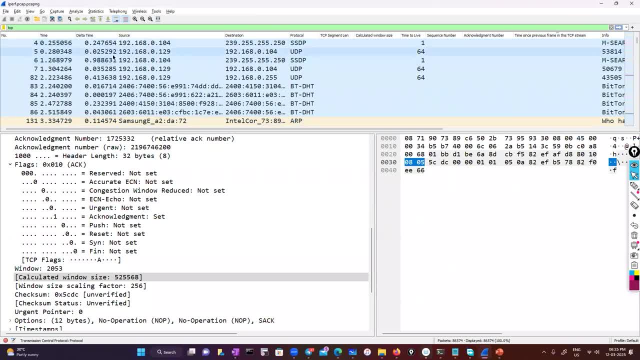 And this Delta time we'll discuss in the class, but for the reference, Delta time is very vital to understand where the problem is. So it's all mostly in milliseconds, but if it crosses the seconds, if you actually see this all milliseconds, this is 35 milliseconds and this is 41 milliseconds and if you see 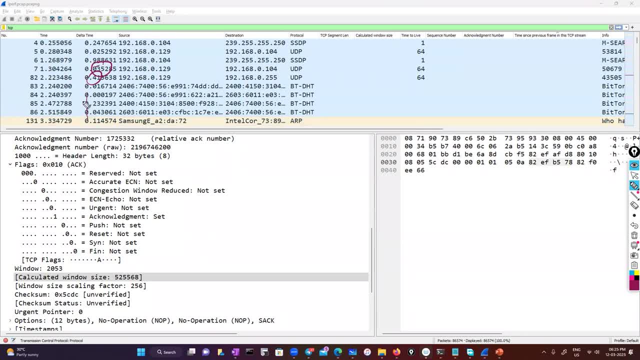 any values that's been incrementing here. here that that is defined as seconds. so in the networking world everything is happening in milliseconds. if it exceeds the milliseconds and if it's going beyond millisecond, if it isn't seconds, then there is a problem. that's a slow connection. so networking never like the packets to be in. 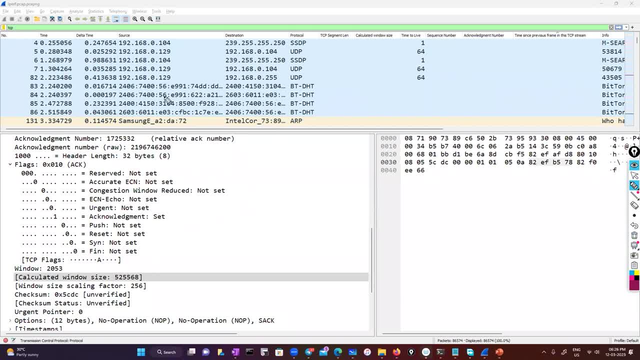 seconds always. so for the optimal performance you always, it has to be in the limitation of milliseconds. so that's how this delta time value is used to. you know, figure out what is the time taken for the source and destination. so delta time, and one key thing i would say is we call this as an 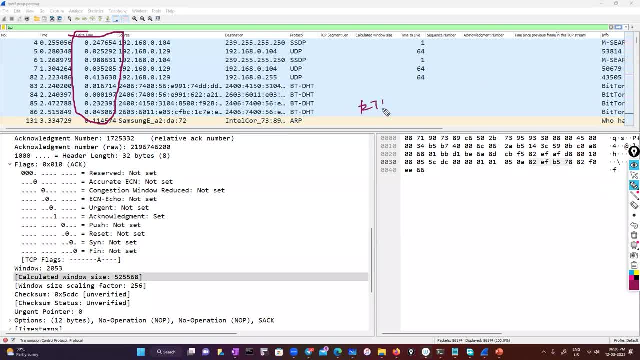 around trip time. call this as rtt example. if you make a flight booking, that's something it will ask for. it's an one-way booking or it's a round trip booking. so that is something from source to destination, from destination to source to destination. so that's how this delta time value is used. 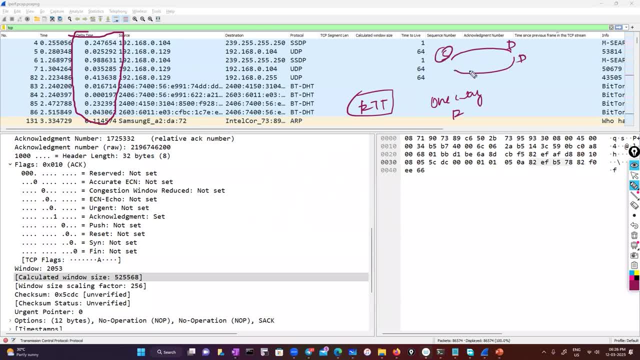 source. what is the time taken? that is bi-directional, from source to destination, from destination to source. how long it took? so that is actually a round trip time. we call this as an rtt, even if in the ping request you you would see your rtt time when you do a ping generally you can see. 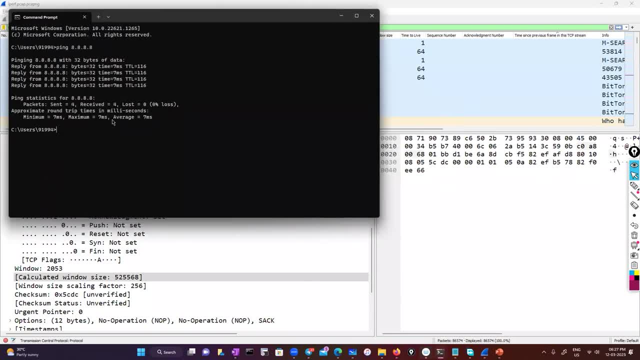 your rtt. what is the average time taken is seven milliseconds. that is your rtt, your rtt time, that is your rtt time. that is your rtt time. that is your rtt time. average time taken is seven milliseconds from source to destination. back from this destination. 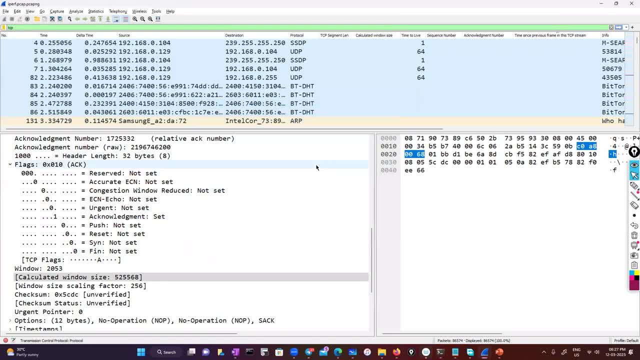 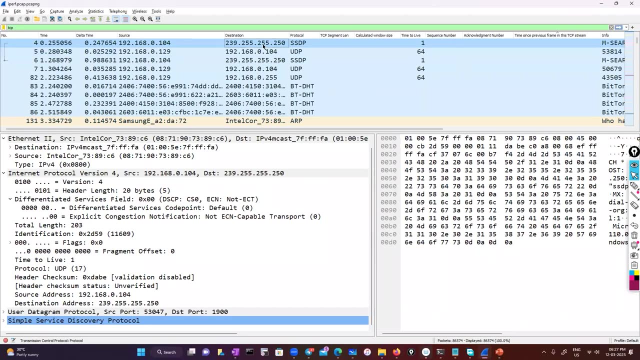 to source, that is, your rtt, and then the this particular field is talking about this as a layer three, and you see all your ip packets here. so what is my source and what is my destination? this is the destination network where i'm trying to establish a connection, and this particular 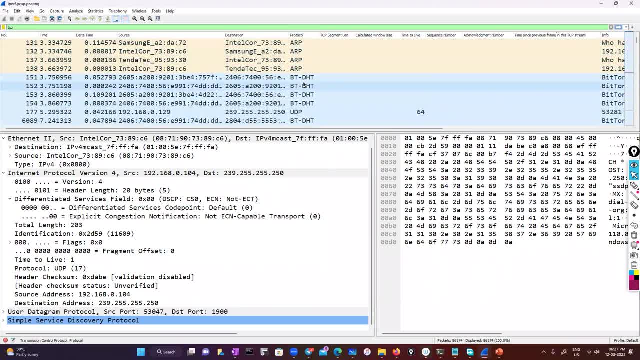 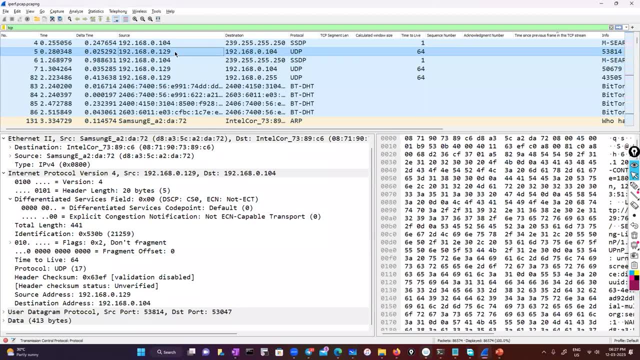 column will give an- you know- a complete insight about what particular column is going to be. particular protocol is used by the source and destination. if you see, here it's my udp. it can be a dns or it can be a video streaming. that's how we can classify the packet. so here. 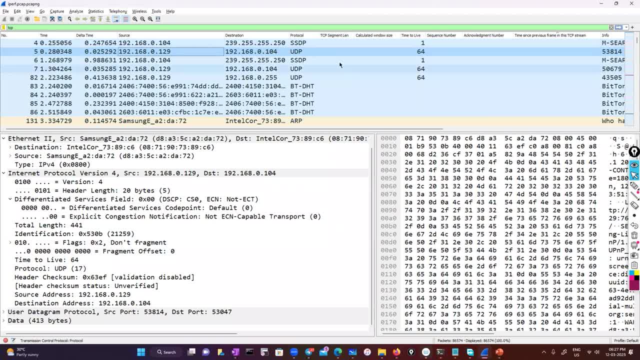 it says it's an udp and tcp segment length. we'll talk about that when we know right when. when we talk about this osa model, we generally we know about this all in the network layer. we say it's packets, all it is ip packets, it's network layer. so from the layer 2 perspective it's all frames. 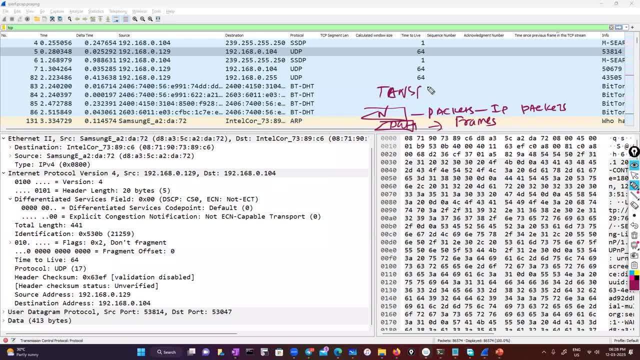 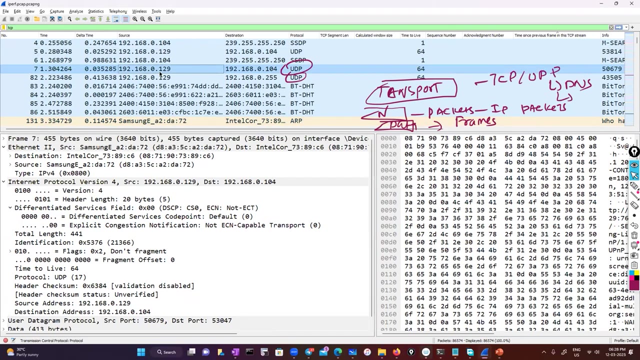 and from the transport layer. i'm going to send a packet using tcp or udp, so it's all udp packets, right, so that defines it can be my dns, it can be my video streaming, so we have to check how, how you will going to classify it using the port number if you just click on this particular packet and 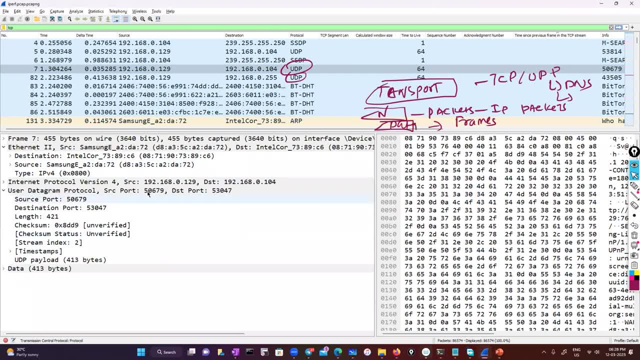 you will drill down, you will see. okay, this is using udp and this is a destination. port is 53047. so this is not my dns packet, this is something else. so here is your actual payload. payload is something your real data, right? so this is your actual payload and this is your real data, right? so 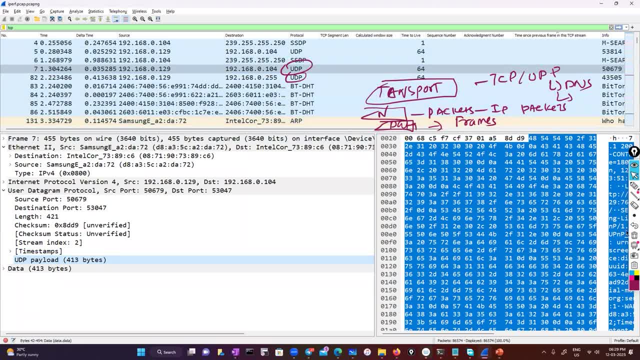 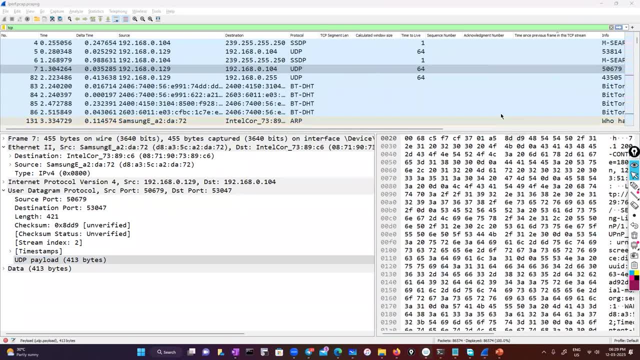 you. you will get about the insight about everything here. this is about what protocol i'm using. it will give you that and tcp segment length. so, uh, we know, in network layer we say packets. in layer 2 we say frames. in the transport layer we call this as a segment. example, if i have a 1gb file, 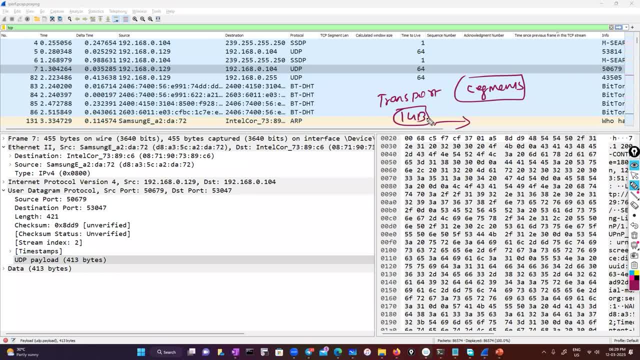 so can i send this a one single file? definitely not. so this 1gb file is again chunked into multiple segments, so we call this as one segment. so for my one segment, how much maximum data i will send? that is your tcp segment length. what is the size of my segment? 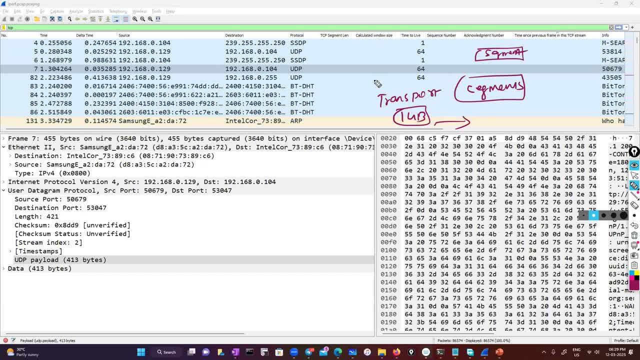 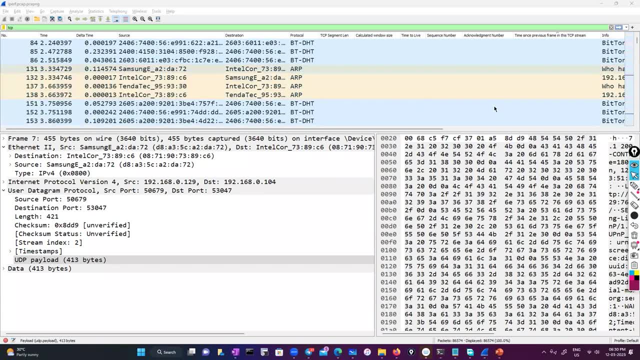 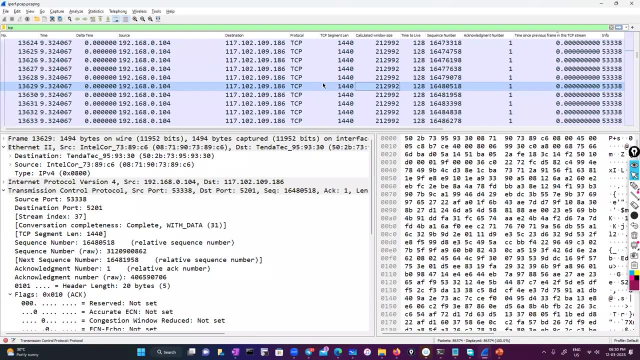 so, and one more thing here: the calculated window size. what is the window size? that is something like a proposal. so i am proposing you example, if i come down, drill down a little bit down, if i see my calculated window size, and this is very important. the maximum tcp. what is this tcp maximum? 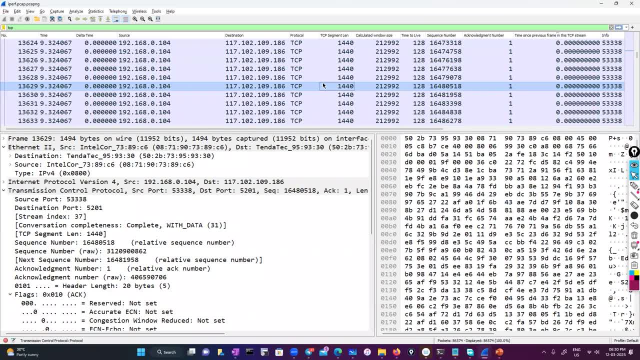 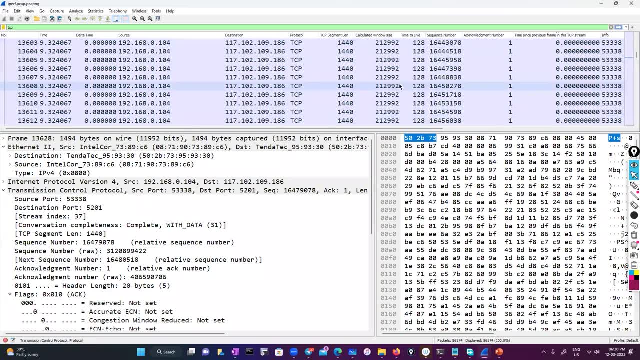 segment length. it can be 14 440.. and what is the calculated window size? so this is something the proposal it's saying that your window size never starts like this in the beginning. if you see the capture in the beginning, if you see the, this window sizes keep increasing. so when we establish 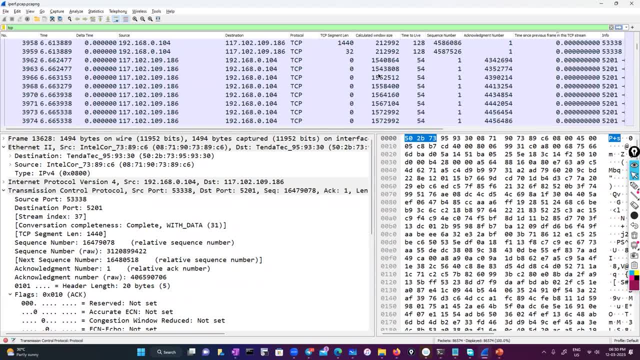 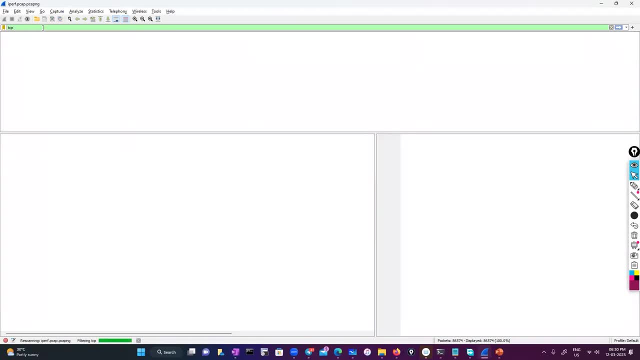 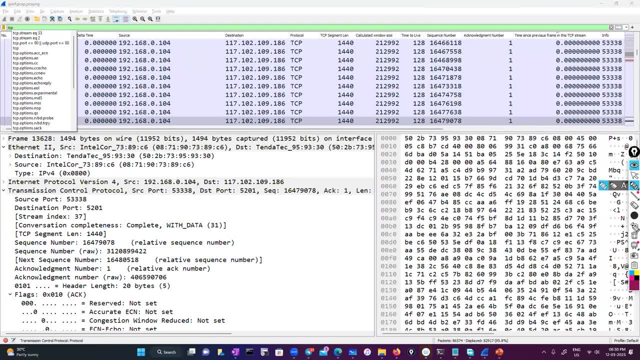 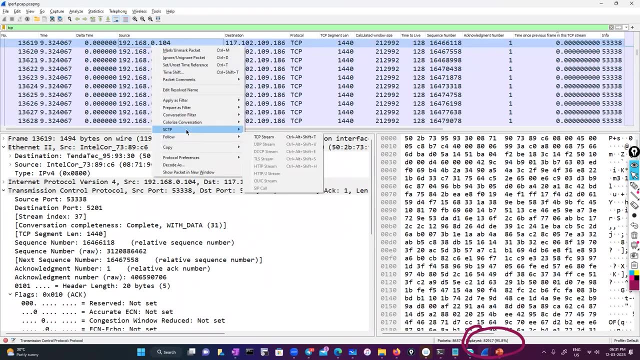 this is all my tcp packet here. sorry for that. so this is the number of tcp packets alone. i have to take the tcp packet and here i'm going to take this and i'm going to conversation filter and i'm going to tcp. so i have to do a right click on this and i'm going to. 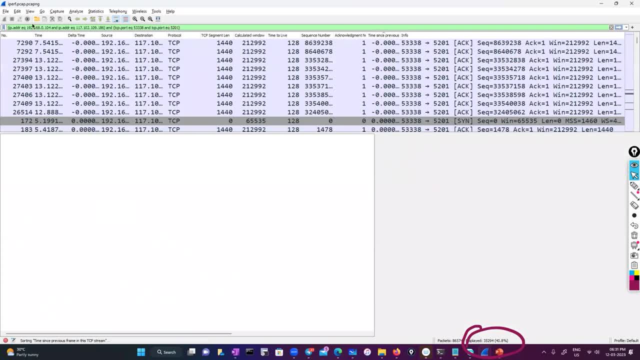 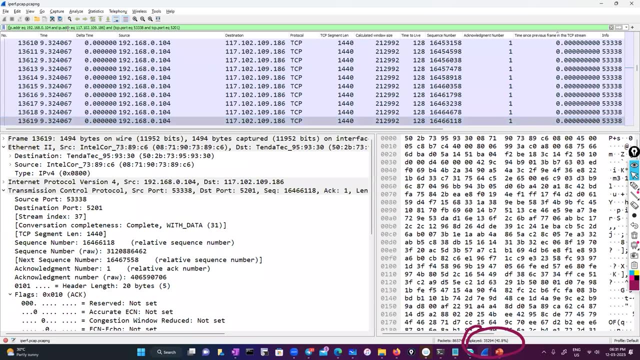 conversation filter and i'm going to give tcp so it's. it has populated a default filter value here with this. so we got what? all the information it says. this ip dot address equal 192, 168.0.104- that is my pc- is 117.102.109.18. this is the public ip address, 186, and this is the port number used. 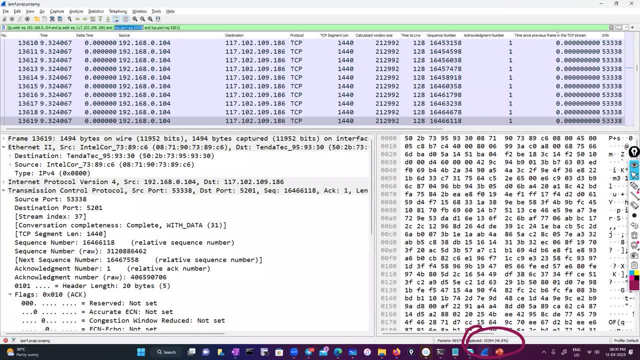 what is my source port number? it's 53333, so that is a randomly generated port number. this is generated by the operating system from our pc and this is a server port 5201. so what is this particular capture? this particular capture is something i have to. 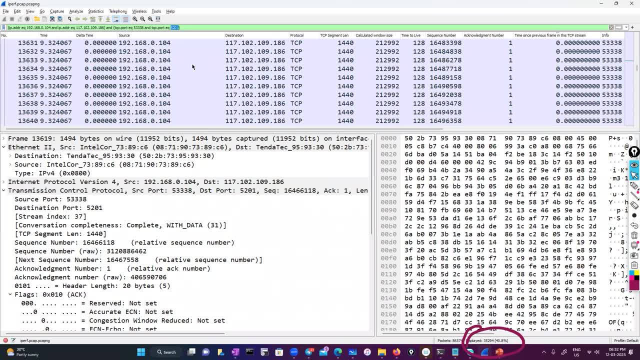 capture this. when there was a throughput issue, i had some problem, my pc had some problem with the throughput. so let's see how this window size exactly helps us to figure out that problem. yeah, let's see that. so before that. so i want to go from to the beginning, right? 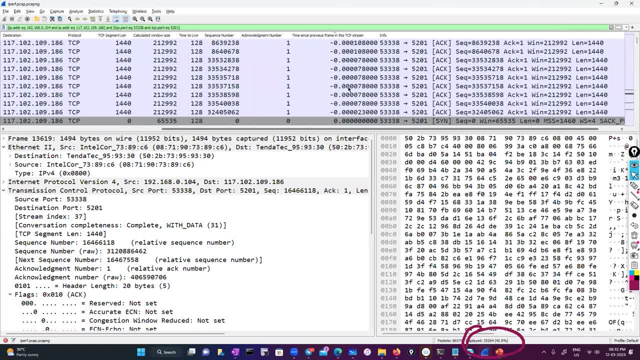 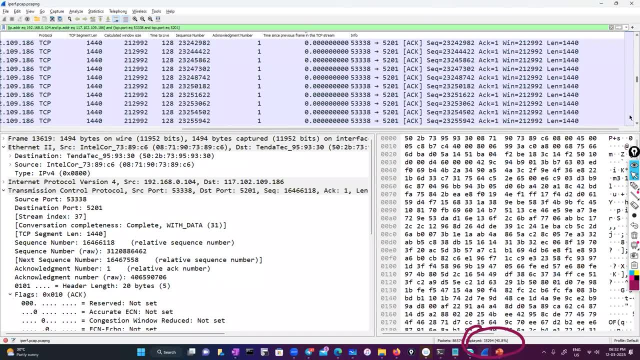 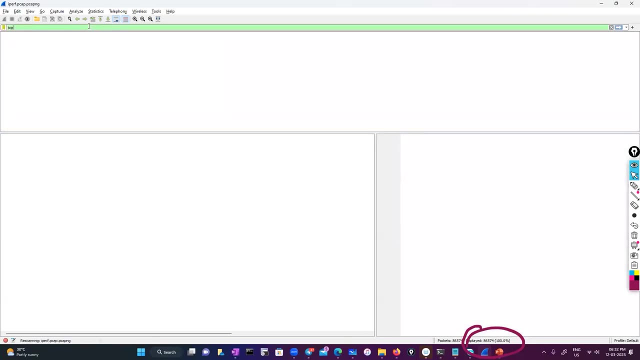 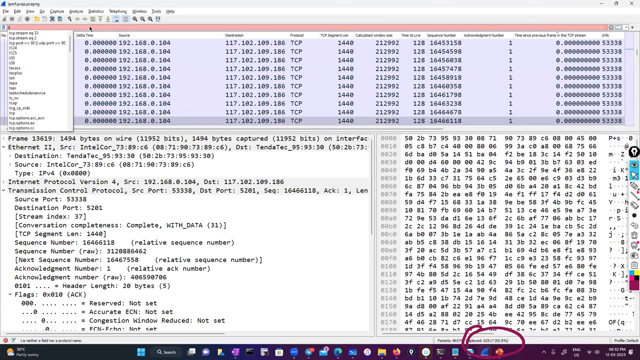 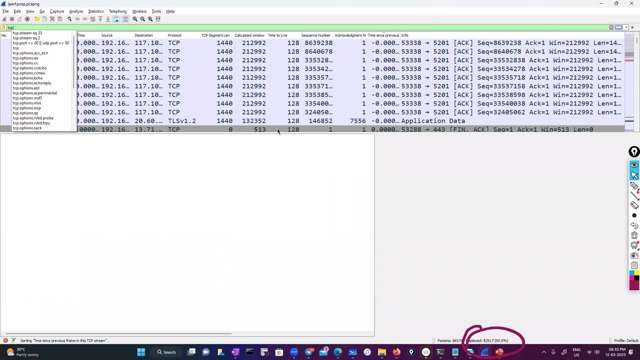 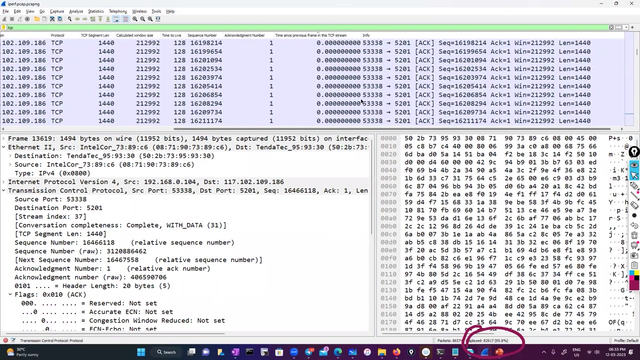 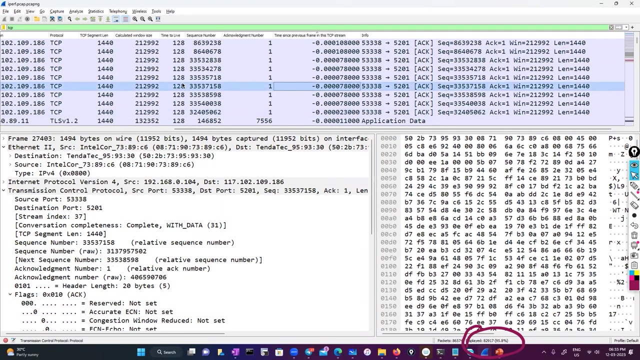 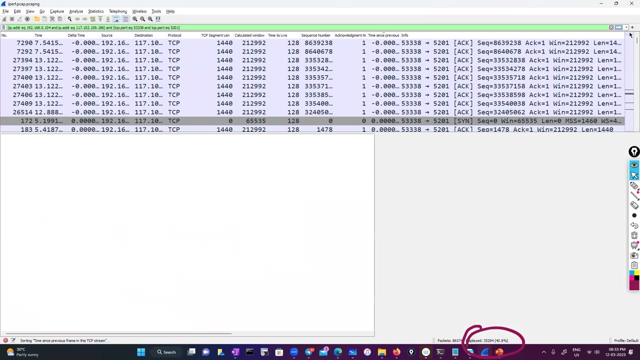 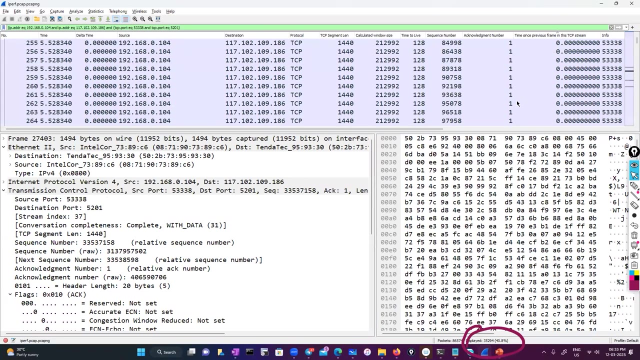 so where exactly my synchronization happened here? let me little bit drill down this. this is actually the finished packet. i don't actually see this tcp flow. it takes some time. that's how the tcp is. okay, this is the information i can see here. let me see conversation filter: tcp. 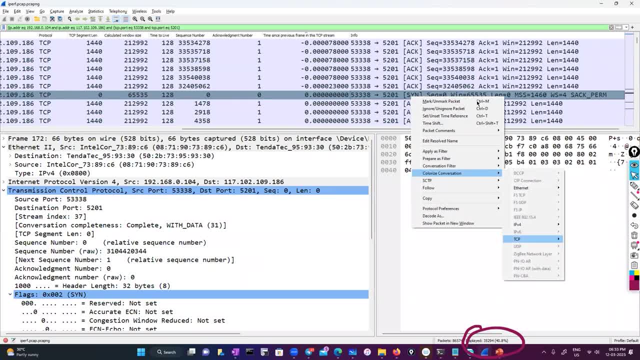 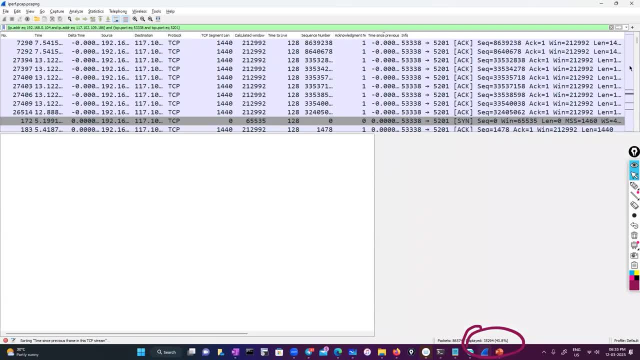 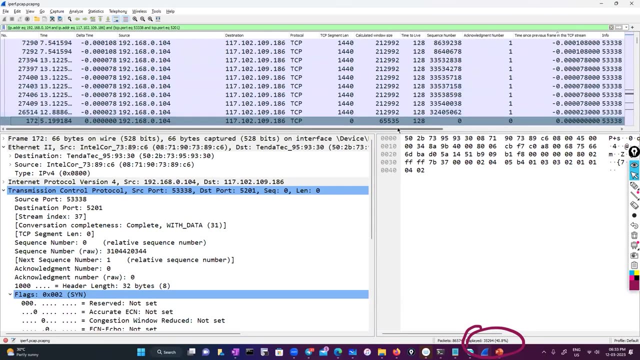 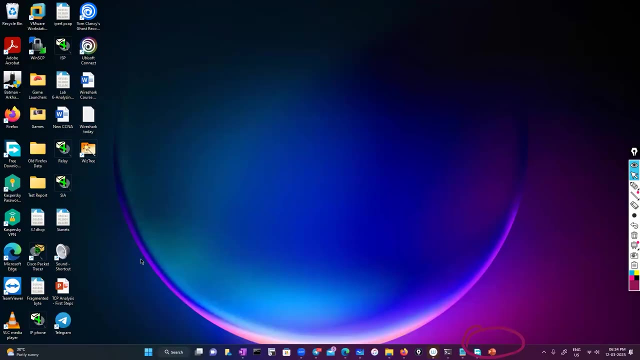 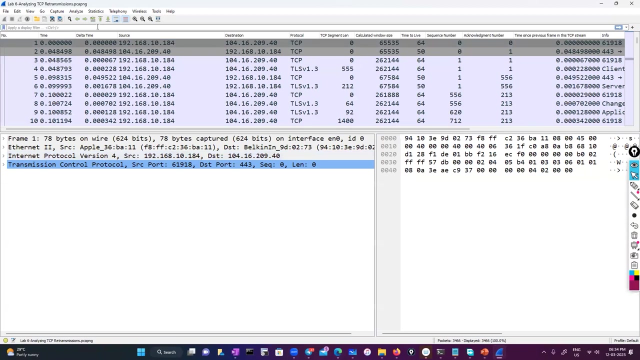 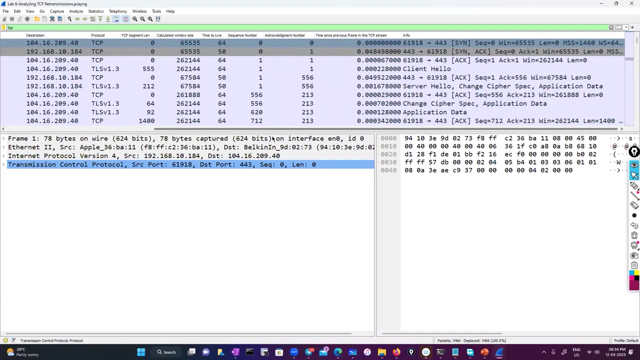 it's a pretty big packet. i couldn't actually figure out. let me take a different capture. i want to see the syn packet. oh, i got stuck here. okay, let me give tcp here, okay, so here we go. so we got, you know, sin senai, senai. 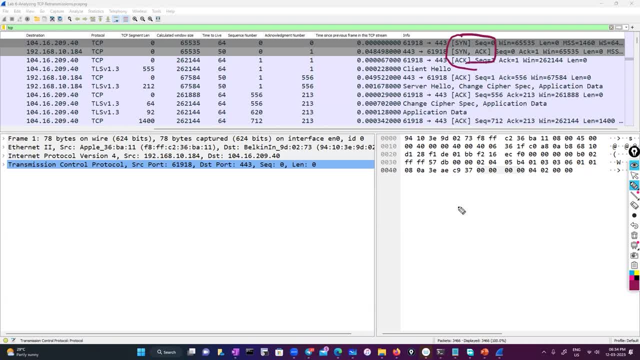 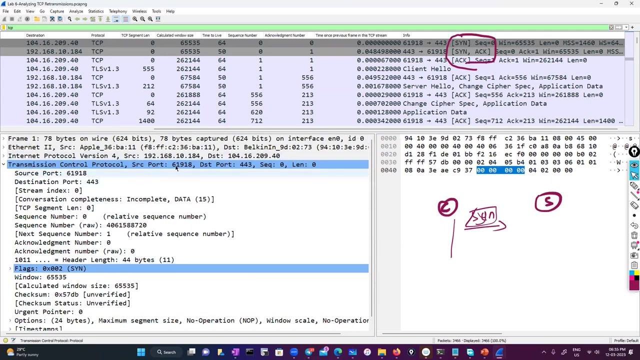 can act. it's talking about this three tuple connection, right? so this is from a client, there's a server and it sends a sin, the beginning before establishing a connection. so let's see. so if i take this particular packet here, if i open up my tcp, it's transmission control protocol. it says my source port number. 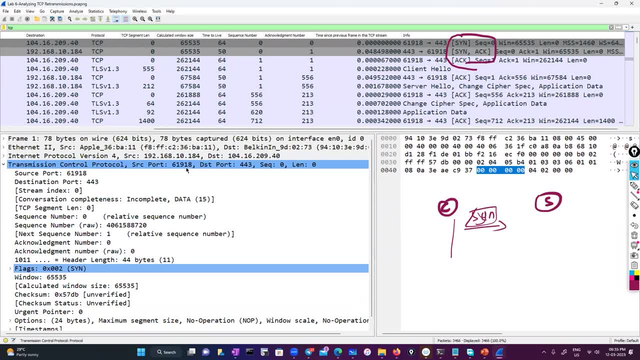 is 61918. that's my source, port number source and this is a destination port. so from 443 i can figure out this is https. so now i i come to know. okay, this is my source and this is my destination. and if i look at this- uh, ip protocol, i know this is my pc and destination is a public server. 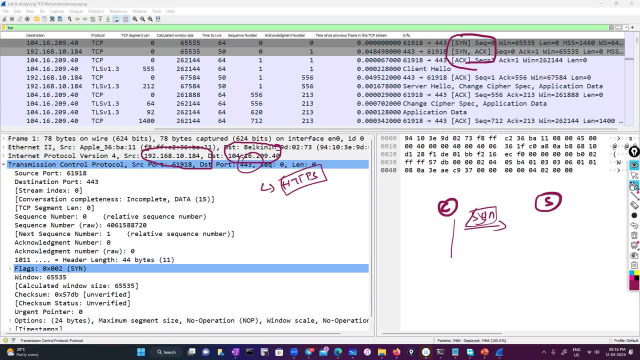 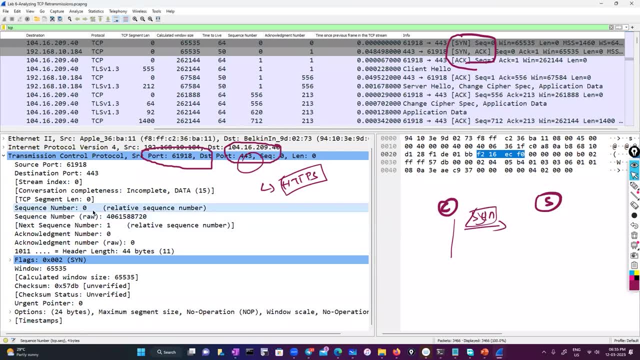 and, if you see this, this are the key things we should know about. you know tcp, so i was talking about this sequence number, since i i i'm not sending any kind of data at this point, so this is my first packet i'm going to send to this destination server. so this is the relative. 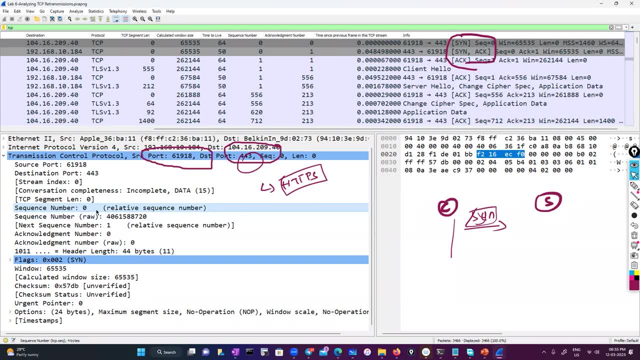 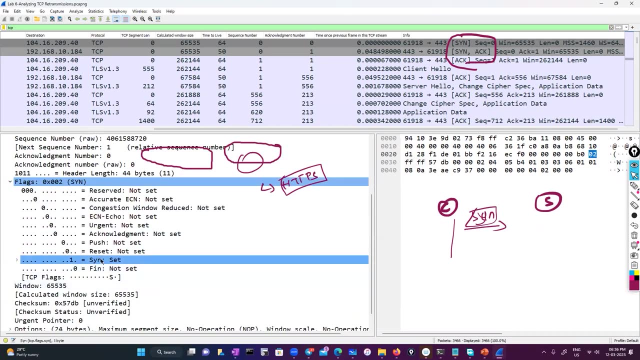 sequence number used by y shark. so this is the only value we are going to see. we are not going to see the you know random sequence number here. so we are going to see this sequence number and if you see the flags, this is what i'm talking about. so it says it's sync flag, right? so 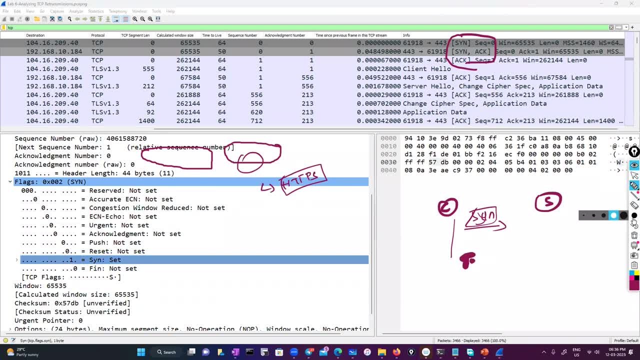 this is a sync packet and this particular flag it says it is sync flag. this is my sync packet. so from the server, what is the response we get from the server? if you see here i i made a filter for you know, granular control. there i can see all the information right away here. 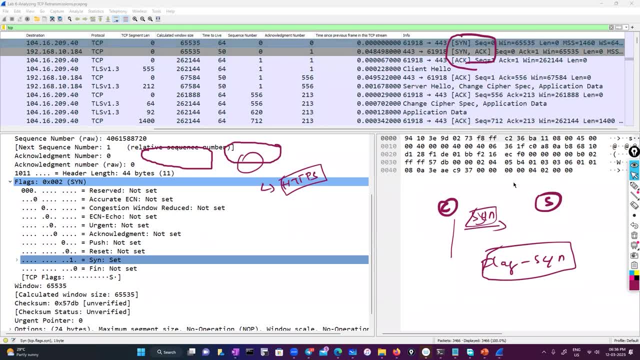 so here, if you see, the ttl is very important. uh, the three default ttl values are 64, 128 and 255. and here my pc is. it's using something: 64, that is the default ttl value. so i'm going to assign this solution to you. so, for example, if i say ttl is for every hop, that is something ttl is. 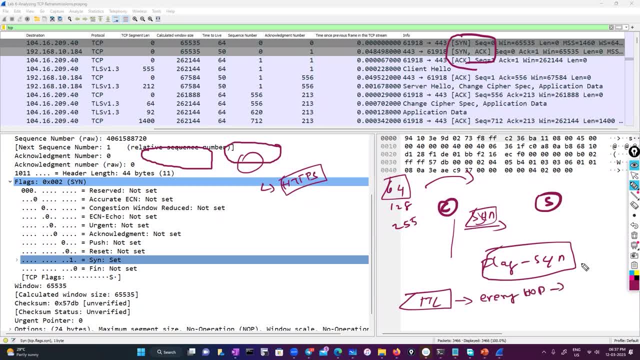 for every hop, your ttl will be decremented. right, ttl is something. for every hop the value will be decremented. so, example: this is three routers. so i know my internet connection. it has, you know, many bgp peering. that happened in the middle that we call as internet cloud. 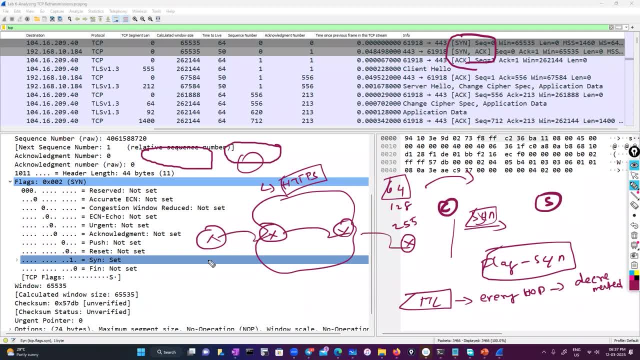 and i got my destination somewhere here. so it's all connected. and for every hop, for every hop, the ttl will be decremented by one. that's the logic. so here, if you see, i can definitely see the packets are routed and my routing is fine. so the sequence number is zero and you know for this, the acknowledge number what 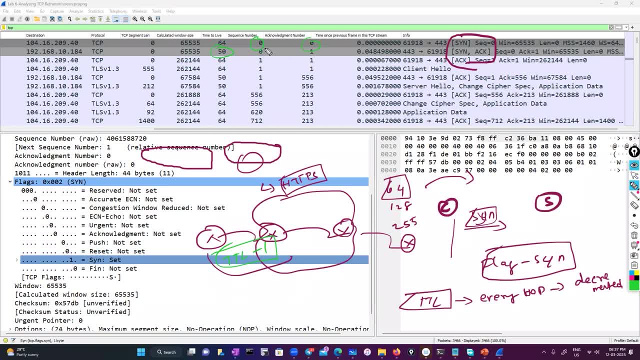 i get from the server is also zero. so what is the acknowledgement number actually? it looks like. so that's your actual data plus one that's your- you know- acknowledgement number, always. so if you see here, the server responded back with a synac and for the synac my pc has been send a send request. 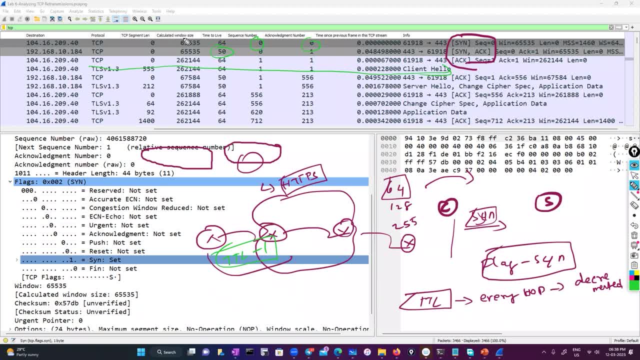 back and if you see the calculated windows, i see it started with the very least value, right, the default value 65500, 535, and that's been increased now. so i am proposing for 65535 bytes. but now, since i established a connection, here we go. you send your real data, your payload here, exactly your payload. 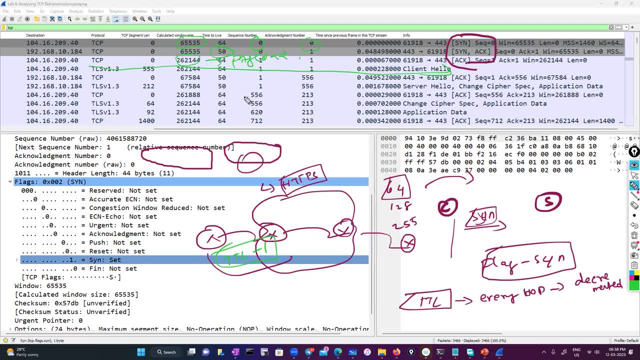 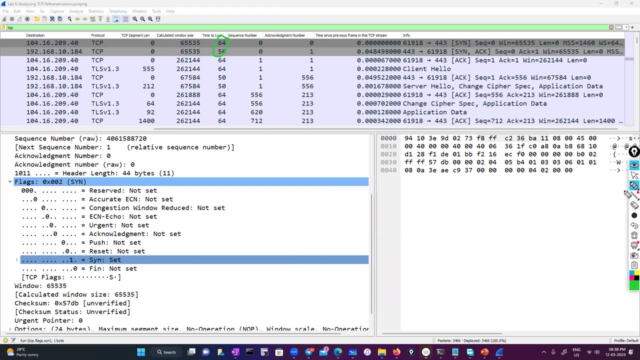 happens and why this is important, that that's a question here, why i should know about all this. definitely because if there is a routing problem i can figure out from the ttl. i can figure out: okay, this is a problem with routing string. right away i am going to stop this. and if i see down, i mean if i drill down, if my ttl is not, 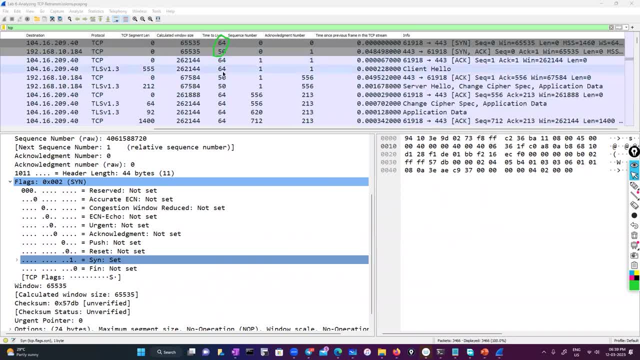 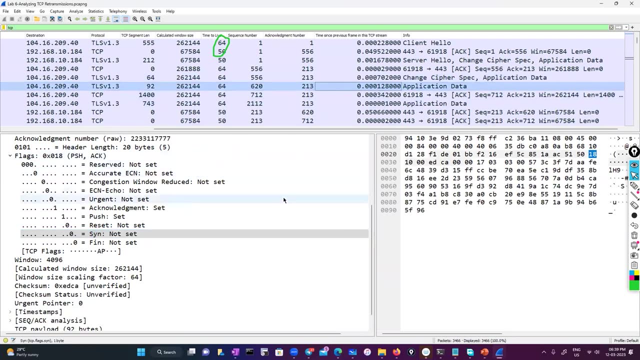 decrementing, there is something problem with routing. so now i conclude: okay, this is not a problem with routing, this is something else. right, if you come down the same way, the ttl is keep decrementing. if you see, here is your application data, exactly your application data, you know, is. 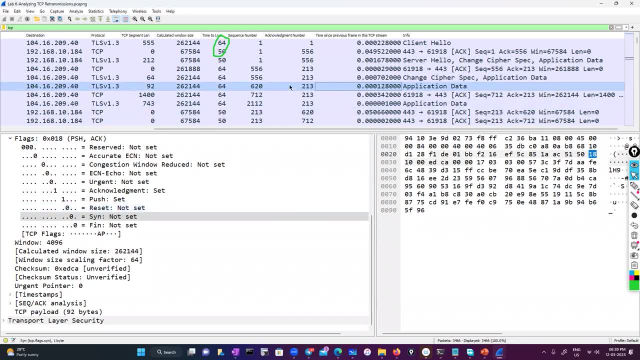 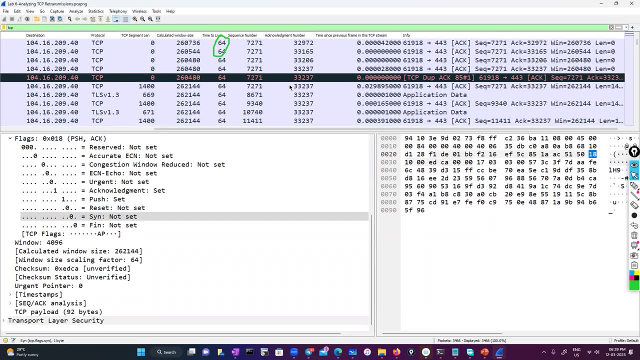 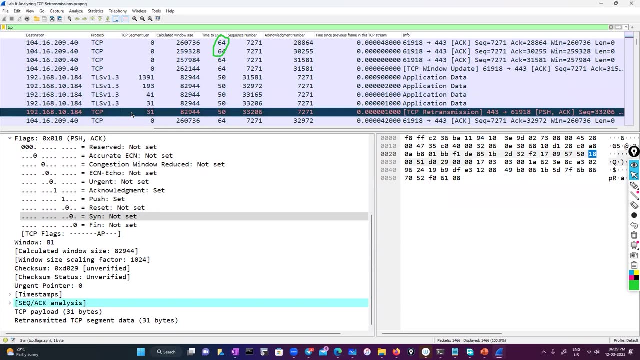 being transferred here. your real data is transferred here. you know, you can see if it can be over three accesses. if you keep drilling down here, your application data exchanges keep happening here. so when i stop here, exactly okay, i come to know. okay, this is a tcp retransmission and this packet 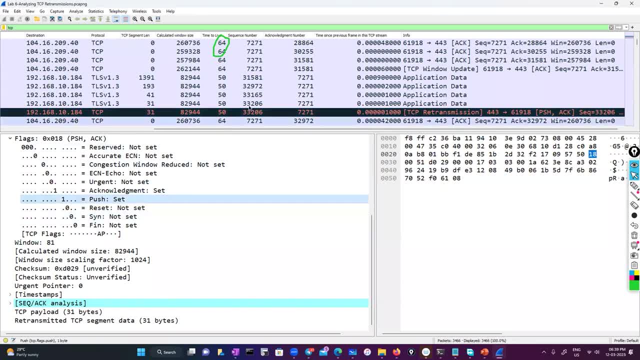 is push packet, how i know about push packet. so if you see the flag here for this particular packet, the push packet is set. okay, i'll discuss about this. so the flags are very important and mostly in my mind as well. so I've drawer products, but also Active admins, gear, devices, etc. 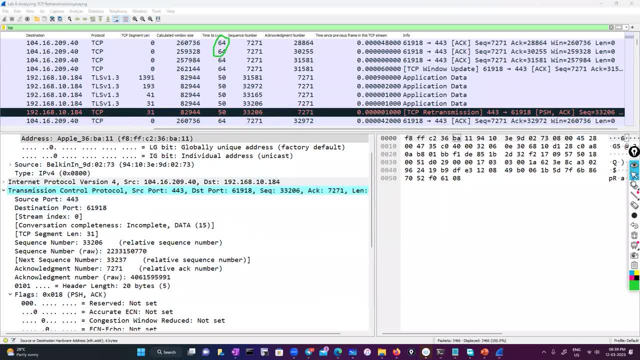 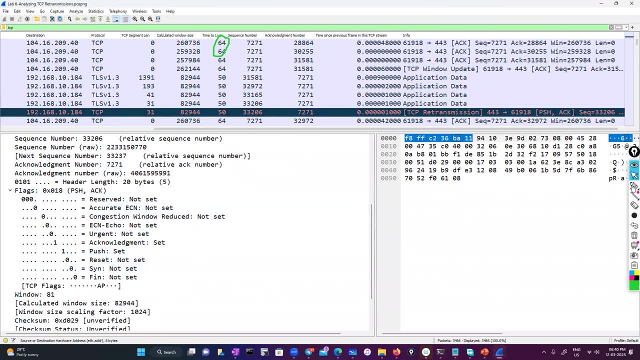 in my experience, and you know, always these three parameters are widely used in most of the time the tcp flags- one is the key thing- is the sin packet, sin flag and then push acknowledgement fin. believe me, these four are the, you know, key flags that most commonly used. 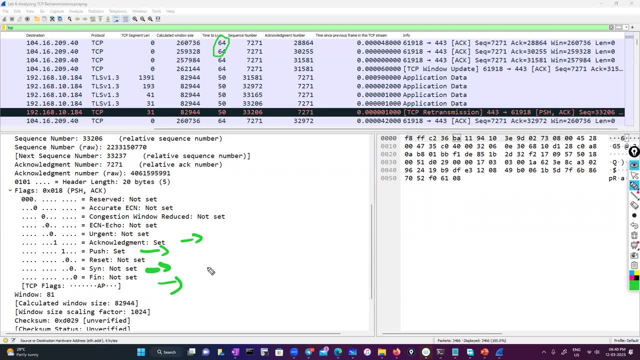 and we are so much interested to know about only these four most of the time, i would say so it will not go beyond that. so push is something here. i would say push is something. see, it generally happens when the you know connection is about to close the data transfer. 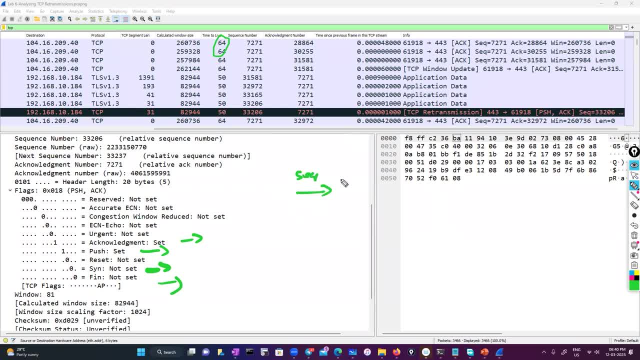 so, example: if you send a sequence number and if you send a sin and you get a synac back from the server for that, i'll send this acknowledgement again. so here your actual data transfer is going to be the same as the actual data transfer. so if you send a sin and you get a, 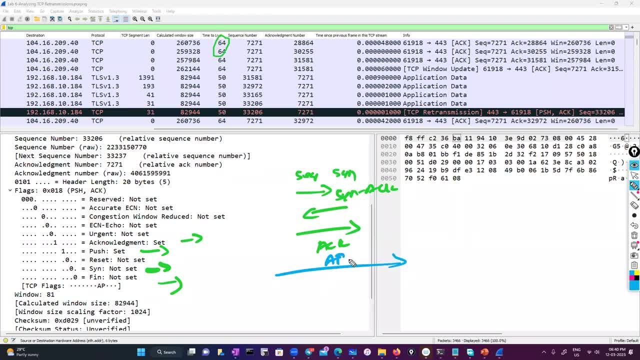 is happening right here, your application data happening and for every single conversation i got an- you know, unique sequence number. and this particular application data transfer is happening between source and destination and when it is about to send this, set this fin flag. it's about the push. hey, you don't worry about that, you keep receiving my data. we are going to finish this. 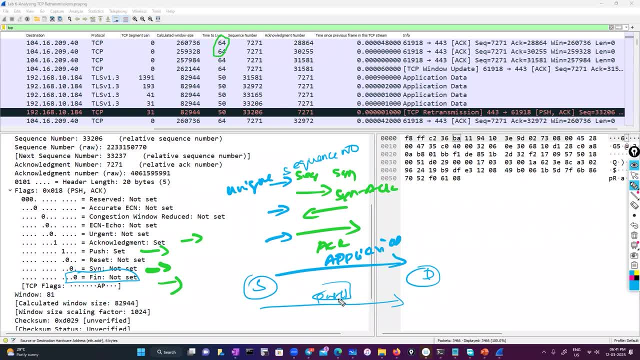 traffic. i mean, we are about to end this conversation. this is, i mean, a couple of bytes that's left out from me. so i'm going to push this packet you're going to receive, and exactly here the problem happened, right. so for the push packet, it's asking for the retransmission. why the retransmission? 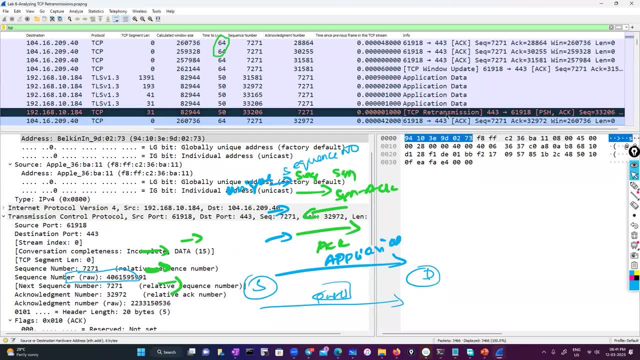 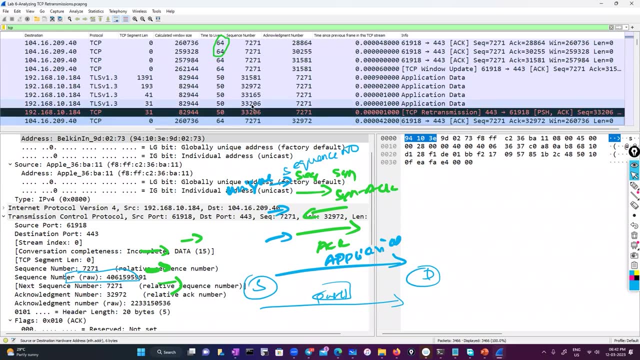 happens. it says you're going to push your data but i haven't received your traffic, what you you sent before. so here comes the role of sequence number. so this particular sequence number for that i didn't get the data for 33026, exactly a packet before this. if you see the calculator, window size is same. 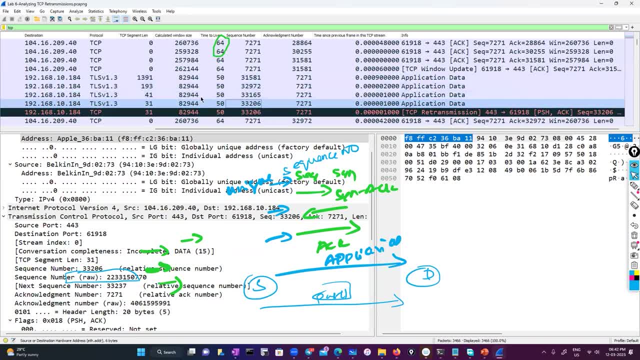 and if you see my calculator, window size is not increasing and it is asking for the retransmission. why, if the window size is not suddenly it's dropped to 80 thousand nine hundred forty four earlier. this is two lakh sixty two thousand hundred and forty. that is because i'm not ready to receive your data. you might be fast enough to send your data, but 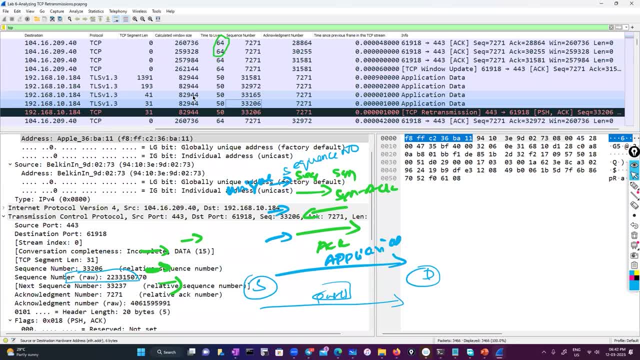 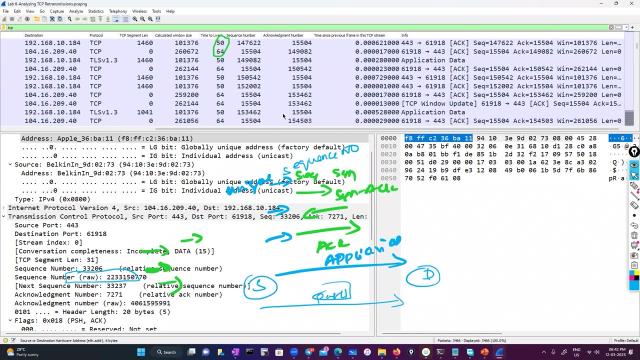 i have a problem here. you have to, you know, send your data slower because i cannot process your data. so the t retransmission, tcp, duplicate acknowledgement, this all happens because of throughput issues. so this is one kind of scenario where i captured. this is see if you see a lot of 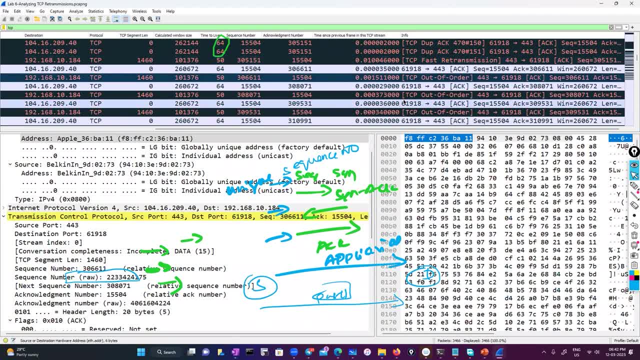 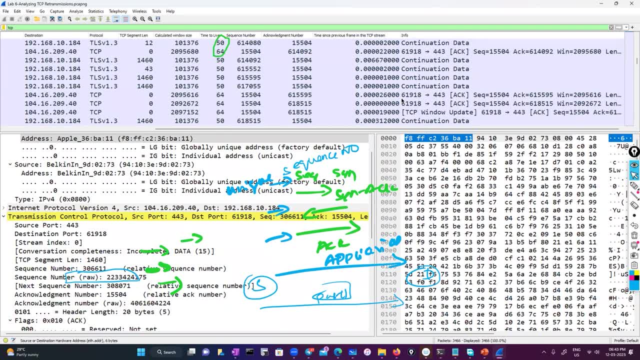 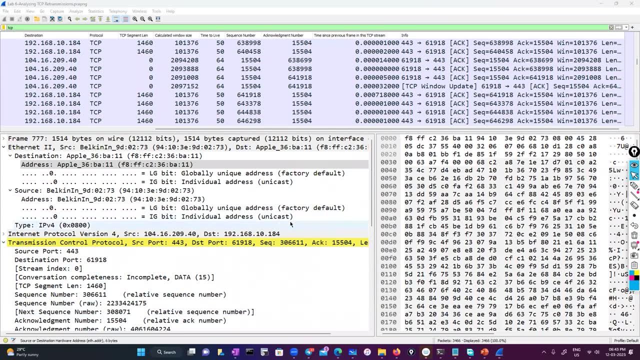 see fast retransmission out of order and all this tcp errors is happening because of a throughput issue. i am dropping your packets here. so this is the level of detail you get from you know, wireshark. so inside the tcp we have different parameter. this is one quick glimpse and you know. 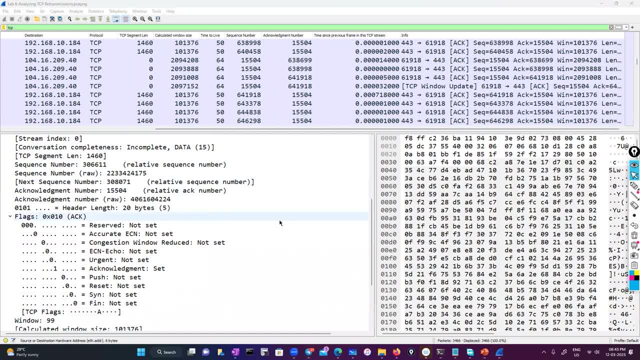 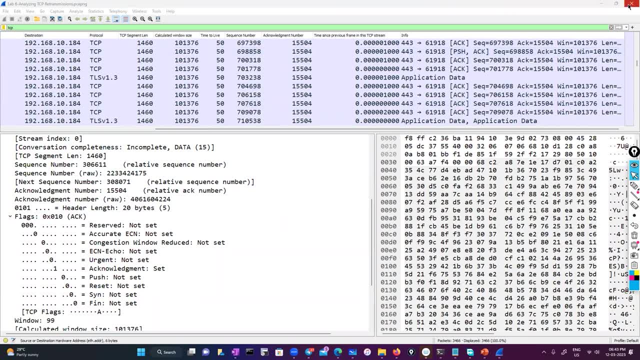 i gave you what, what does this window size and how we, you know, rule out this window size problem? right, and i'll give, i'll show you one more scenario where we had a throughput issue with a different scenario. i'll close this connection and let me open up this, um, okay, 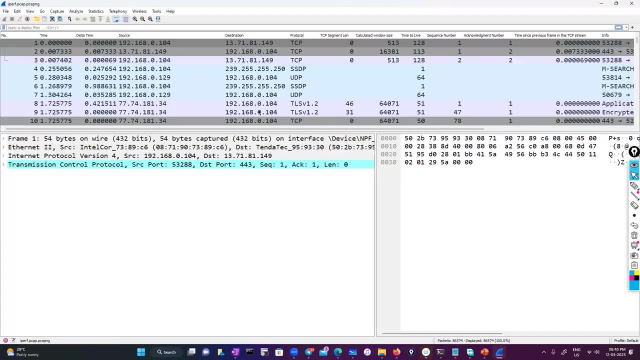 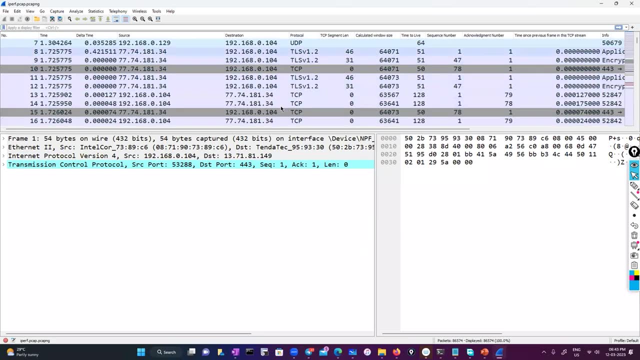 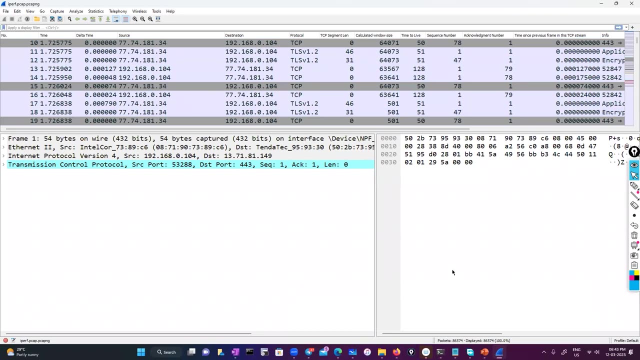 so, before that, let me give you, uh, insight about how exactly we should capture this throughput issue. so i would suggest that there is a tool called ipurf. uh, it is a very, you know, most widely used tool by the network administrator to find the bandwidth. so, before that, 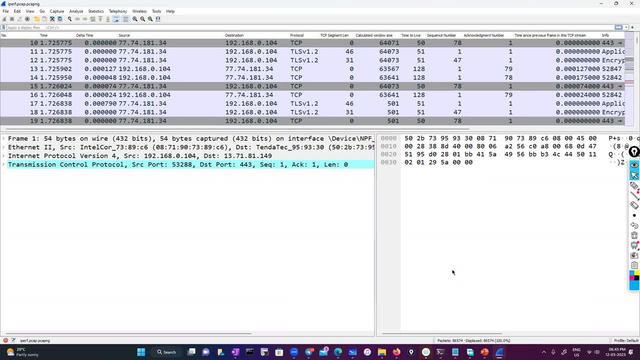 i'll give again an overview of what is bandwidth, what is throughput, what is speed. so my early- i mean when i started a career- i had this confusion. so what people are talking about bandwidth, throughput and speed, what exactly the key difference between all these three and what it really matters here in wireshark? definitely, yes, we should know about all that. 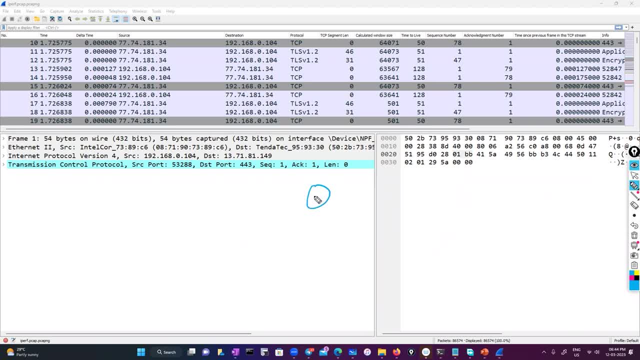 here. so bandwidth example: if you got a link here and you have connected to your isp and this is your switch router, anything that's connected here, this all in use of pcs, so you got your 100 mbps link, at least line connection, guaranteed bandwidth, 100 mbps. so this particular 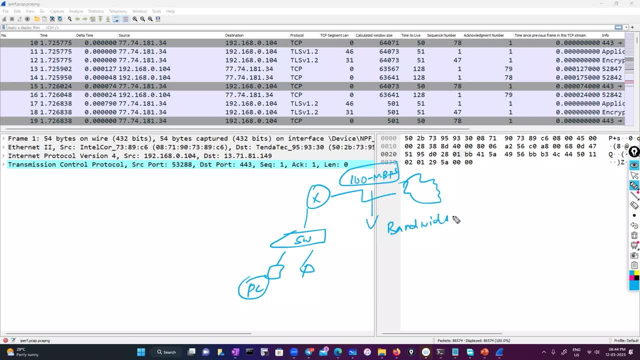 parameter. we call this as a bandwidth, so some so they say it's something problem with your bandwidth and you have some performance issue. that's happening here. so how you figure out that you have to bypass your router. i mean what i mean about bypass or something. i should not use a router. instead, this particular connection that's coming from the isp i have. 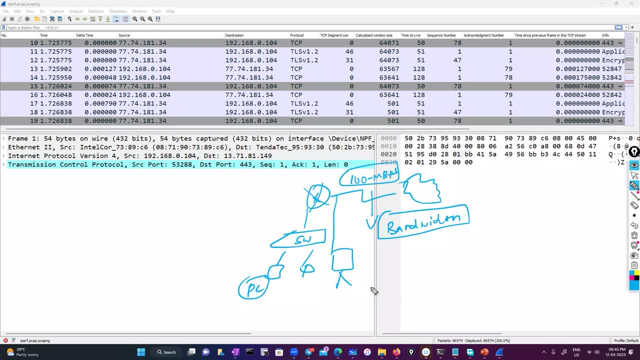 to connect to my laptop and i should do a capture and i should see if any retransmission is happening, like before we have seen. right, sorry for that. let me write it clearly. so i should see if i see any kind of re-transmissions. so i have to figure out that. so before that, using the ipov tool- uh, i did a capture here. 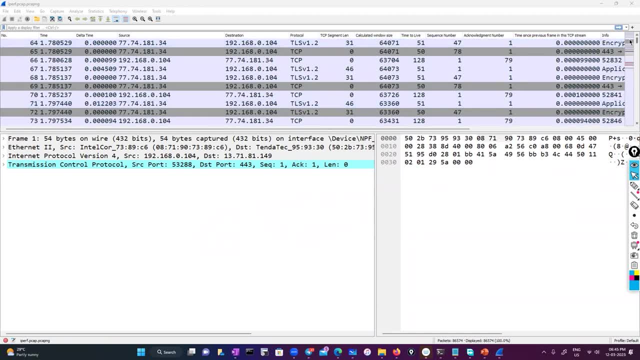 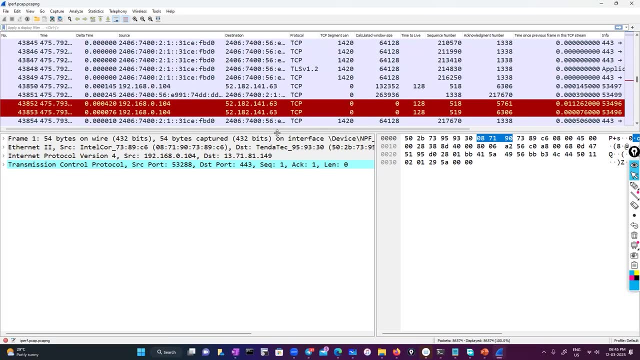 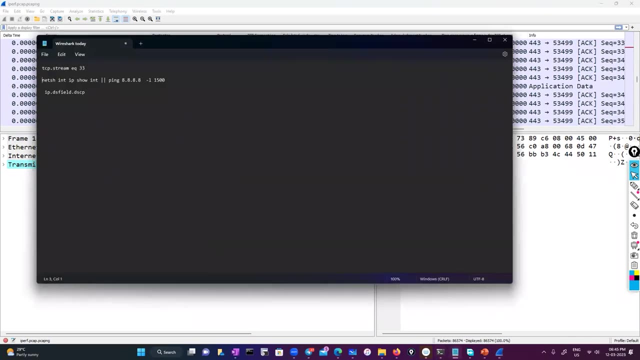 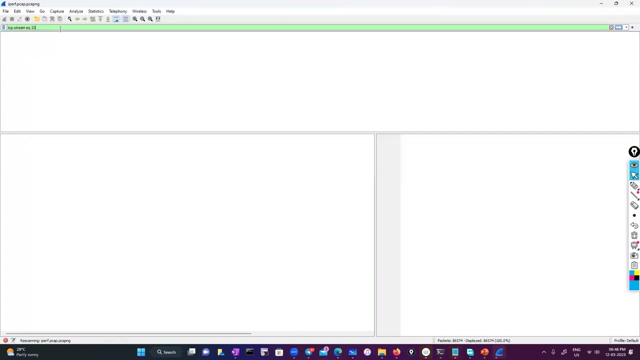 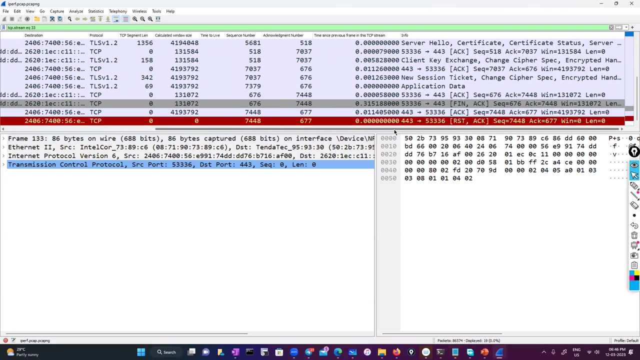 the ipov tool, so where i want to show you exactly where this window problem happened. so if i come back here, this is a reset, so there is a particular filter to figure out this. if you actually see here- see, this is the fin packet- where exactly my communication. 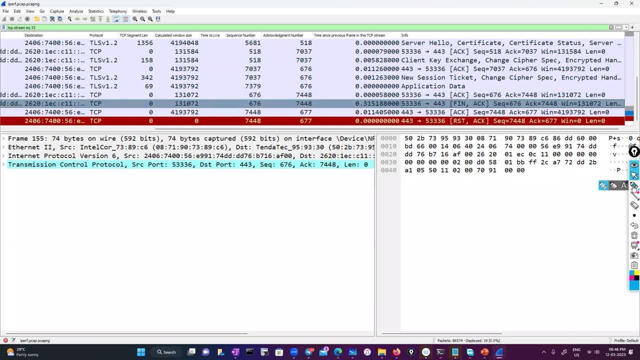 you know, successfully terminated on both ends. so fin when, when fin packet exactly happens, this is a client and this is a server, right? so when there is a successful connection it has to send a sin packet and for that sin it has to send a synac back and it will send a acknowledgement for the synac. 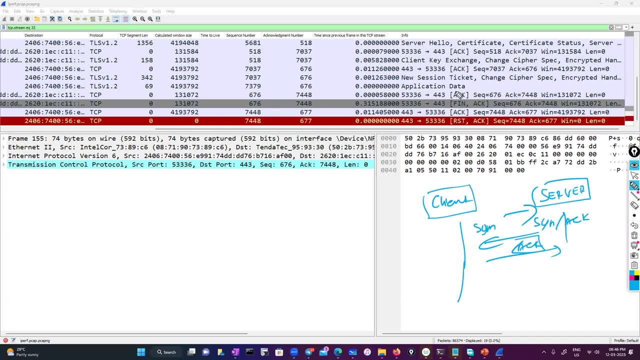 this is a common scenario where, where this particular fax comes in here, i told you push, happens before the fin and finish something. hey, i agree for that. i got all the data in this particular segment. i'm talking about the segment, this particular segment. i got 64 bytes. i got all the data. i am fine. i'm good to close the connection and it's going to set this. 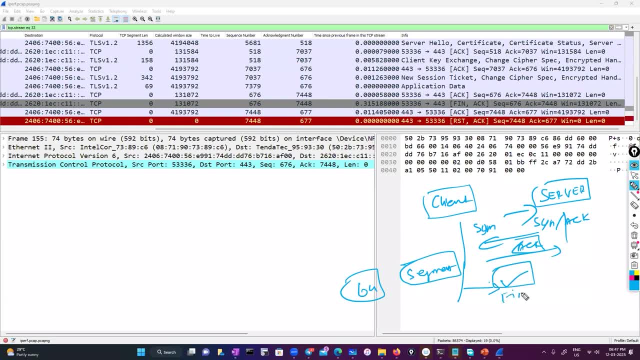 fin file flag set inside tcp from the source and the same way in the destination. it's going to send a fin packet here. it's a mutual agreement to terminate the connection, to close down the connection from the source and destination. it's something like you know, you are talking to your friend. 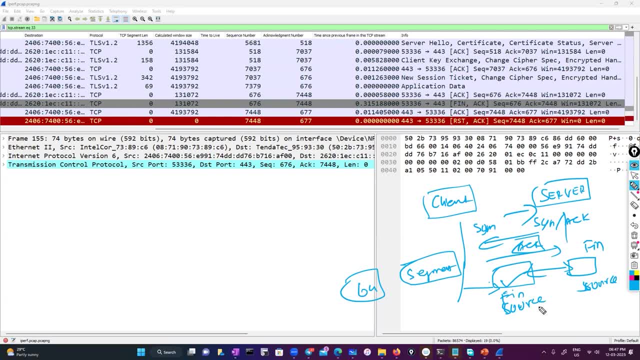 in the phone call and say: i'm done with my conversation, let me disconnect. that's a, you know, mutual understanding between source and destination. so that's how this fin comes here. so why there is a problem with what is this packet? coloring is red because this is a reset. why 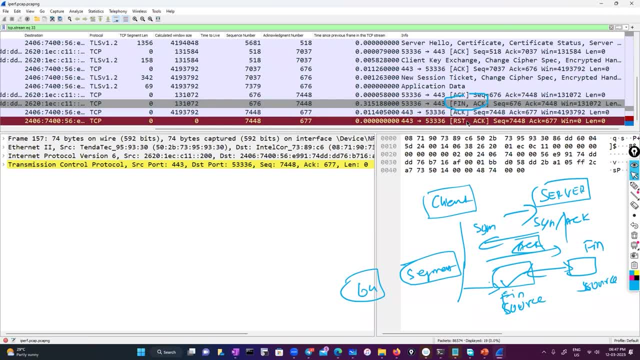 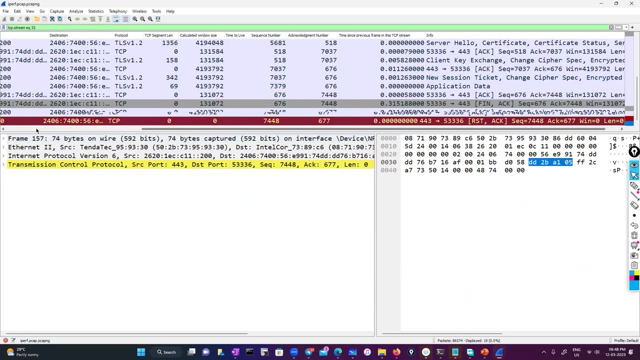 it is a reset. i didn't get your packet. it's abruptly disconnecting a connection, so my tcp conversation is happening here and who is doing this reset? that's a key thing. you have to figure out, okay, where there is a problem with the throughput. so, if you exactly see, this is my 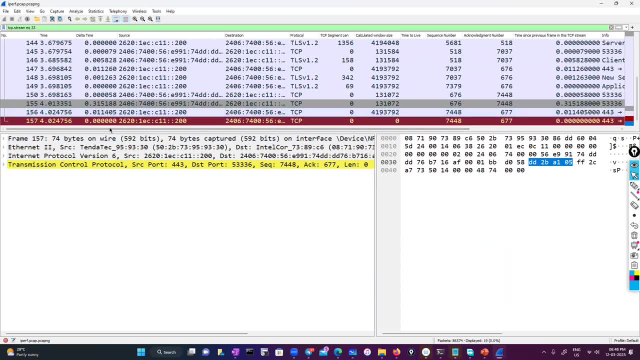 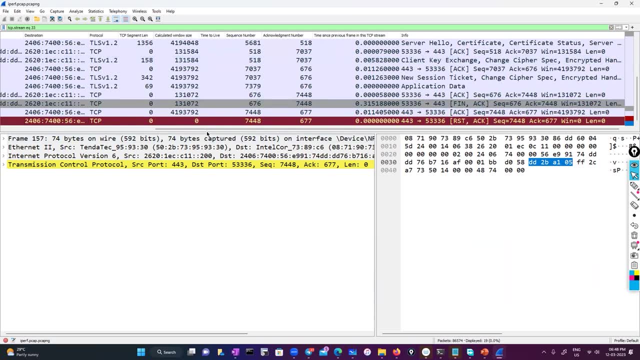 source: pc and this is a destination PPC. because you see this connection, i am going to reset this v4, explain location and here, exactly, if you see, calculated window size is zero. i'm going to reset this connection. i'm not going to propose anything because i am not ready to. 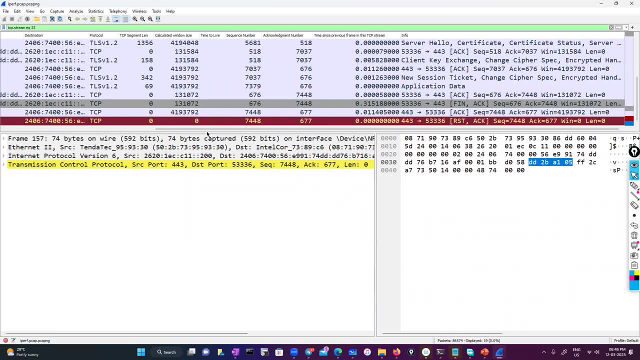 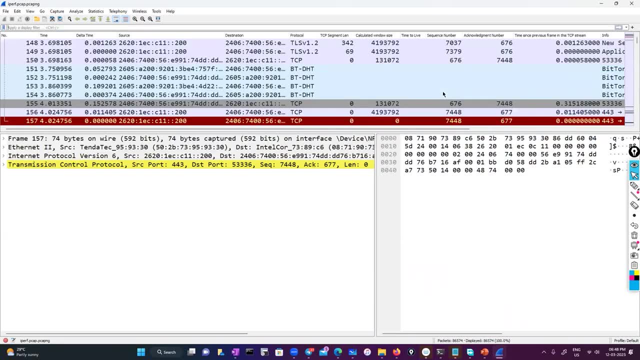 receive anything because i didn't get the previous packet, so i'm going to reset this connection. this connection is not successful. if you see lot of reset packets in your network, then definitely it's a problem, but the key thing is where exactly this is opening happening. that's. 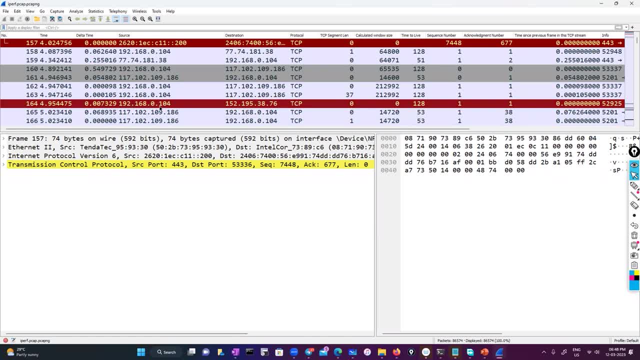 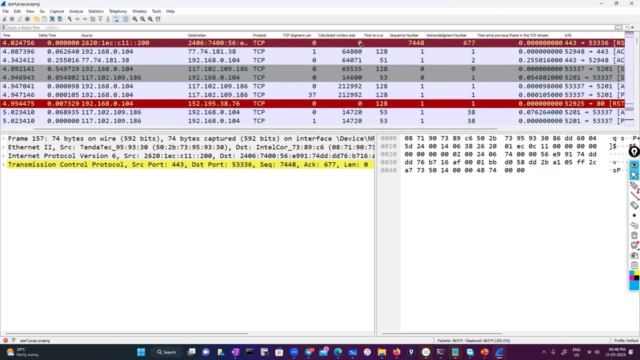 ip address here. this is 192.163.0.104. this is private ip and this is public ip. range 152 and if you see 30 cp segment length for all the reset packets, it's all zero. you see, see the acknowledgements. also, i i'm not acknowledging your actual segment length. 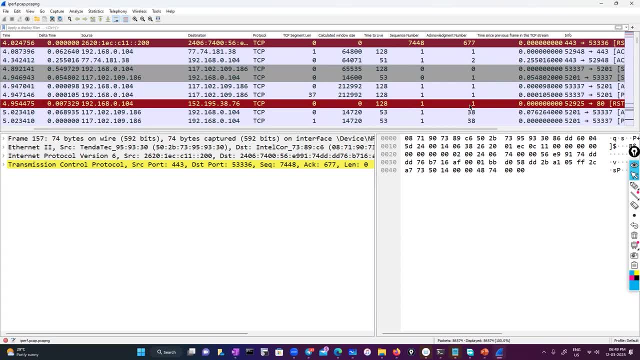 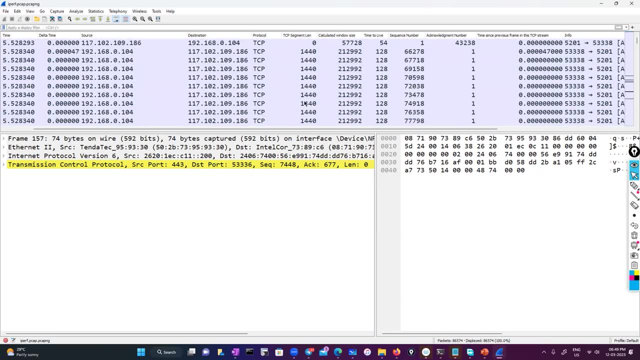 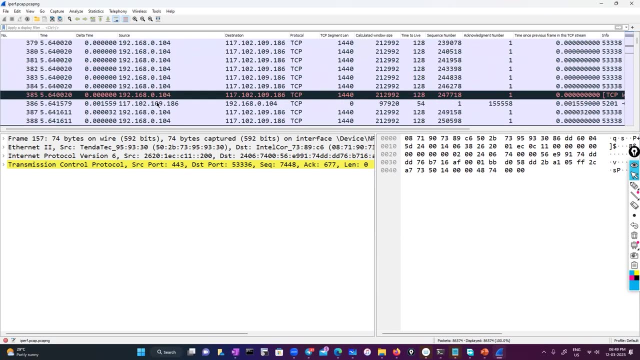 this is something problem. so the real data exchange is not happening at this point. so all this red priorities and this alarm signals, that indicates that there is a problem. but why wireshark is, you know, very helpful at this point i can, i can figure out where exactly this. 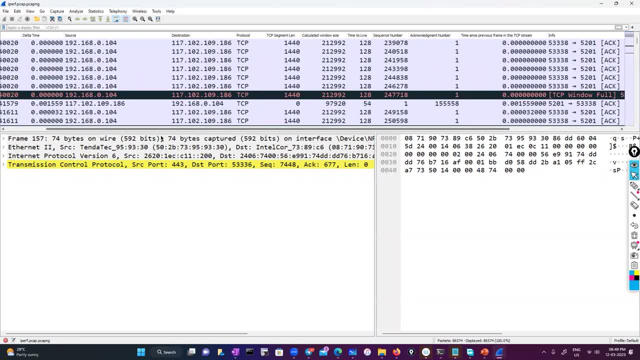 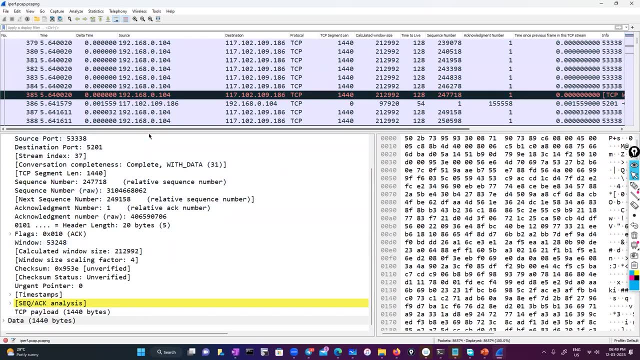 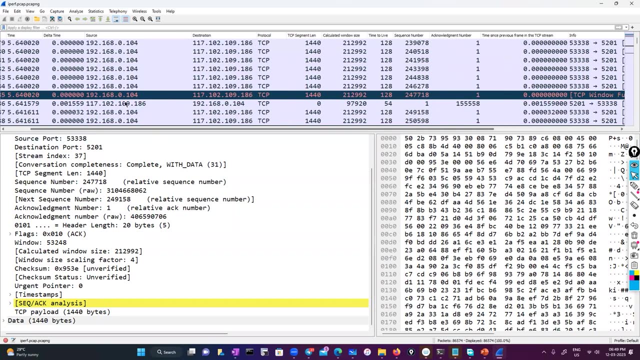 happened. this is what exactly i'm trying to find. see, if this is something i am proposing. i am saying that my tcp window is full. you don't send any kind of data. if you see, after this particular conversation, this part, this is from the client to server. so here we have to see this is very 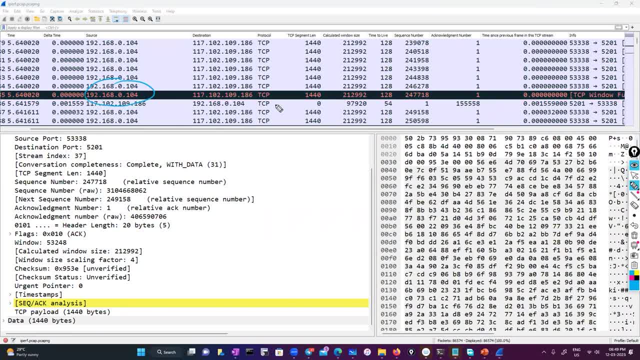 important. so, if i see the client, i got three resets. all happened because of my pc and along with that, this is the destination and this is the calculated window size and this is the sequence number. see, and this is my tcp window is full. it's saying: you don't send any data. i'm not ready to. 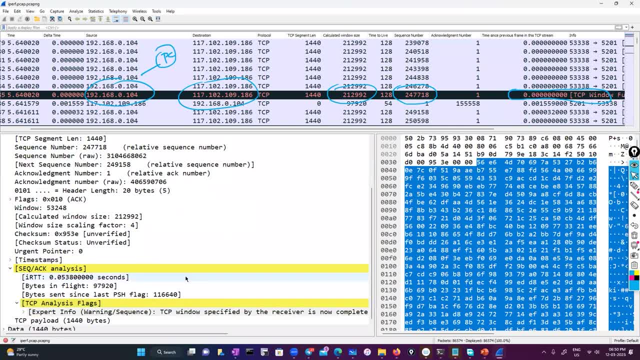 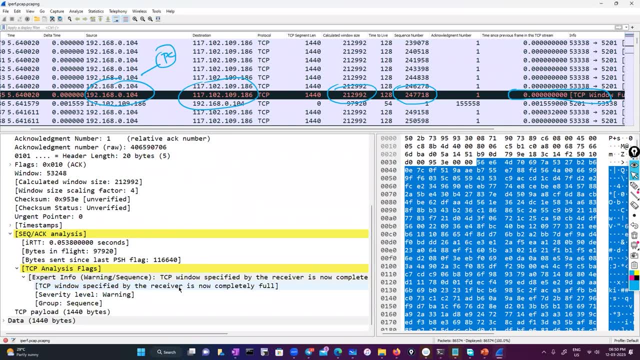 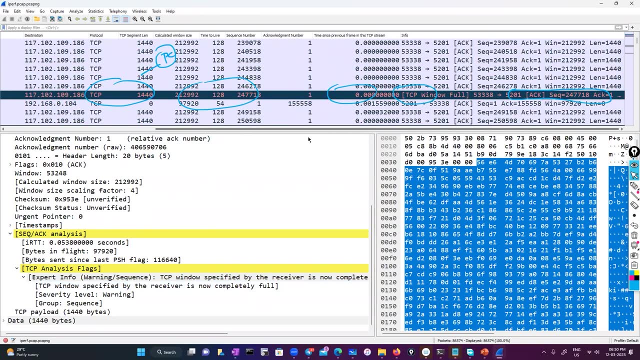 send any data. so i can just say that my tcp window is full. tcp windows specified by the receiver is now completely full. you don't send any data, i'm full. so now i can figure out. okay, this is something problem with my connection. at some point i am dropping packets. i cannot process a packet, but even though the server is ready, 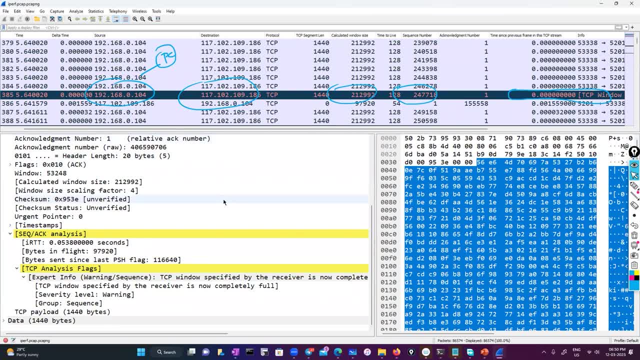 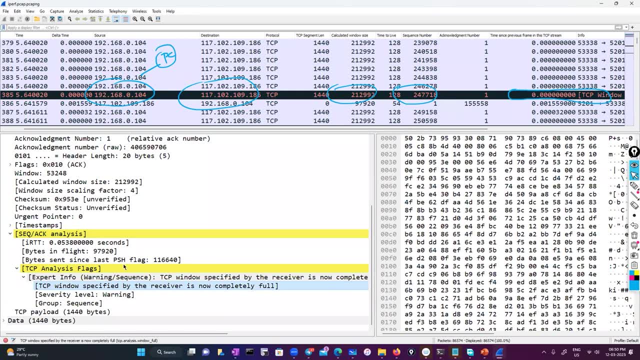 to send the data but i cannot send because my tcp window is full. i cannot receive any more data. this is some kind of proposal, some warning. it says so. now i can go ahead and and say, hey, yeah, i agree, it is something problem with my pc. i have to look into this pc why. 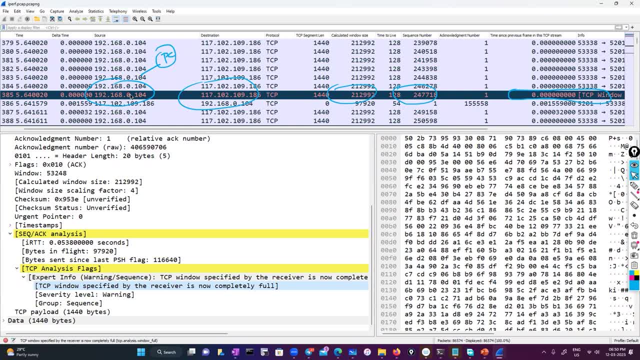 it can happen. maybe this particular pc might have established multiple connections to the internet and it cannot process the packet right, so my particular throughput is low. what's okay? what is throughput here? so when we discussed about bandwidth, i explained what is throughput here. so when we discussed about bandwidth, i explained what is throughput here. 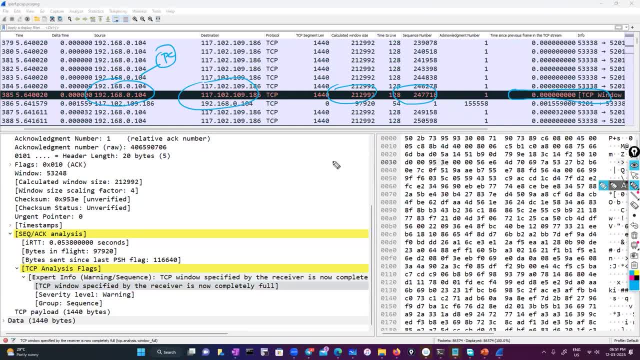 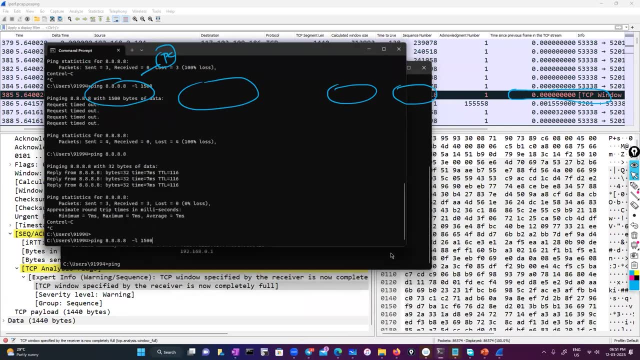 is bandwidth. that is where your actual link speed is your bandwidth. the throughput is something how much i get out of the bandwidth, but how, how i know what is the throughput i get for my pc. so if we go back, let me try to bring up the ipov tool here. 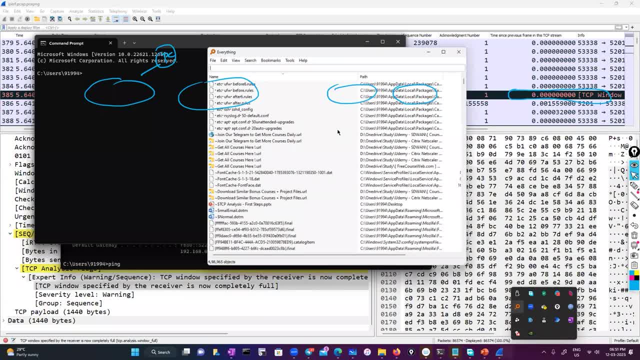 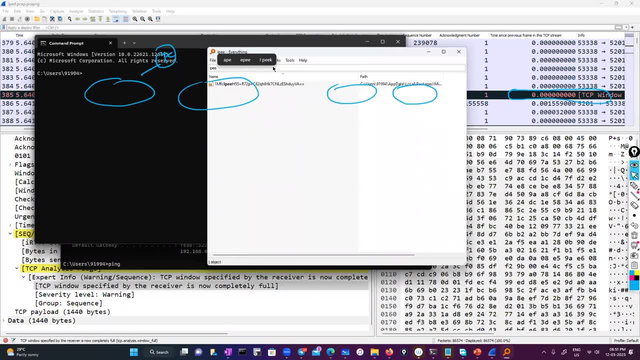 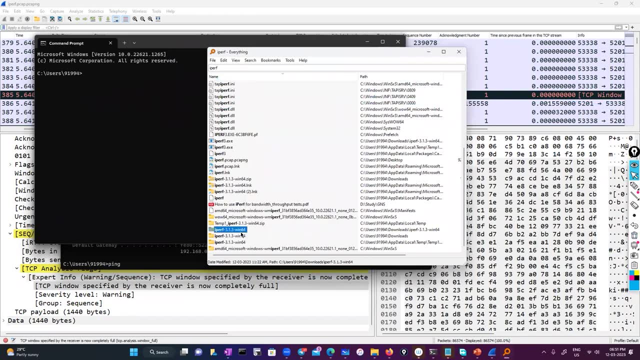 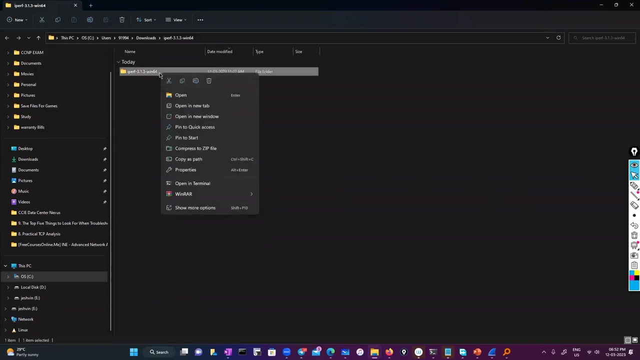 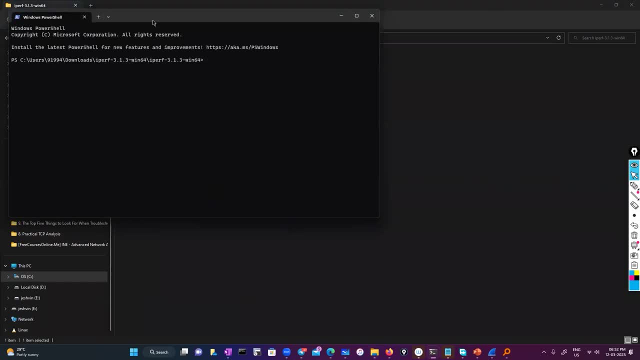 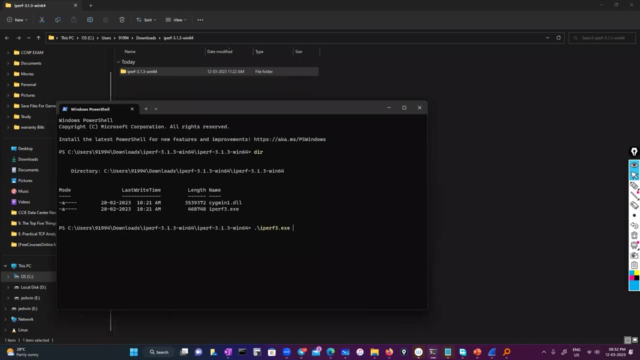 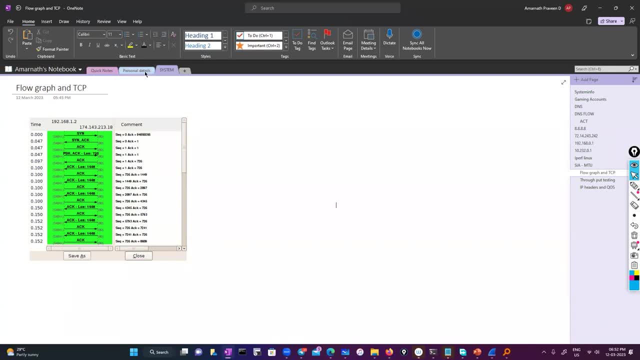 and the there is. there are many you know and the there is there are many you know. ipof uh servers that you can test. i'll ipof uh servers that you can test. i'll ipof uh servers that you can test. i'll tell you what is the ipo server. so we 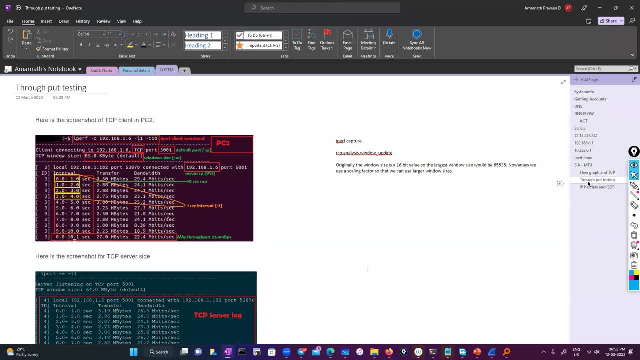 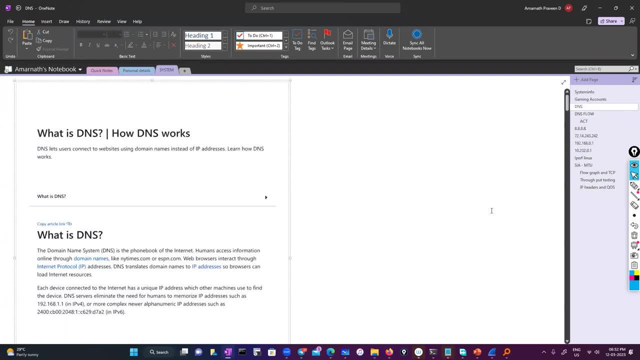 tell you what is the ipo server, so we tell you what is the ipo server. so we will do, will do, will do ipof testing, ipof testing, ipof testing. so let me check, so let me check, so let me check dns flow here, dns flow here. 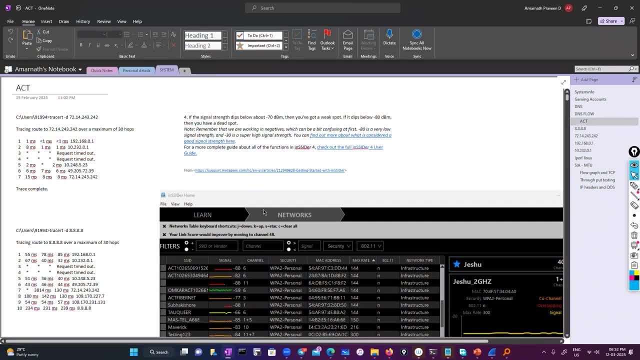 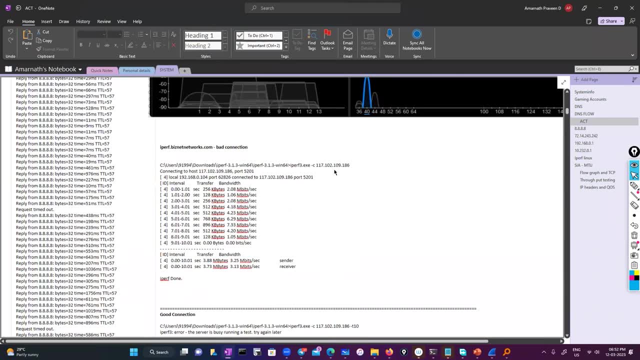 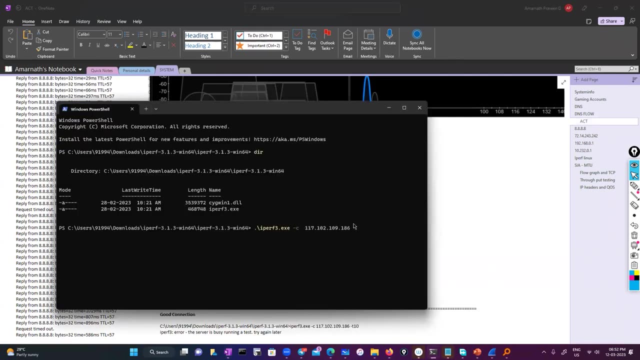 dns flow here dns, dns flow here, dns. this is a place where exactly i did an. this is a place where exactly i did an. this is a place where exactly i did an ipof, ipof, ipof for the public server. okay, so now i'm connected. so they say: 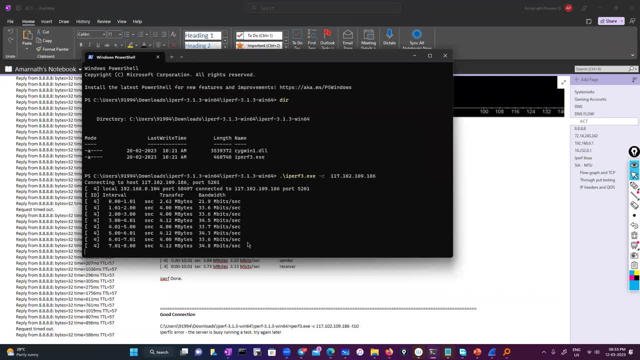 okay, so now i'm connected. so they say: okay, so now i'm connected. so they say: you've got 100 mbps link, you've got 100 mbps link, you've got 100 mbps link. so here are the key things we have to. 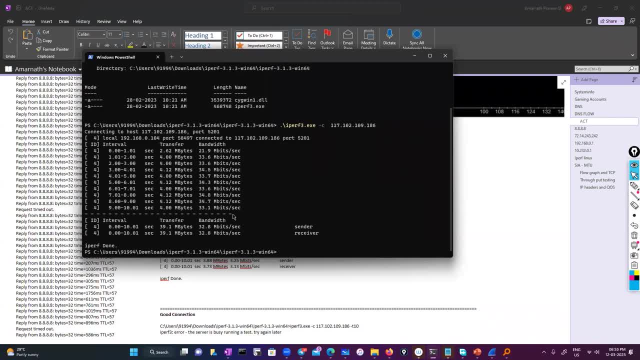 so here are the key things we have to. so here are the key things we have to understand here. so we'll see what is the understand here. so we'll see what is the understand here. so we'll see what is the throughput: throughput, throughput, throughput. okay, see per second, what is the throughput i? 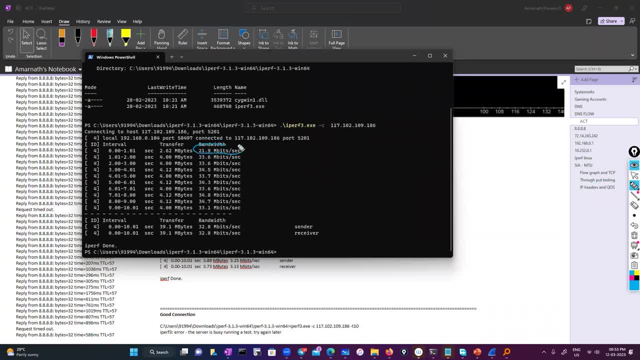 see per second. what is the throughput? i see per second. what is the throughput? i get here. so this is the guaranteed get here. so this is the guaranteed get here. so this is the guaranteed bandwidth. bandwidth, bandwidth. so i got 100 mbps link and how much i. 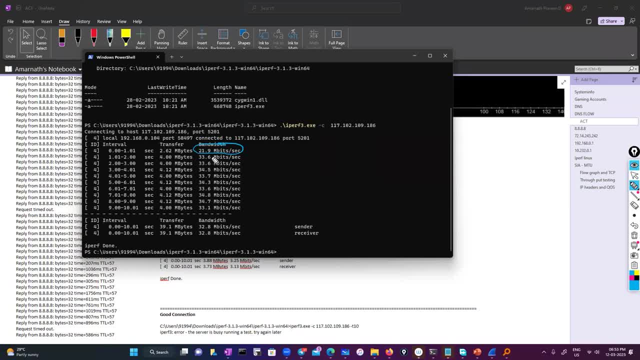 so i got 100 mbps link and how much i so i got 100 mbps link and how much i can send per pc. this particular pc can can send per pc. this particular pc can can send per pc. this particular pc can send, send, send. you know this particular speed for this. 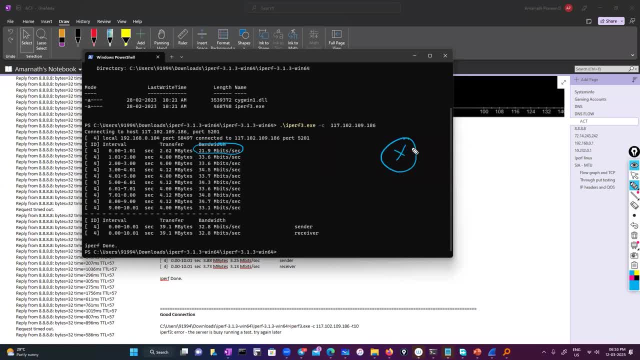 you know this particular speed for this. you know this particular speed for this pc. you got it right. this is a guaranteed pc. you got it right. this is a guaranteed pc. you got it right. this is a guaranteed bandwidth: 100 mbps. bandwidth: 100 mbps. 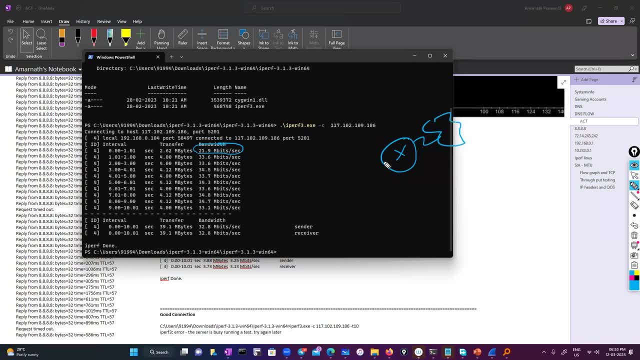 bandwidth 100 mbps. but that particular 100 mbps is not. but that particular 100 mbps is not. but that particular 100 mbps is not completely, completely completely given for my pc. it's a shared given for my pc, it's a shared. 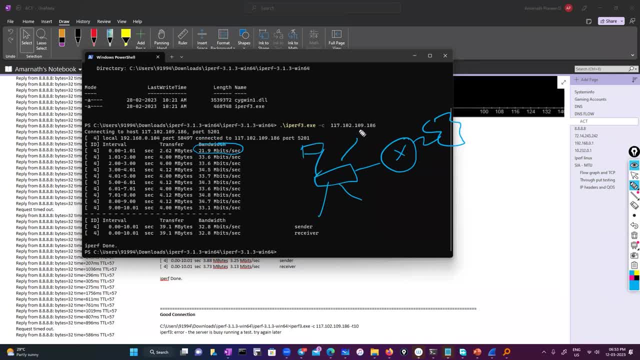 given for my pc. it's a shared bandwidth, bandwidth, bandwidth. so now i have connected my computer, my, so now i have connected my computer, my, so now i have connected my computer, my tv is consuming a few bandwidth and my tv is consuming a few bandwidth and my 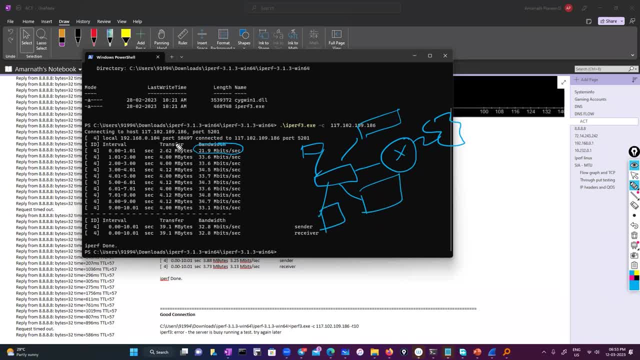 tv is consuming a few bandwidth and my mobile is consuming few bandwidth and my mobile is consuming few bandwidth and my mobile is consuming few bandwidth and my laptop, laptop, laptop, and i got a guaranteed bandwidth and and i got a guaranteed bandwidth and and i got a guaranteed bandwidth and this is the throughput i can send 21.9. 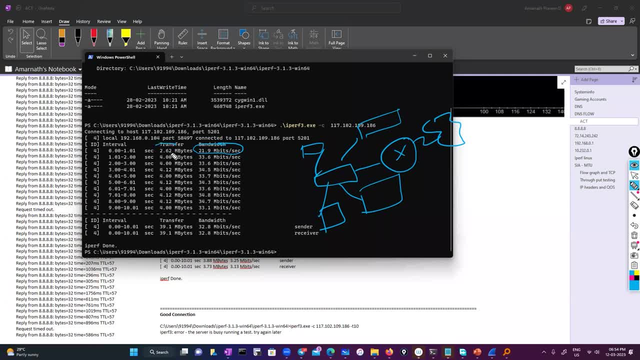 this is the throughput i can send 21.9. this is the throughput i can send 21.9. is the interval is between every second. is the interval is between every second? is the interval is between every second? i'm sending this data. i'm sending this data. 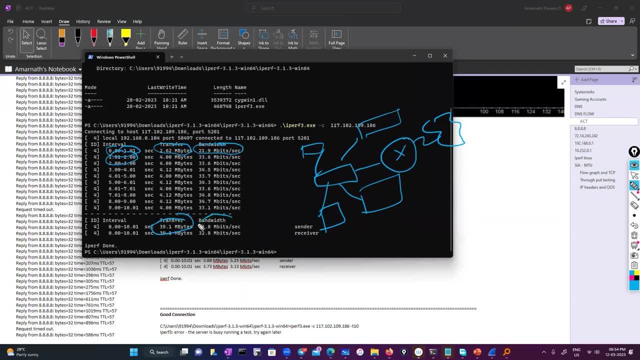 i'm sending this data, so this is your average data sent, and so this is your average data sent, and so this is your average data sent, and this is your average throughput, and one point of time where my pc it and one point of time where my pc it. 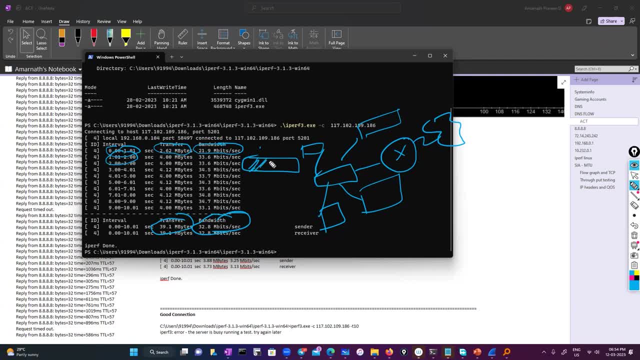 and one point of time where my pc it says hey, my says hey, my says hey, my, my tcp window size is full. you don't, my tcp window size is full. you don't, my tcp window size is full. you don't send any data. send any data. 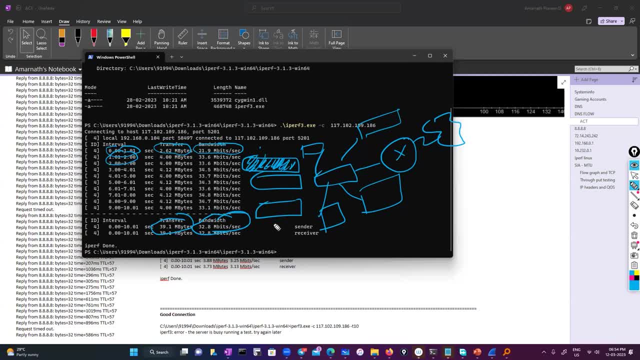 send any data until i process this packet and i'll send until i process this packet. and i'll send until i process this packet and i'll send out a new proposal where i i know i'll out a new proposal where i i know i'll out a new proposal where i i know i'll propose the new window size. 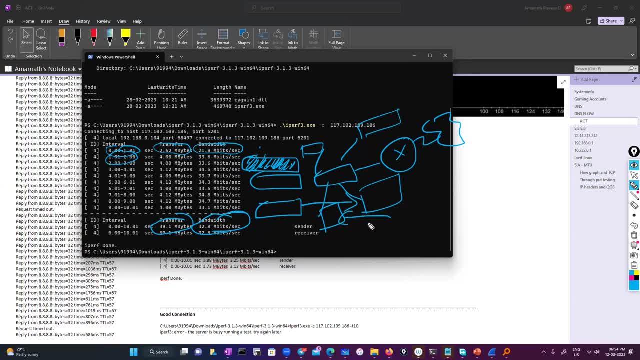 propose the new window size, propose the new window size and then, after you know, after that, you and then, after you know, after that, you and then, after you know, after that, you can send your data back, and i am ready, can send your data back, and i am ready. 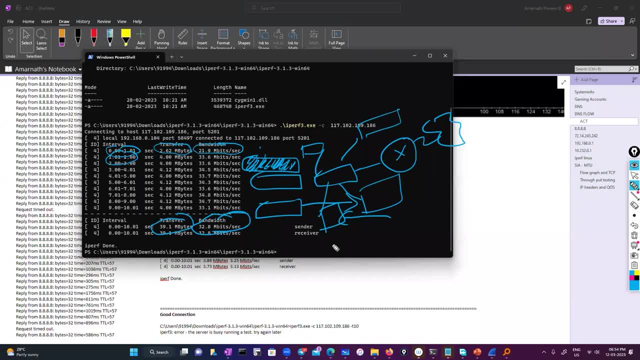 can send your data back and i am ready to receive so, but at this point of time, to receive so, but at this point of time to receive so, but at this point of time. no, my window size is full. no, my window size is full. no, my window size is full. so that that is the use of window size. 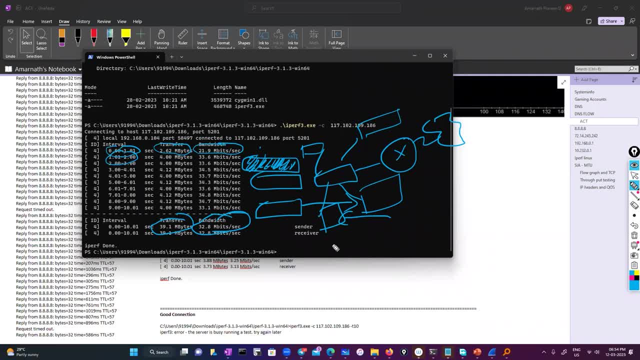 so that that is the use of window size. so that that is the use of window size. that's why we, that's why we, that's why we- we should know about windows. so where is we should know about windows? so where is we should know about windows? so where is the problem? so here: 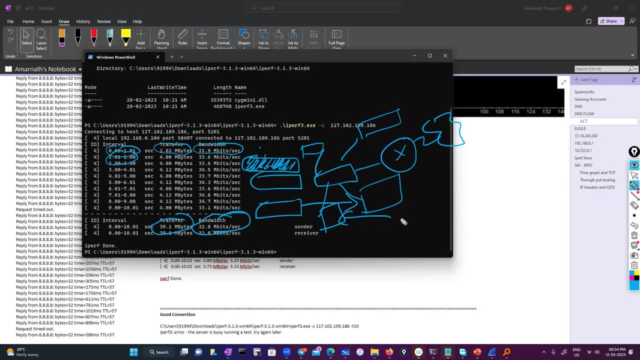 the problem. so here the problem. so here, my bandwidth is fine, my transfer rate, my bandwidth is fine, my transfer rate, my bandwidth is fine, my transfer rate is fine, my internet is fine. but i come to is fine, my internet is fine, but i come to is fine. my internet is fine, but i come to know it's because of the tcp. know it's because of the tcp. know it's because of the tcp, since my window size is full, i cannot. since my window size is full, i cannot. since my window size is full, i cannot. process a packet i'm busy with. process a packet i'm busy with. 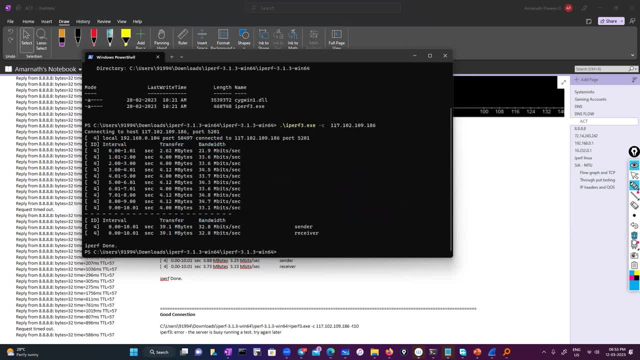 process a packet. i'm busy with other connection. established connection. yeah, this is about you know real-time. yeah, this is about you know real-time. yeah, this is about you know real-time scenario where where we we often scenario, where where we we often scenario, where where we we often experience this problem. that's something. 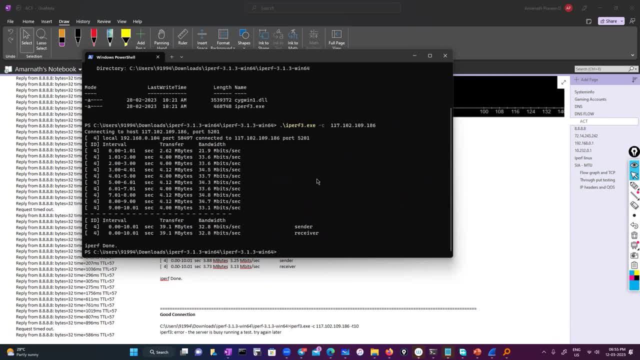 experience this problem, that's something. experience this problem, that's something. people they keep barking about this. people they keep barking about this. people they keep barking about this: throughput issues, throughput issues, throughput issues. so you can make use of ipof and when i, so you can make use of ipof and when i, 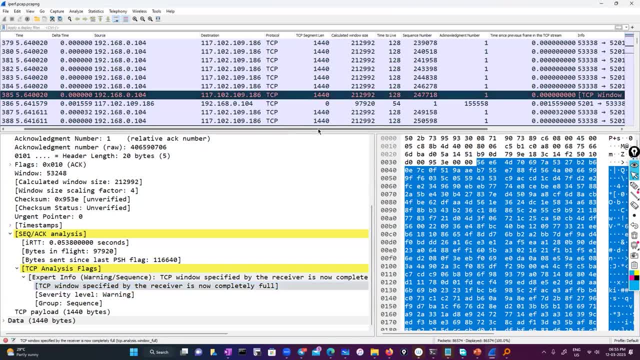 so you can make use of ipof. and when i did an ipof- this is a capture- i exactly did an ipof. this is a capture. i exactly did an ipof. this is a capture i exactly did and where exactly it said that okay did and where exactly it said that okay. 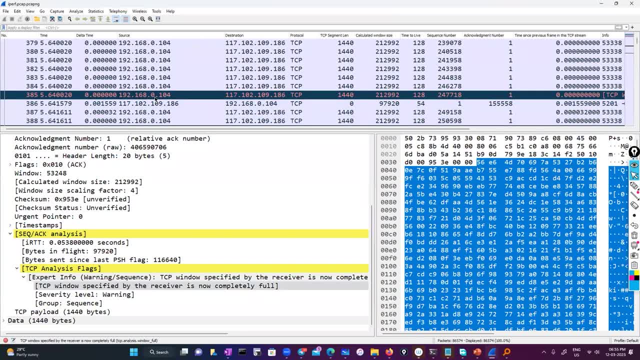 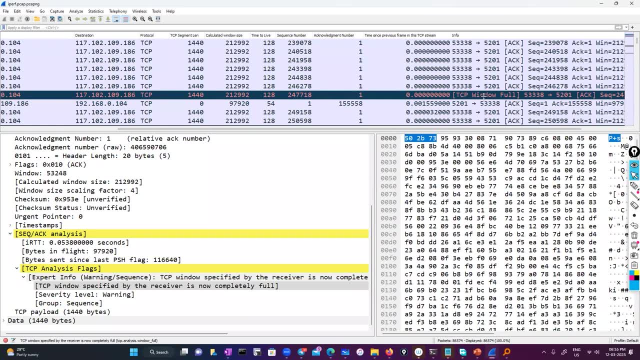 did and where exactly it said that: okay, my, my, my, my pc is proposed a window size. it says: my pc is proposed a window size. it says: hey, i am full, you don't send anything. hey, i am full, you don't send anything. hey, i am full, you don't send anything because my tcp window is full. 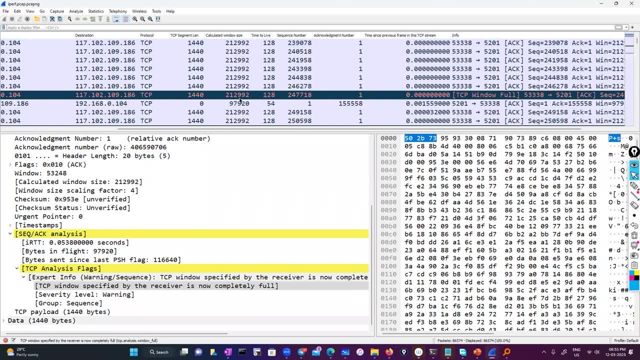 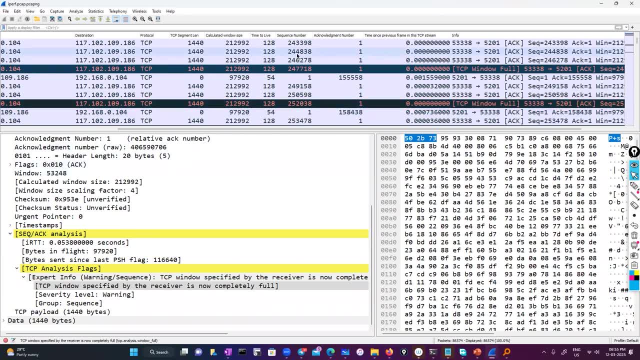 because my tcp window is full. because my tcp window is full. here you can see my calculator window, here you can see my calculator window. here you can see my calculator window size. here it is full. yeah, that's it about, uh, the throughput. yeah, that's it about, uh, the throughput. 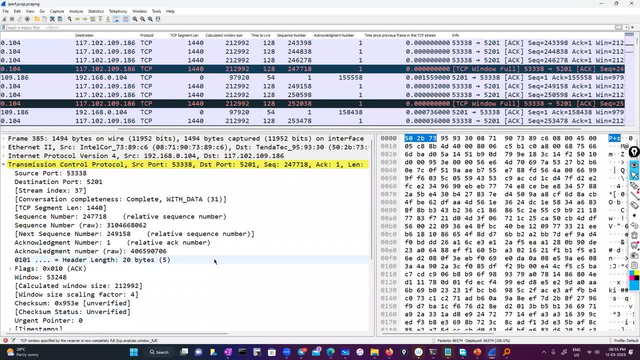 yeah, that's it about. uh, the throughput issue issue issue. uh, you, you have more details in the real. uh, you, you have more details in the real. uh, you, you have more details in the real: classes, classes, classes. uh, this is one scenario we have so many. uh, this is one scenario we have so many. 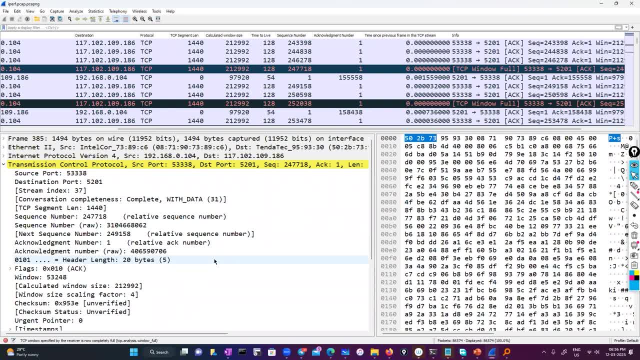 uh, this is one scenario. we have so many interesting topics like how we do the interesting topics like how we do the interesting topics like how we do the same for udp traffic, same for udp traffic, same for udp traffic, and every packet that's guaranteed you and every packet that's guaranteed you. 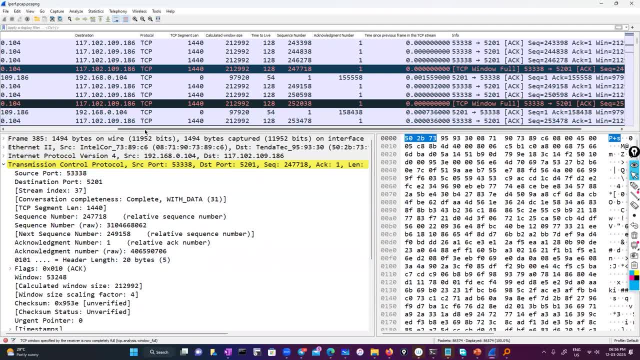 and every packet. that's guaranteed you. you can definitely figure out, where you can definitely figure out where you can definitely figure out where exactly the problem is. exactly the problem is, exactly. the problem is: if you see here it proves again, i got a. if you see here, it proves again, i got a. 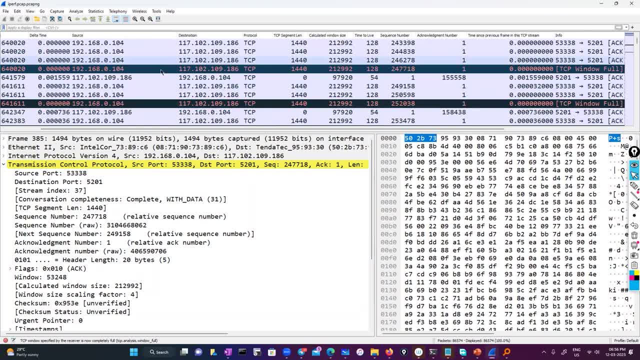 if you see here it proves again. i got a tcp window full error again from my tcp window. full error again from my tcp window. full error again from my client, client, client. it's, it's very visible, it's, it's my pc, it's, it's very visible, it's, it's my pc. 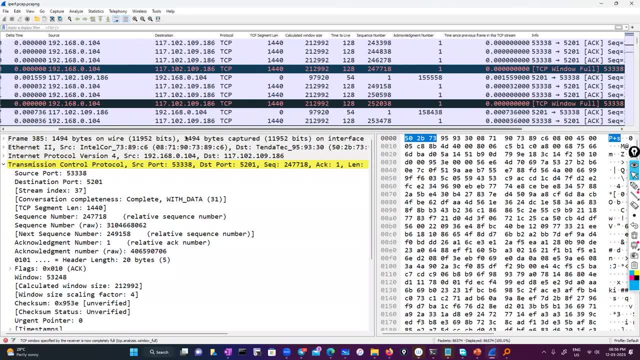 it's. it's very visible. it's. it's my pc. it's my pc. it's not about the bandwidth. it's. it's not about the bandwidth. it's. it's not about the bandwidth. this is something i have you know many. this is something i have, you know many. 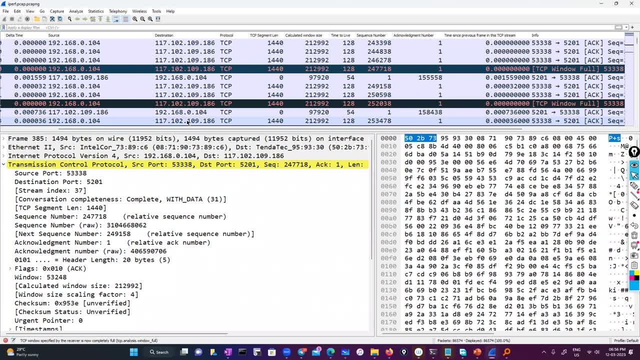 this is something i have, you know, many connections running, so from there, i have connections running, so from there, i have connections running, so from there, i have to drill down, to drill down, to drill down. what is the problem so? the problem is the. what is the problem so? the problem is the. 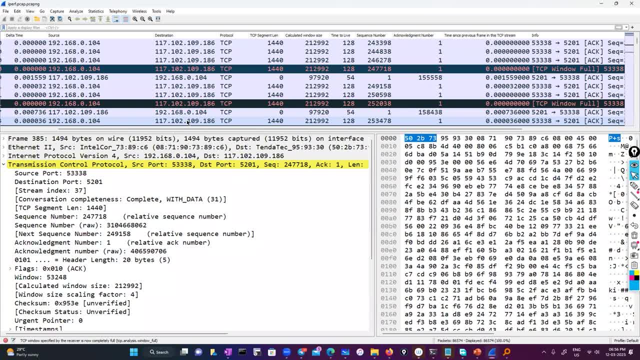 what is the problem? so the problem is the. what is the biggest takeaway of this? what is the biggest takeaway of this? what is the biggest takeaway of this? scenario is scenario is scenario is you can figure out exactly where the. you can figure out exactly where the. you can figure out exactly where the problem is. that's the root cause and we. 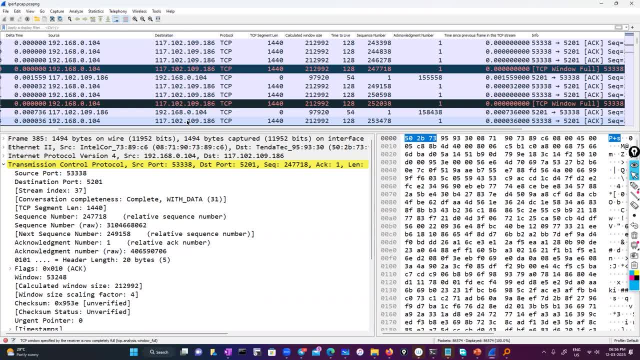 problem is that's the root cause and we problem is that's the root cause and we always have problem in finding that. we always have problem in finding that. we always have problem in finding that we don't know where is the root cause and don't know where is the root cause, and 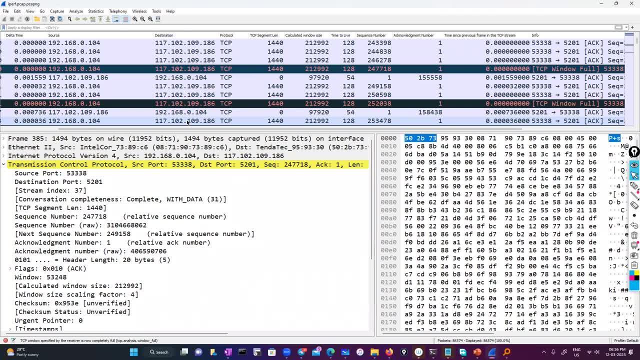 don't know where is the root cause, and you are, you know, rattling around to find you are, you know, rattling around to find, you are, you know, rattling around to find where exactly the problem is that, the where exactly the problem is that, the where exactly the problem is that the root clause is the main thing. so, from 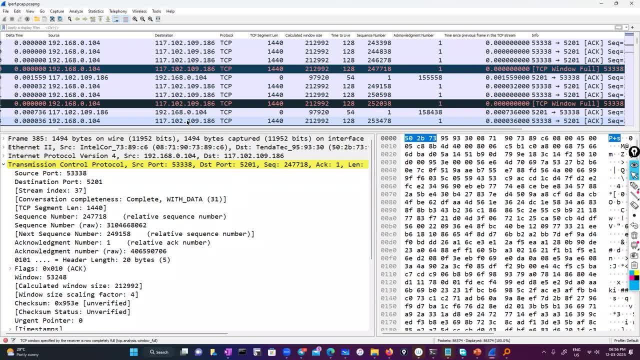 root clause is the main thing. so from root clause is the main thing. so from there we have to dig deeper, and there we have to dig deeper, and there we have to dig deeper and figure out where, figure out where, figure out where, why this particular pc is proposing. 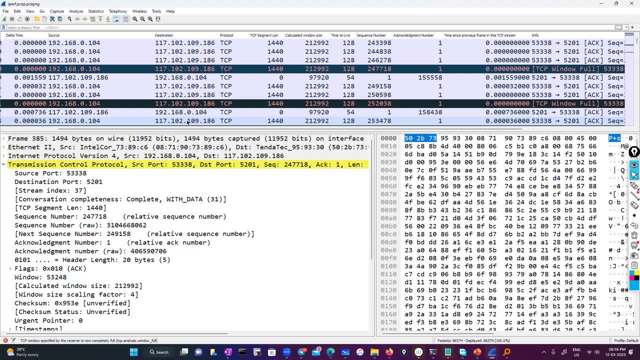 why this particular pc is proposing, why this particular pc is proposing your pcb into a size, your pcb into a size, your pcb into a size as in you know it says i am full. you as in you know it says i am full. you as in you know it says i am full. you be a problem with my internet link nodes. 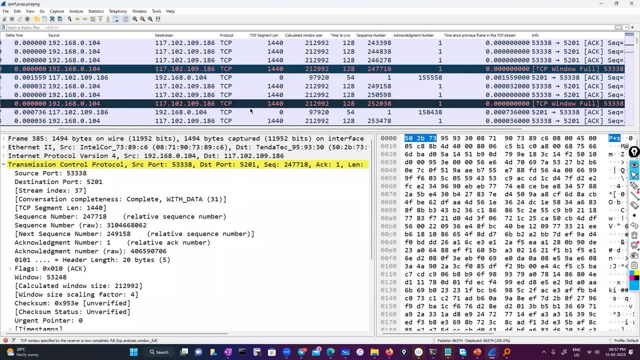 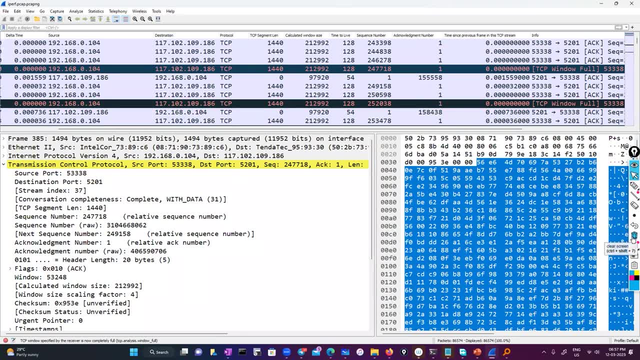 be a problem with my internet link nodes, be a problem with my internet link nodes, all clean. so this is all about the throughput. so this is all about the throughput. so this is all about the throughput and a quick overview about and a quick overview about and a quick overview about empty mtu and mss. 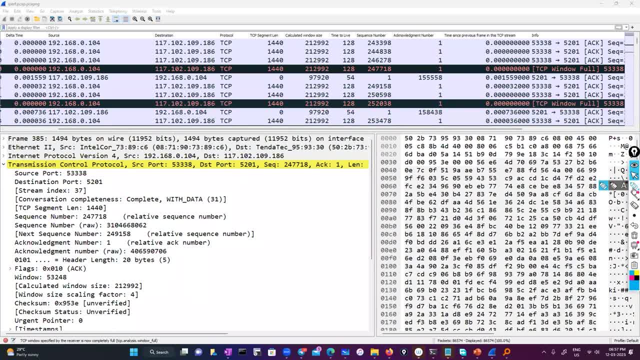 empty mtu and mss. empty mtu and mss. so this is a major confusion. many people so this is a major confusion. many people so this is a major confusion. many people. they have, you know, even i had questions. they have, you know, even i had questions. 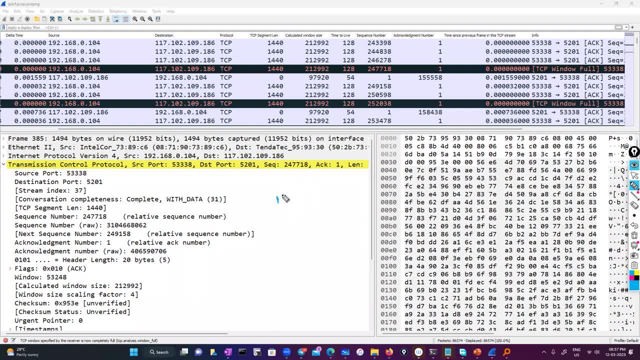 they have. you know, even i had questions: uh four, five years back. what is the what? uh four, five years back? what is the what? uh four five years back? what is the? what is uh the difference between mss and is uh the difference between mss and? 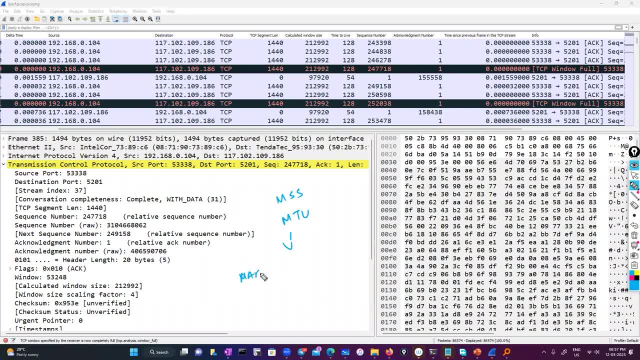 is uh the difference between mss and mtu. mtu is a maximum, mtu mtu is a maximum, mtu mtu is a maximum transmission unit. it comes under your ethernet header. the maximum value is 1500 bytes. why this is important? let's discuss: 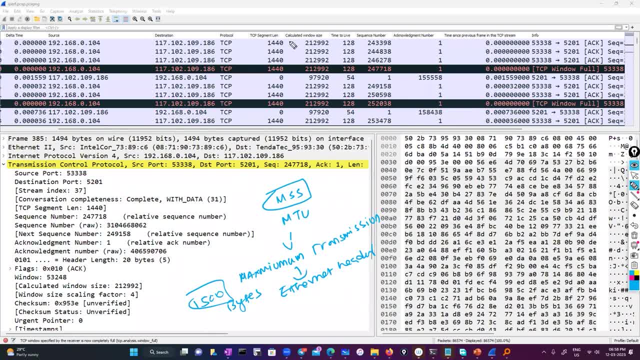 why this is important. let's discuss why this is important. let's discuss about some maximum segment, about some maximum segment, about some maximum segment. size is size. is size is for tcp, for tcp, for tcp. what is your maximum segment size there? what is your maximum segment size there? 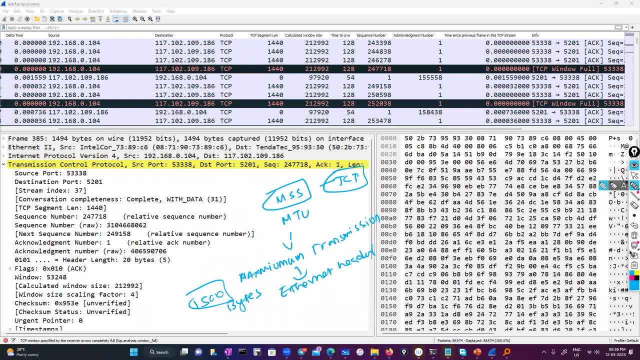 what is your maximum segment size? there is a limitation for it is a limitation for it is a limitation for it. so i'll give you a visual about how it. so i'll give you a visual about how it. so i'll give you a visual about how it looks like. 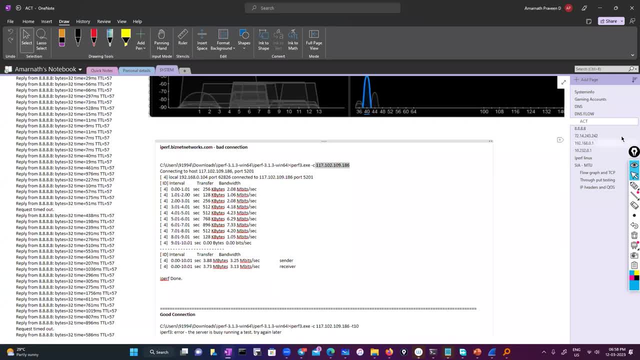 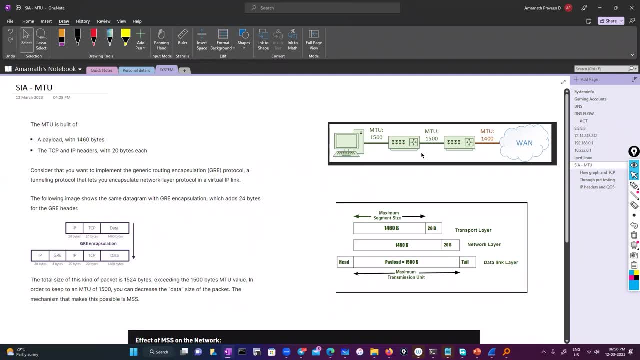 from the wireshark perspective. let me go to mtu, so mtu is. let me go to mtu, so mtu is. let me go to mtu, so mtu is. layer two and it has to match. see if layer two and it has to match, see if. 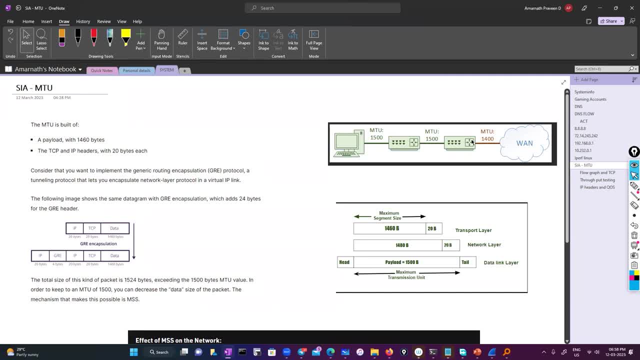 layer two and it has to match. see if you have, you have, you have set your mtu as thousand. finally, if you set your mtu as thousand. finally, if you set your mtu as thousand. finally, if you see here, if there is an mtu mismatched. 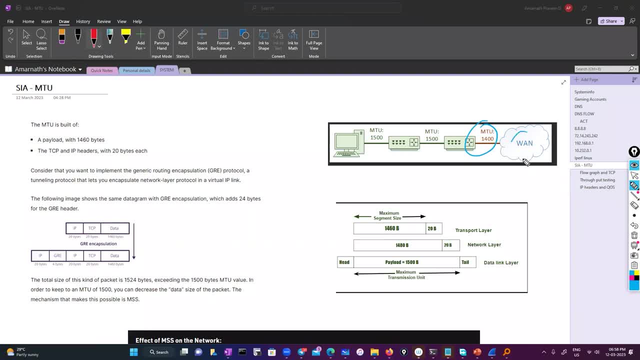 see if there is an mtu mismatched. see if there is an mtu mismatched. your connection is not going to happen. so you can find everything in wireshark. so you can find everything in wireshark. so you can find everything in wireshark. how do we find an mtu mismatch? 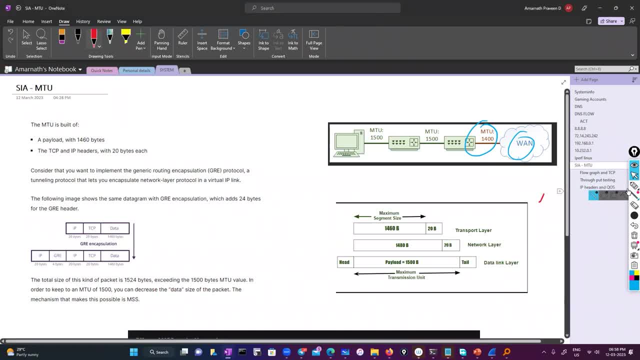 and if you see here this mss maximum and if you see here this mss maximum and if you see here this mss maximum, segment size, segment size, segment size, santi cp, some tcp layer and if you see the maximum, some tcp layer and if you see the maximum, 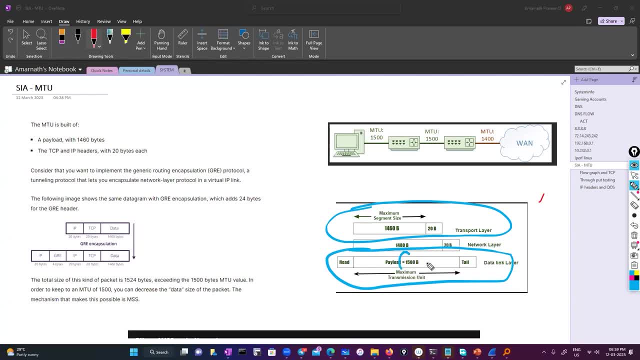 some tcp layer and if you see the maximum transmission unit, transmission unit, transmission unit: 1500 bytes and it's in the layer 2- 1500 bytes. and it's in the layer 2- 1500 bytes. and it's in the layer 2, ethernet header. 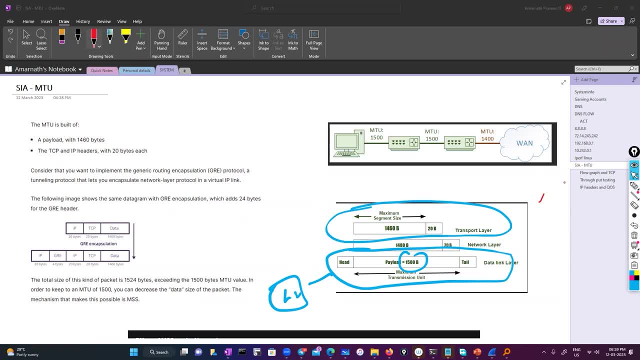 and you i'm people from networking and you i'm people from networking and you i'm people from networking. background, they, they might encounter this background. they, they might encounter this background. they, they might encounter this. i mean they, they would adjust the. i mean they, they would adjust the. 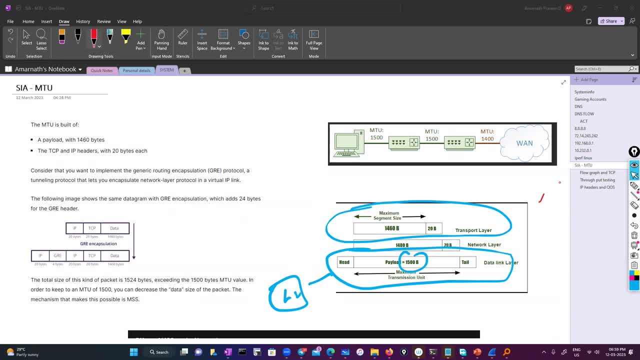 i mean they, they would adjust the mss value in the mss value in the mss value in the gre header, gre header, gre header, so generally in the in the ip header. i'll so generally in the in the ip header, i'll so generally in the in the ip header. i'll give an insight and insight in the ip. 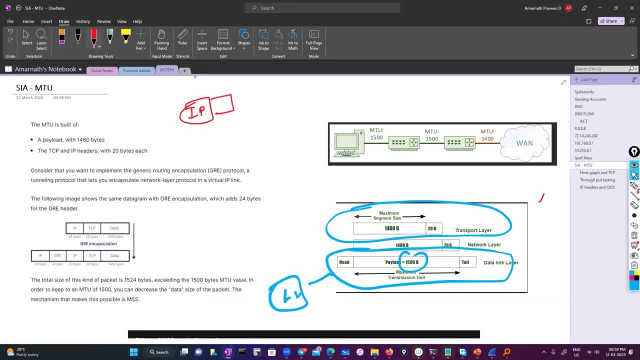 give an insight and insight in the ip. give an insight and insight in the ip header, header header right in inside the ip header. there is right in inside the ip header. there is right in inside the ip header. there is one more header is called gre header. why this is used? because, if i 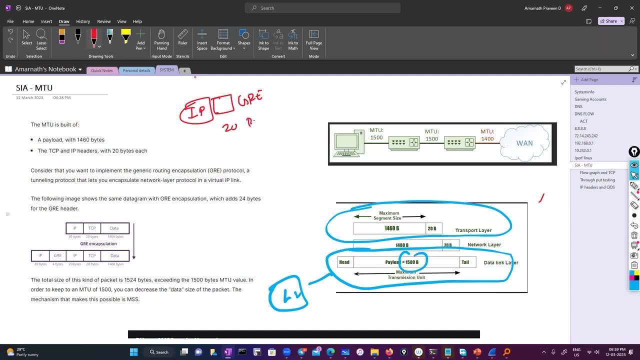 why this is used. because, if i, why this is used? because if i, if i want my, because my id packets is, if i want my, because my id packets is, if i want my, because my id packets is 20 bytes, 20 bytes, 20 bytes, and if i add this gre header, it's a 2. 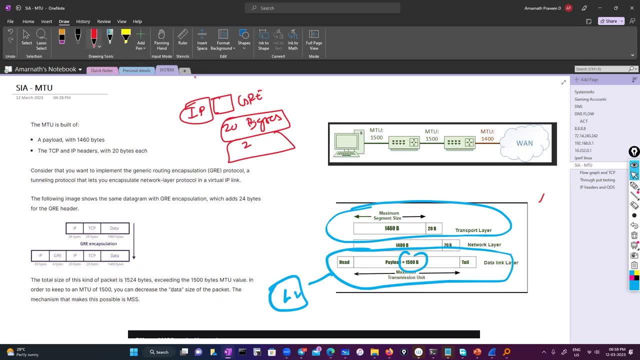 and if i add this gre header, it's a 2 and if i add this gre header, it's a 2. byte and additional information. i cannot byte and additional information. i cannot byte and additional information. i cannot exchange this data because my actual packet size will be. 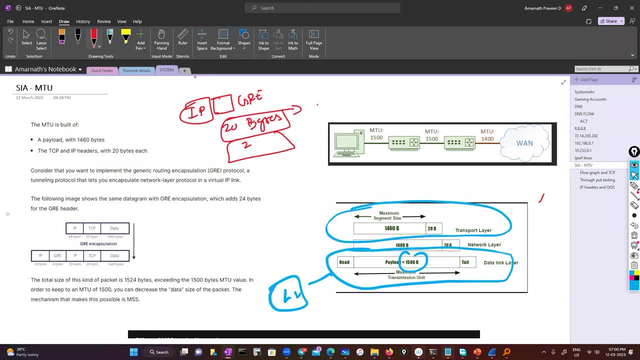 because my actual packet size will be, because my actual packet size will be incremented and it cannot be routed back incremented, and it cannot be routed back incremented, and it cannot be routed back. so what i am going to do here, so i am. so what i am going to do here, so i am. 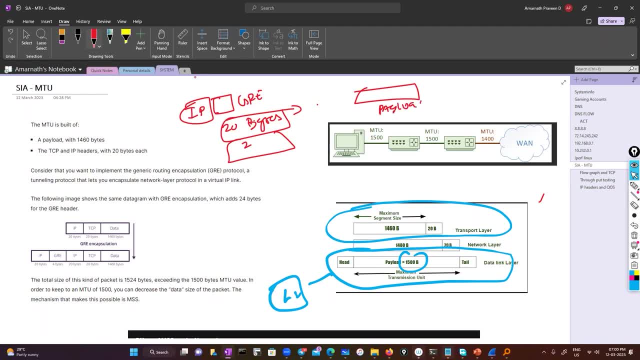 so what i am going to do here. so i am going to decrement my payload, going to decrement my payload, going to decrement my payload, how to decrement the payload. so i am giving some part of bytes to gre. so i am giving some part of bytes to gre. 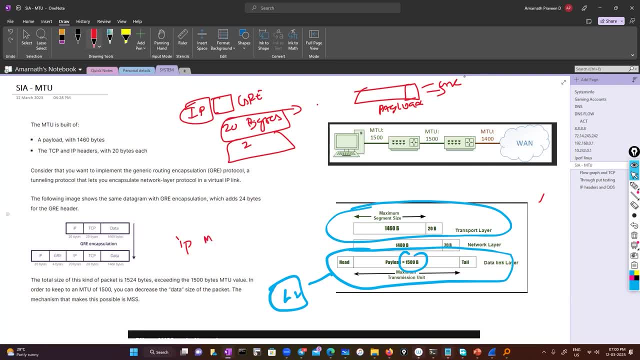 so i am giving some part of bytes to gre header. so that that's the reason you do header. so that that's the reason you do header. so that that's the reason you do this ip mss, this ip mss, this ip mss: adjust command in your router and you. 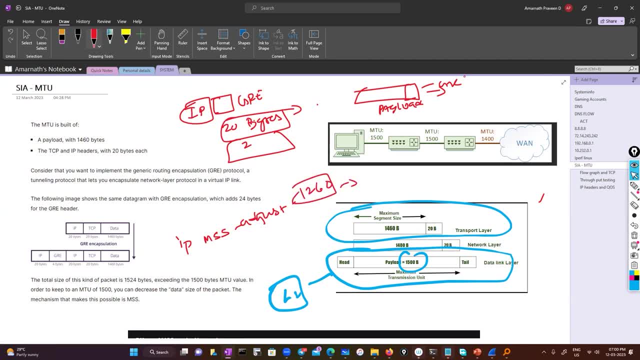 adjust command in your router and you adjust command in your router and you will decrement the value. something like will decrement the value, something like will decrement the value, something like one two six zero, one two six zero, one two six zero. so generally it will look something like: 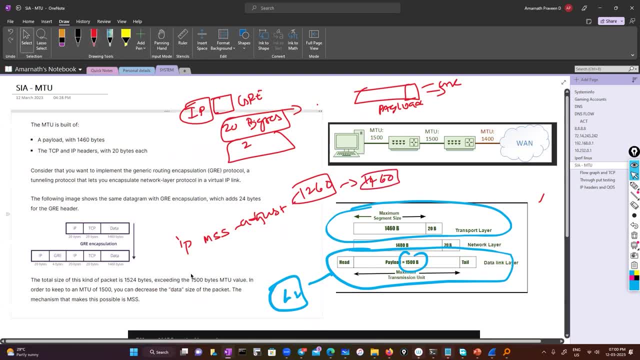 so generally it will look something like: so generally it will look something like: one four six zero t4, one four six zero t4, one four six zero t4. so if you see this particular 1500 is, so if you see this particular 1500 is, 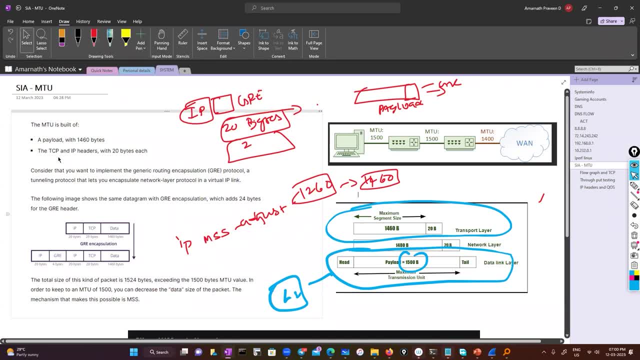 so if you see this particular 1500 is the mtu, but the maximum segment line as the mtu, but the maximum segment line as the mtu, but the maximum segment line, as i said, tcp and ip header is a 20 byte. i said tcp and ip header is a 20 byte. 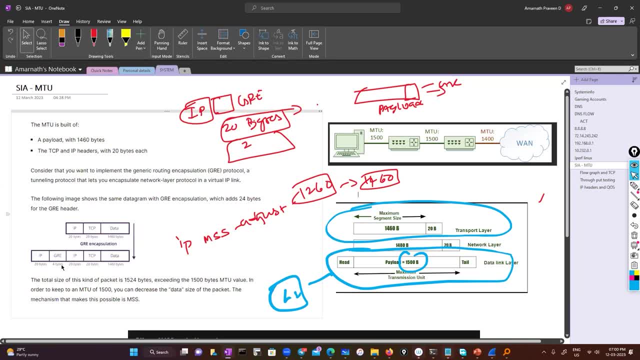 i said, tcp and ip header is a 20 byte each and you it consumes 20, 24 bytes each and you it consumes 20, 24 bytes each and you, it consumes 20, 24 bytes extra. and you, your packet cannot be extra and you, your packet cannot be. 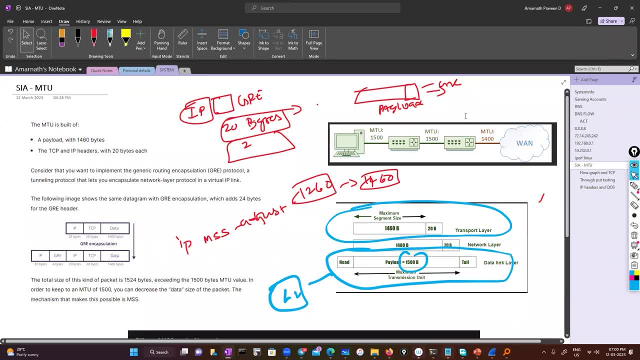 extra and you, your packet cannot be routed back. so you from your actual routed back. so you from your actual routed back. so you from your actual payload. they'll decrement this, so that's payload. they'll decrement this, so that's payload. they'll decrement this. so that's the reason. 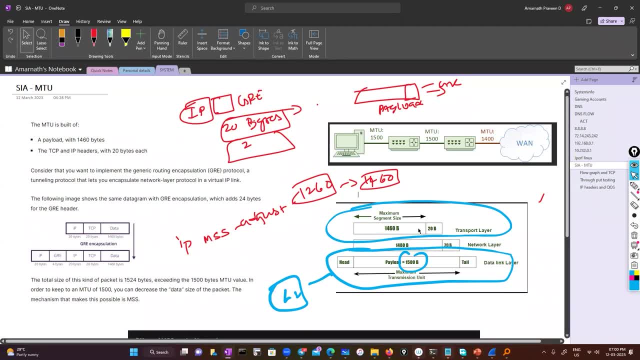 the reason, the reason the actual payloads comes here. maximum. the actual payloads comes here. maximum. the actual payloads comes here. maximum segment size, and here it they. we have to segment size, and here it they. we have to segment size, and here it they. we have to borrow some bytes. 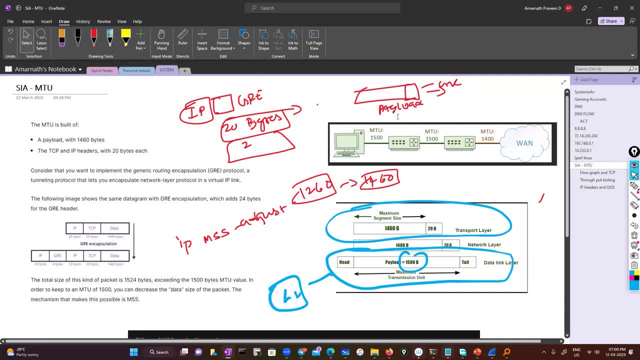 borrow some bytes. borrow some bytes. so we are freeing up some space in the. so we are freeing up some space in the. so we are freeing up some space in the segment size and you're going to route segment size and you're going to route segment size and you're going to route your traffic and 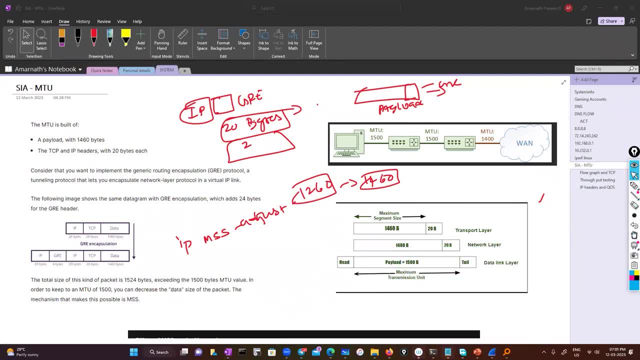 your traffic and your traffic. and now the gre package has been forwarded. now the gre package has been forwarded, now the gre package has been forwarded without any problem, without any problem, without any problem. so that is something you have to adjust. so that is something you have to adjust. 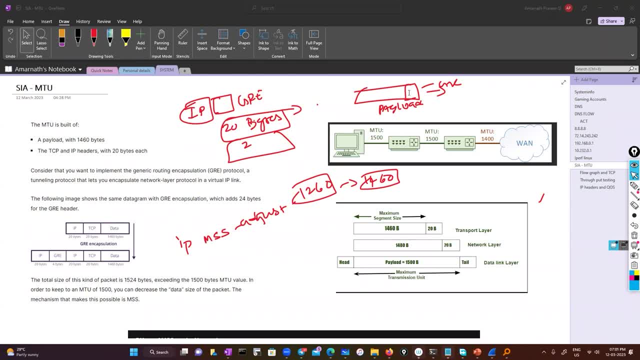 so that is something you have to adjust: your mss, your mss, your mss. segment size your payload traffic will segment size your payload traffic will segment size your payload traffic will you know that should be reduced a bit? you know that should be reduced a bit. 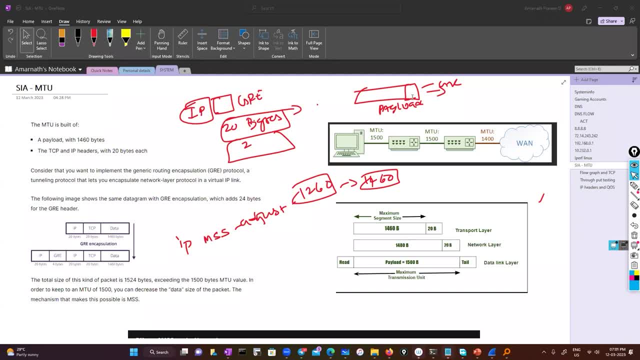 you know that should be reduced a bit from your default value, so that that from your default value, so that that from your default value, so that that particular space will be used for the particular space will be used for the particular space will be used for the gre head. 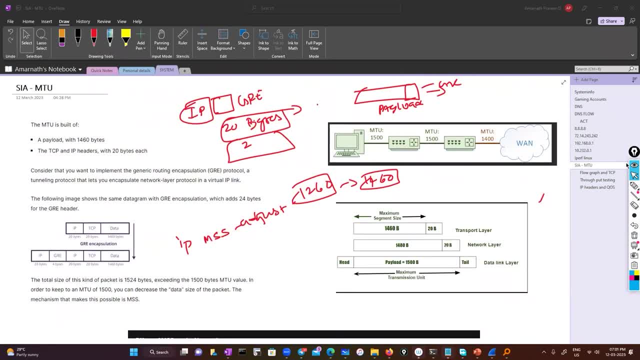 so that's it about mtu and mss. so that's it about mtu and mss. so that's it about mtu and mss. so i'm done with my presentation. so i'm done with my presentation. so i'm done with my presentation. so if you, 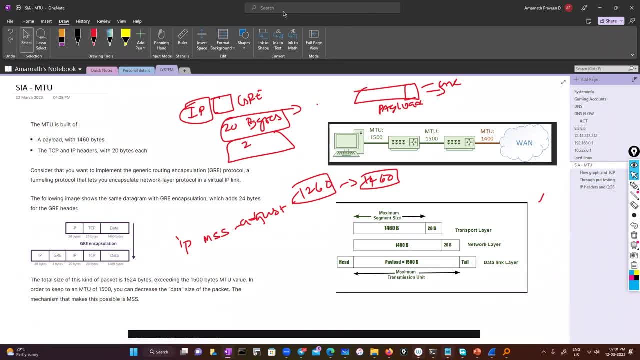 so, if you, so, if you, let me give control, let me, let me give control, let me, let me give control, let me and mute everyone. yeah, so, yeah, so, yeah. so you have a new permission, and if you have, you have a new permission. and if you have, 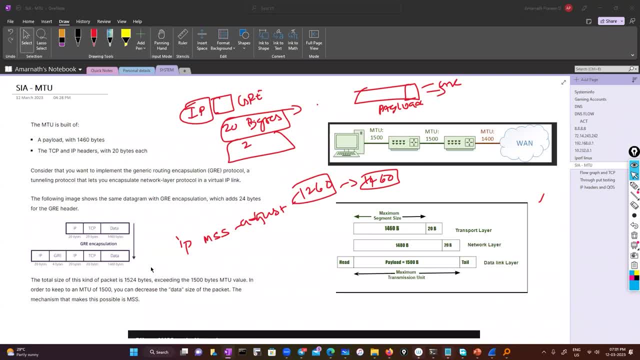 you have a new permission and if you have any questions, you can ask questions. can any questions you can ask questions? can any questions you can ask questions? can you just make me the co-host? sorry, sorry, sorry. yeah, this is him who just make me the. yeah, this is him who just make me the. 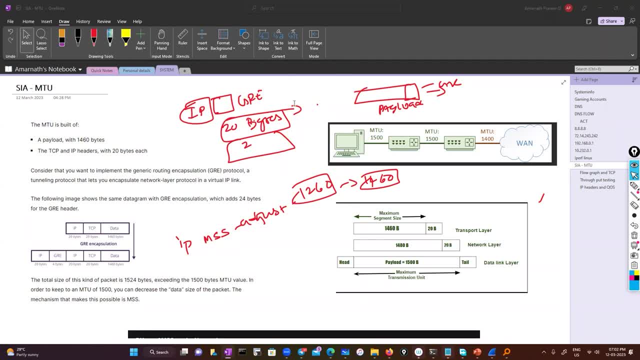 yeah, this is him who just make me the co-host, actually. uh, okay, okay. so, guys, let me tell you this particular. so guys, let me tell you this particular. so guys, let me tell you this particular y-shaped training. we are y-shaped training, we are y-shaped training. we are starting from 18th of march and it's 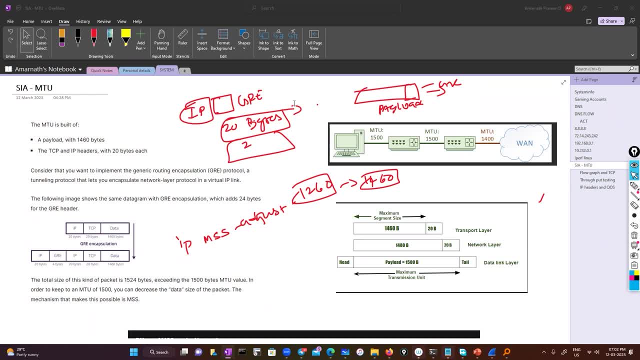 starting from 18th of march. and it's starting from 18th of march and it's like weekends batch, like weekends batch, like weekends batch, and your classes will happen starting from, and your classes will happen starting from, and your classes will happen starting from 11 am to 1 pm ist. 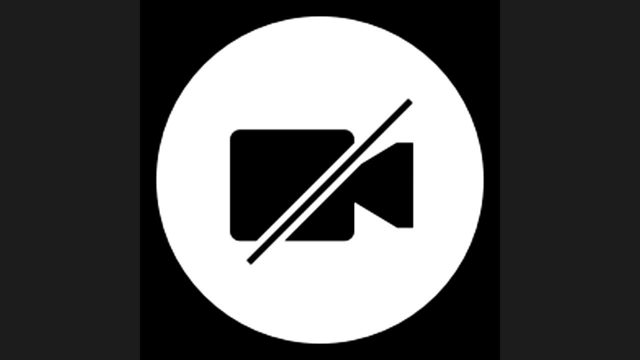 the fees for this training is seven. the fees for this training is seven. the fees for this training is seven thousand, sorry, five thousand. and what's about duration? and what's about duration, and what's about duration. so, can you arjun, can you just take this? so, can you arjun, can you just take this? 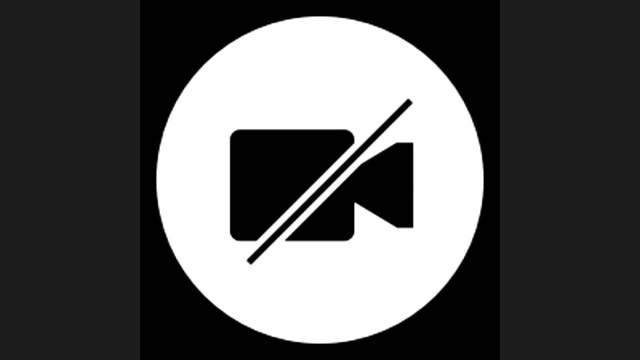 so can you, arjun, can you just take this question? how much, yeah? yeah, it's a 45 question. how much, yeah? yeah, it's a 45 question. how much, yeah? yeah, it's a 45 house maximum, house maximum, house maximum. it will go around 45 hours, yeah, yeah. 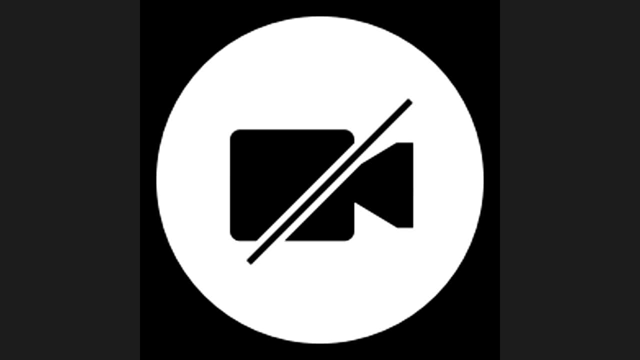 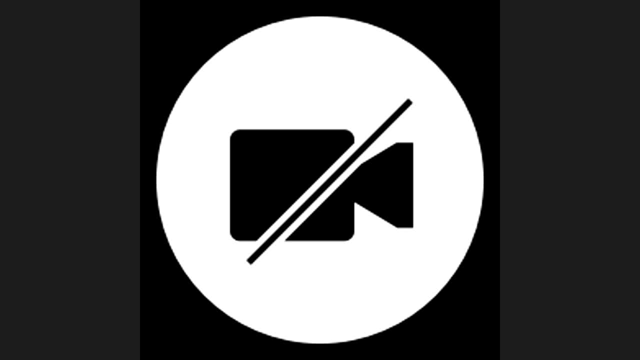 sir, yes, training sir, sir, yes, training, sir, sir, yes, training sir. not possible, not possible. not possible, sir, because, uh, we are five hours ahead, sir, because, uh, we are five hours ahead. not possible, sir, because, uh, we are five hours ahead, not to early morning. i mean, the course is very. 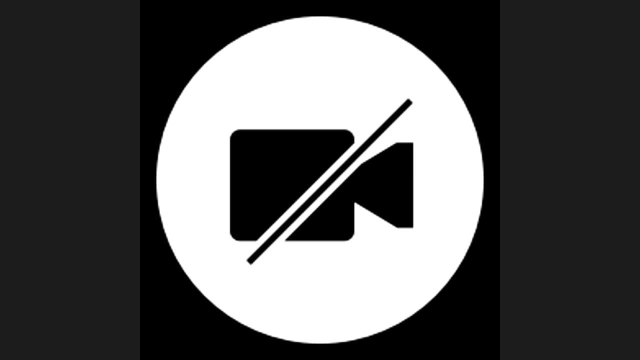 early morning. i mean the course is very early morning. i mean the course is very good. i've i've gone through the content, good, i've i've gone through the content. good, i've i've gone through the content as to it's. it's very good and the 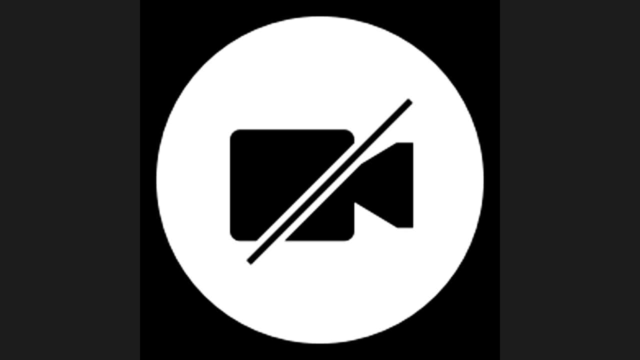 as to it's it's very good and the as to it's it's very good and the piece is also very. piece is also very, piece is also very. please, please, please. let's see, we will discuss internally. let's see, we will discuss internally. let's see, we will discuss internally and we will let you know on that. 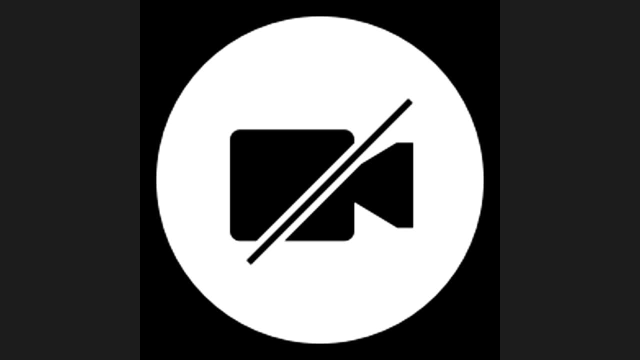 and we will let you know on that. and we will let you know on that. okay, you can reach out to me directly. okay, you can reach out to me directly. okay, you can reach out to me directly. no worries, sir, thank you. thank you, yeah, guys, if you have any questions, uh. 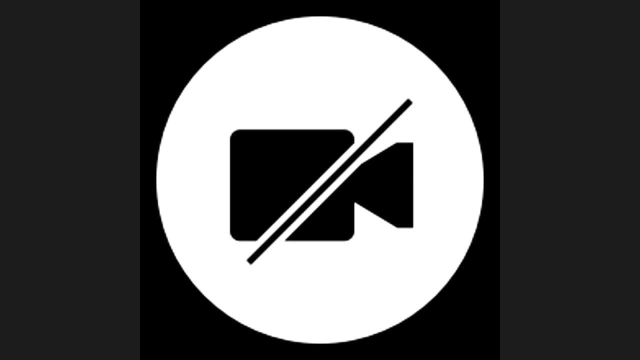 yeah, guys, if you have any questions. uh, yeah, guys, if you have any questions, uh, you can ask your questions, sir. one more, one more question about the sir. one more, one more question about the sir. one more, one more question about the. the troubleshooting part, sir. the troubleshooting part, sir. 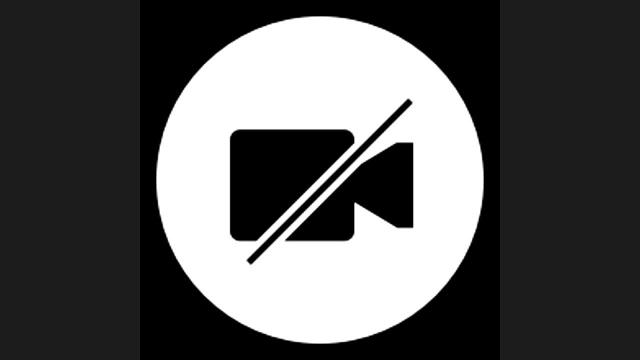 the troubleshooting part, sir. troubleshooting, troubleshooting, troubleshooting, troubleshooting, wireshark, wireshark, wireshark. sir, about this sir, will there be any real sir about this sir? will there be any real sir about this sir? will there be any real scenarios like, say, for example, if we 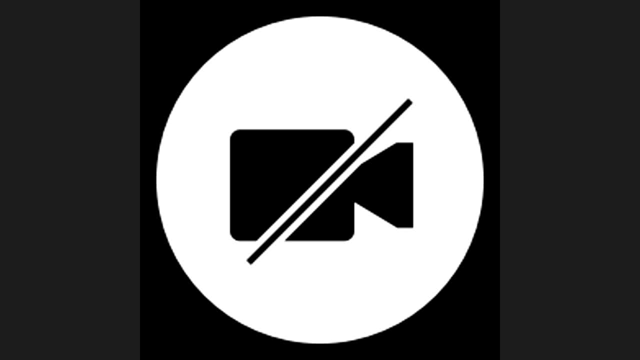 scenarios like say, for example: if we scenarios like say, for example, if we find a problem at work, find a problem at work, find a problem at work where there is like a slowness, or where there is like a slowness or where there is like a slowness or somebody is complaining that we cannot. 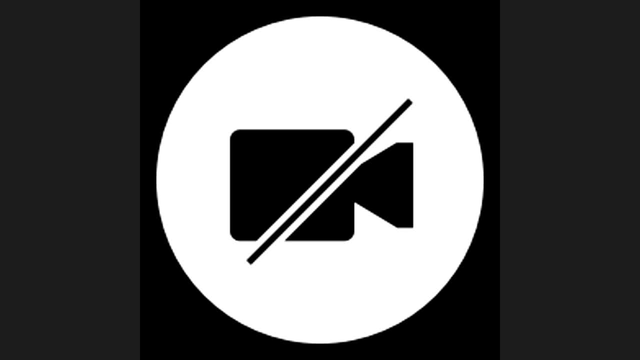 somebody is complaining that we cannot. somebody is complaining that we cannot access xyz server. access xyz server. access xyz server. or there is a delay or something like. or there is a delay or something like. or there is a delay or something like that. so, sir, that so sir. 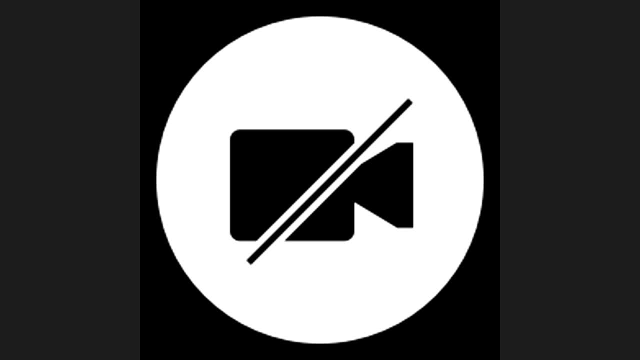 that. so, sir, would we have like some sort of you know? would we have like some sort of you know? would we have like some sort of you know? you mean to say you, you know you mean to say you, you know you mean to say you, you know. that's something different. i didn't get. 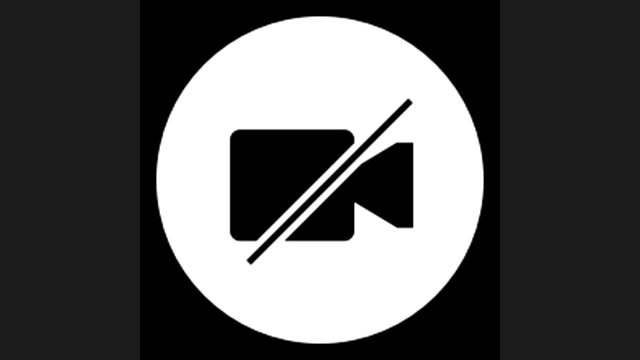 that's something different. i didn't get. that's something different. i didn't get your question, something you you mean to your question, something you you mean to your question, something you you mean to say we have to replicate a problem and say we have to replicate a problem and 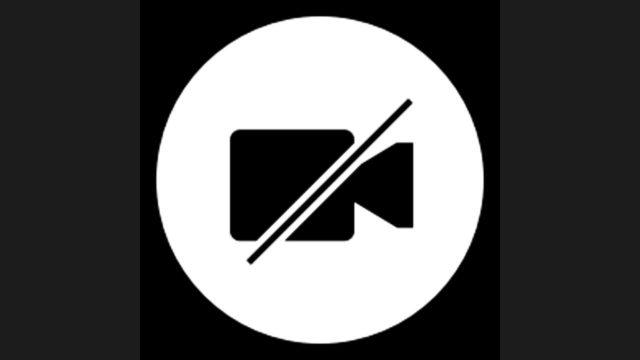 say, we have to replicate a problem and do a capture, do a capture, do a capture and uh do an analysis. so that helps you and uh do an analysis so that helps you and uh do an analysis. so that helps you to figure out exactly where the problem. 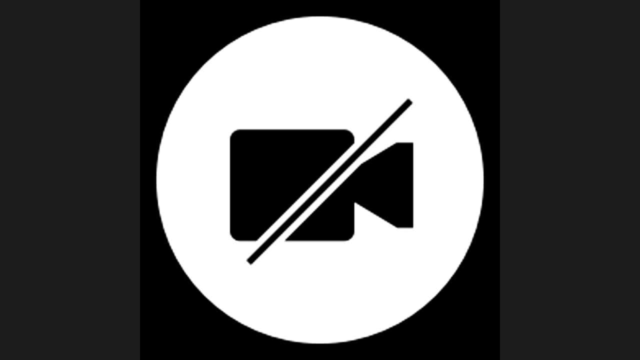 to figure out exactly where the problem. to figure out exactly where the problem is is is, sir, exactly, i can give you examples. say, sir, exactly, i can give you examples. say, sir, exactly, i can give you examples. say, for example, i have a problem at work. for example, i have a problem at work. 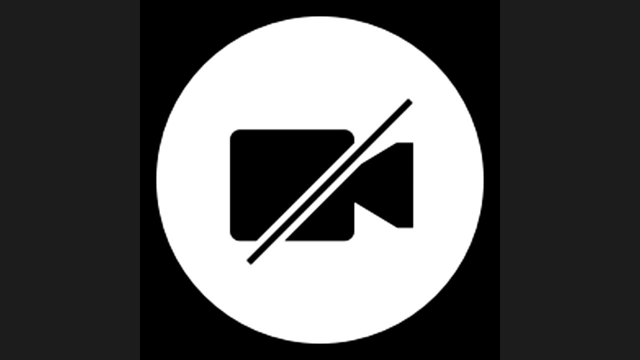 for example, i have a problem at work. same like you discussed that same. like you discussed that same. like you discussed that there was, you know, like a throughput there was. you know like a throughput there was, you know like a throughput issue or something like that. so would 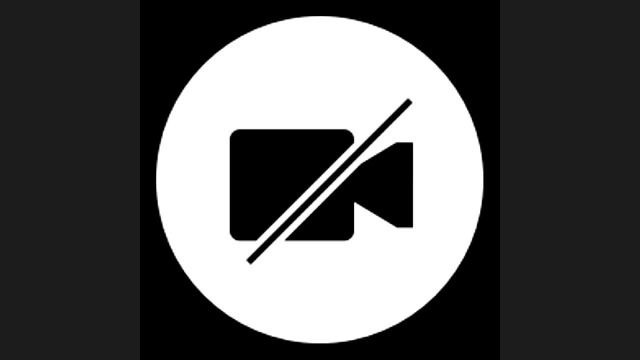 issue or something like that. so would issue or something like that, so would there be like any more scenarios that we there be, like any more scenarios that we there be, like any more scenarios that we can look into and you know compare it. can look into and you know compare it. 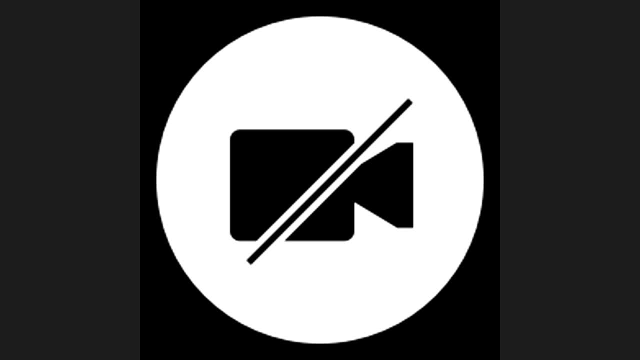 can look into and you know compare it: what we have, what we have, what we have, and you know, give them some suggestions and you know give them some suggestions and you know give them some suggestions. yeah, of course you have to take a. yeah, of course you have to take a. 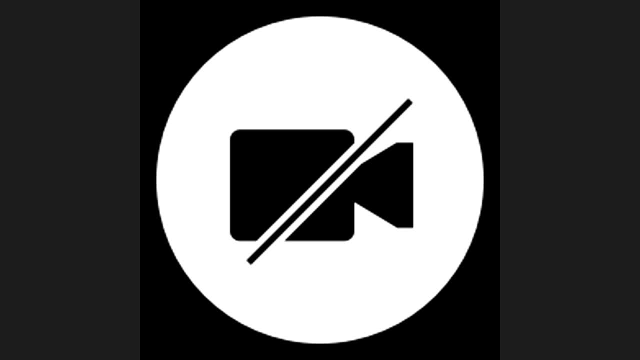 yeah, of course you have to take a capture. it depends on your device. i mean capture, it depends on your device. i mean capture, it depends on your device. i mean you can take pcp down power if it is a. you can take pcp down power if it is a. 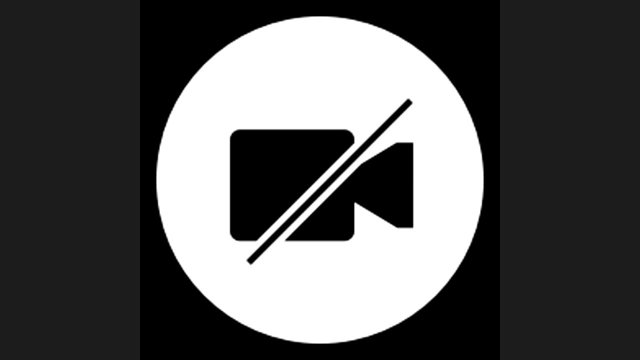 you can take pcp down power if it is a cisco boxes. you have, you know, inbuilt cisco boxes. you have, you know, inbuilt cisco boxes. you have, you know, inbuilt embedded packet capture functionality. embedded packet capture functionality. embedded packet capture functionality. that is, you know you can make use of uh. 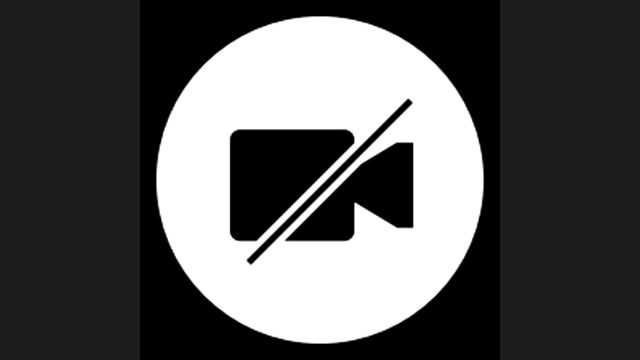 that is, you know you can make use of uh. that is, you know you can make use of uh- your device and you can take a tcp down your device. and you can take a tcp down your device and you can take a tcp down and you can offload the pcaf file to. 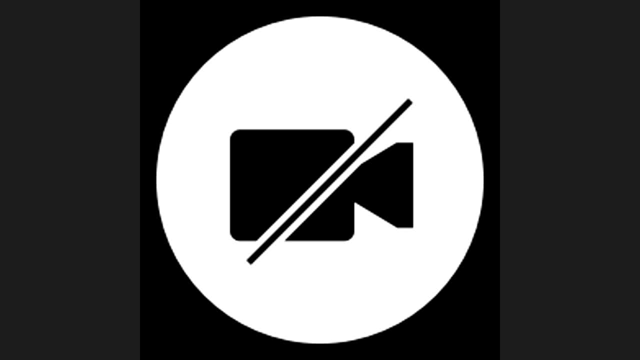 and you can offload the pcaf file to. and you can offload the pcaf file to your local pcrt. you know your tftp, your local pcrt. you know your tftp, your local pcrt. you know your tftp somewhere. and if you have your pcaf, 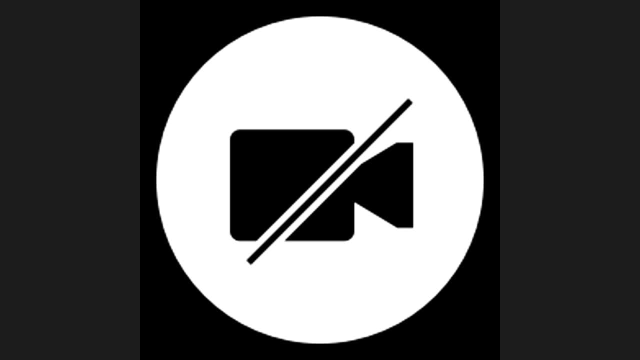 somewhere and if you have your pcaf somewhere and if you have your pcaf file, then yeah, definitely, we can look file. then yeah, definitely, we can look file. then yeah, definitely, we can look into it and we can figure out what would into it and we can figure out what would. 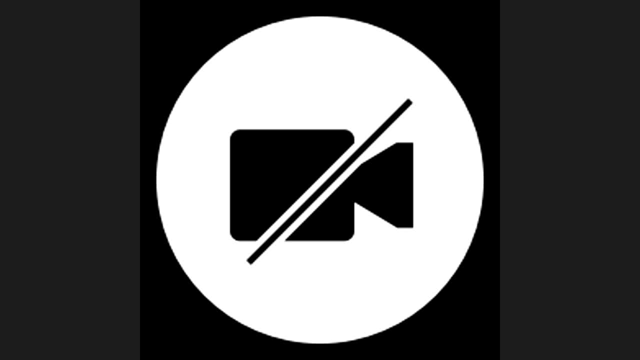 into it and we can figure out what would be the problem there be the problem there. be the problem there. okay, okay, okay, thank you no problem. okay, okay, thank you, no problem, okay, okay, thank you, no problem. yeah, uh, hi arjun, this is shoye. yeah, uh, hi arjun, this is shoye. 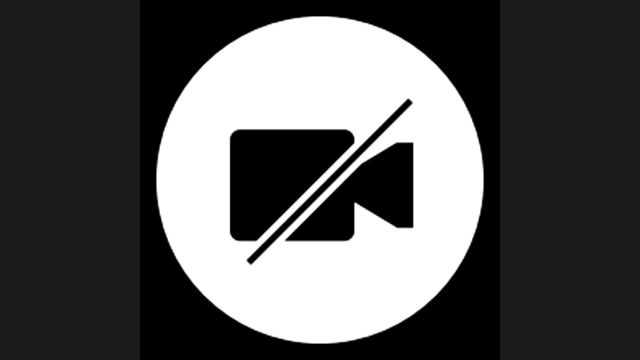 yeah, uh, hi arjun, this is shoye. i show you, uh, i think the session was uh. i show you, uh, i think the session was uh. i show you, uh, i think the session was uh. first of all, i would like to. first of all, i would like to. 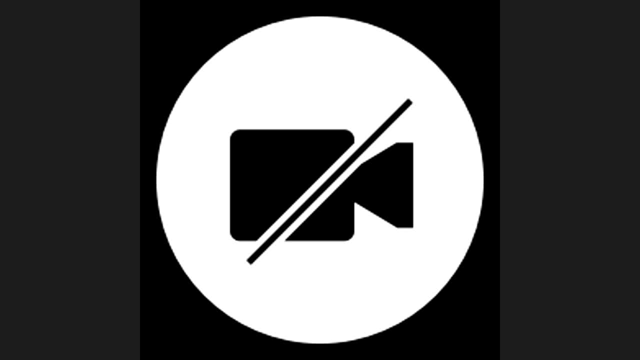 first of all, i would like to congratulate that the session was good, congratulate that the session was good, congratulate that the session was good. so, like uh, you mentioned about the. so, like uh, you mentioned about the. so, like uh, you mentioned about the throughput issue from your pc, that it. 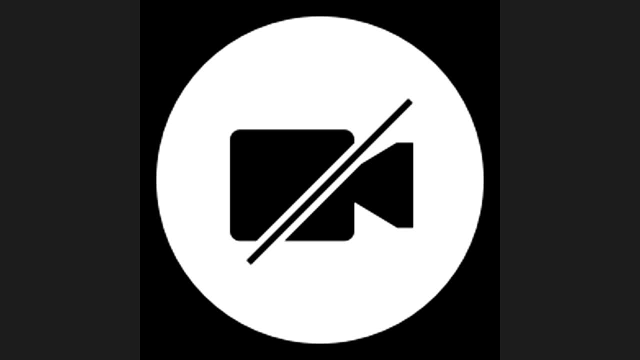 throughput issue from your pc that it throughput issue from your pc that it was not able to, was not able to, was not able to. uh receive the packet. uh send the packet. uh receive the packet. uh send the packet. uh receive the packet. uh send the packet again because it has this: 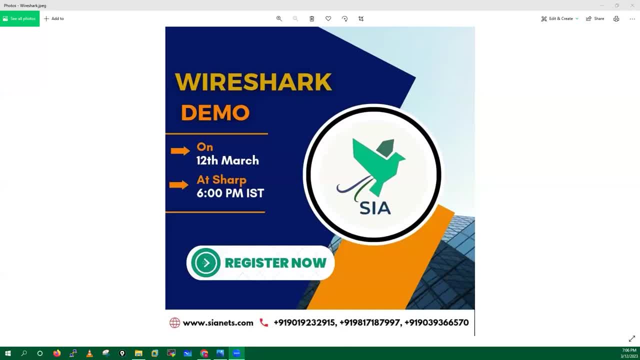 again because it has this again, because it has this capacity pool, okay, so probably it was capacity pool. okay, so probably it was capacity pool. okay, so probably it was due to the due to the due to the throughput issue, so similar issue i am. throughput issue, so similar issue i am. 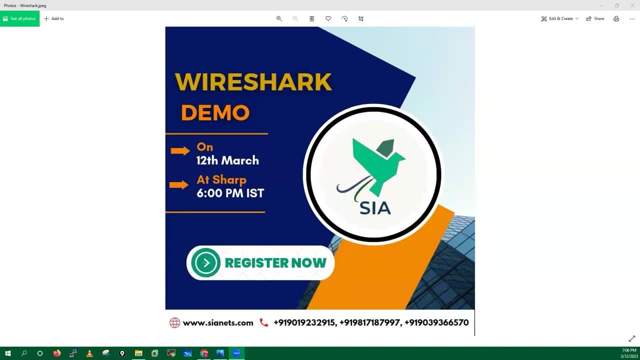 throughput issue. so similar issue i am having in a production environment: where having in a production environment? where having in a production environment where the end user is your android apk, the end user is your android apk, the end user is your android apk, okay, and there are multiple uh. 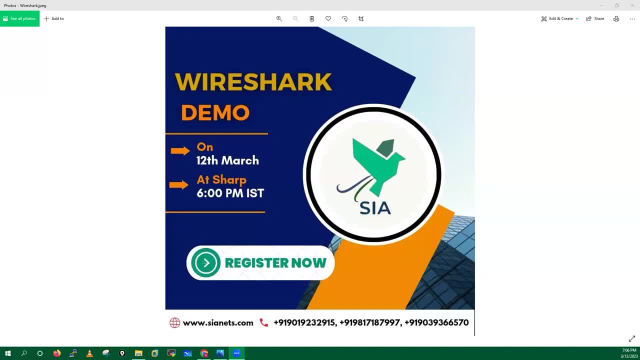 okay, and there are multiple uh okay, and there are multiple uh. retransmission is being retransmission is being retransmission is being uh sent from the source to the uh. sent from the source to the uh. sent from the source to the means, from the. 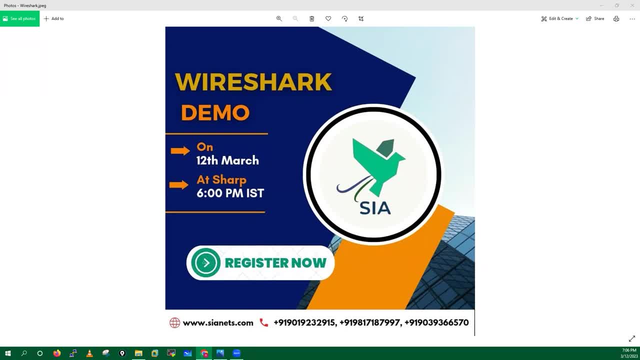 means, from the means, from the android apk device to android apk device to android apk device, to the destination which is behind the f5, the destination which is behind the f5, the destination which is behind the f5, firewall, firewall, firewall. okay, so what would be the possible? 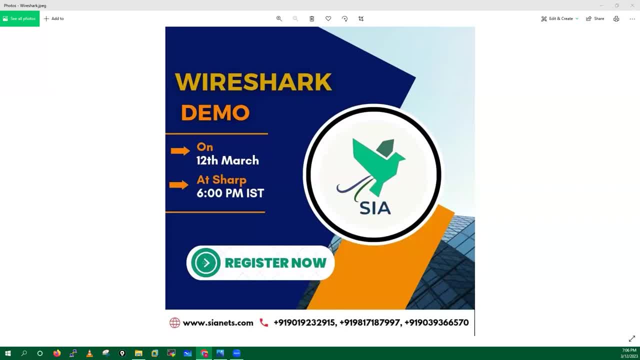 okay, so what would be the possible? okay, so what would be the possible reason? i have that uh reason. i have that uh reason. i have that uh captures with me. if you can uh captures with me, if you can uh captures with me, if you can uh, if you allow me to share, then i can i. 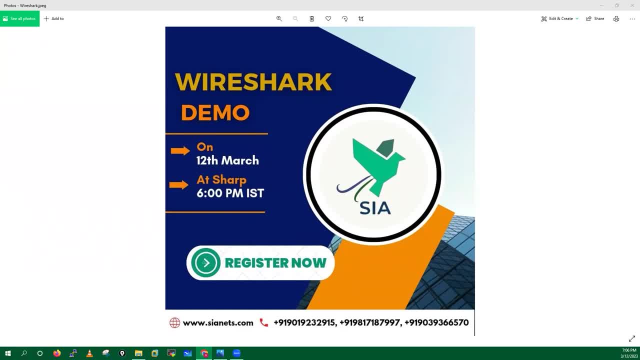 if you allow me to share, then i can i. if you allow me to share, then i can. i can share those, can share those, can share those. no, no in the in the real classes. we can no. no, in the in the real classes. we can no. no, in the in the real classes, we can do it. but since this is a demo, one that 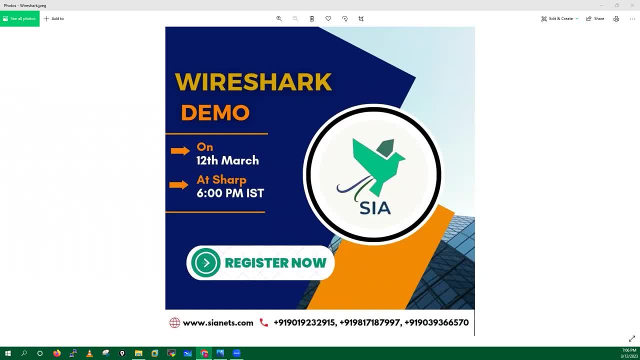 do it. but since this is a demo one, that do it. but since this is a demo one that is strictly, is strictly, is strictly confidential, then fine, then fine, then fine, yeah, no problem. yeah, hello, hello, yeah, no problem. yeah, hello, hello, yeah, no problem. yeah, hello, hello yeah. 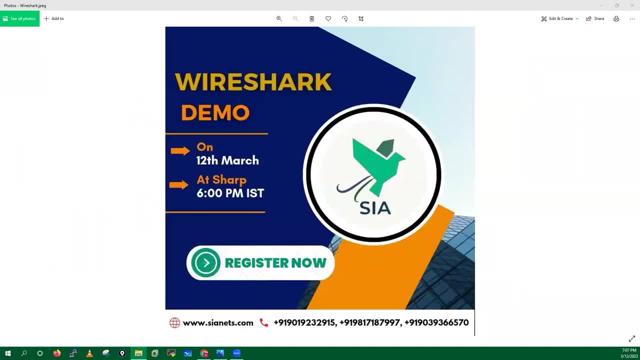 yeah, no problem, yeah, hello, yeah, yeah, no problem, yeah, hello, yeah. sir manish decided actually, sir uh, i want, sir manish decided actually, sir uh, i want. sir manish decided actually, sir uh, i want to ask uh means rather than uh wire, to ask uh means rather than uh wire. 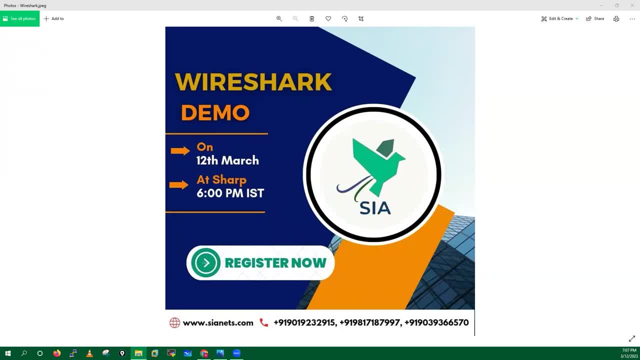 to ask: uh means, rather than uh wire, serving actually one interview question, serving actually one interview question, serving actually one interview question. i want to discuss with you. is it okay, sir? i want to discuss with you. is it okay, sir? i want to discuss with you, is it okay, sir? means: yeah, yeah, yeah, yeah, yeah, yeah. 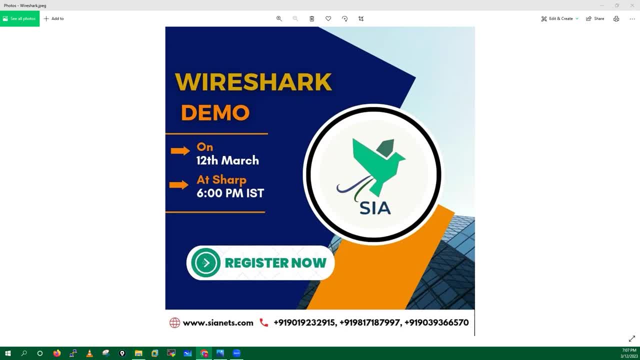 means yeah, yeah, yeah, yeah, yeah, yeah means yeah, yeah, yeah, yeah, yeah, yeah, yeah, okay uh. last uh means two days ago. i okay uh. last uh means two days ago. i okay uh. last uh means two days ago. i had an interview with the tcs, so they 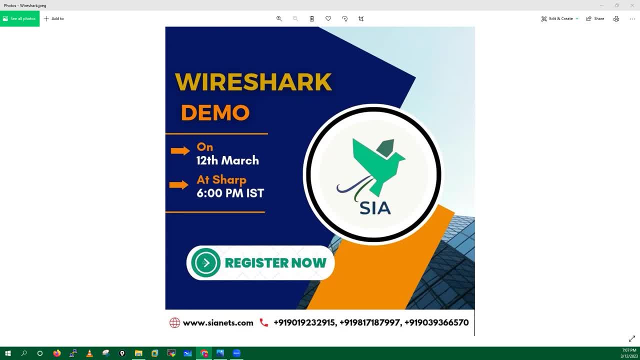 had an interview with the tcs. so they had an interview with the tcs. so they asked me about the. uh means uh. if uh asked me about the, uh means uh. if uh asked me about the, uh means uh. if uh uh william. if they asked me about the, 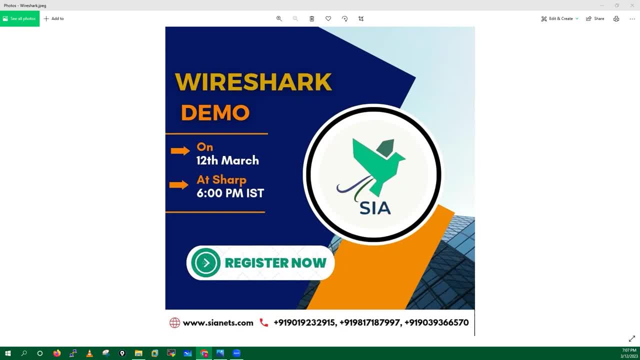 uh william if they asked me about the. uh william if they asked me about the dhcp server. okay, dhcp server is not in dhcp server. okay, dhcp server is not in dhcp server. okay, dhcp server is not in our vlan. so what is the this scenario? our vlan? so what is the this scenario? 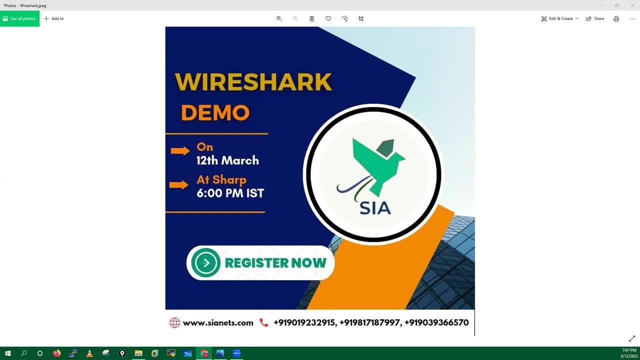 our vlan. so what is the this scenario means means means the client and server of the different, the client and server of the different, the client and server of the different vlan segments can communicate. so means vlan segments can communicate. so means vlan segments can communicate. so means so i at that time i had no idea about. 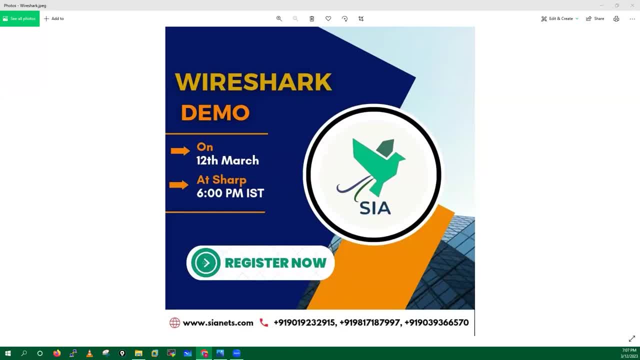 so i at that time i had no idea about. so i at that time i had no idea about the dhcp relays and how to work the dhcp relays and how to work the dhcp relays and how to work. please could you explain me in means in: 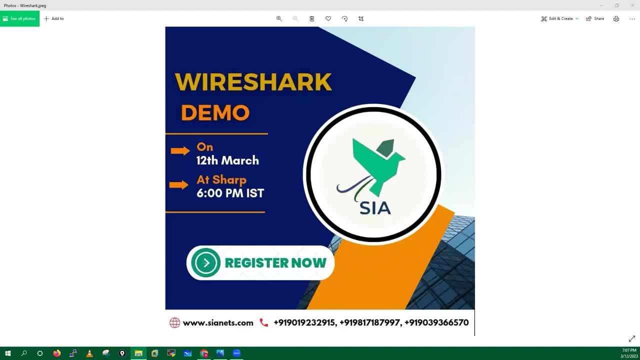 please could you explain me in means in. please could you explain me in means, in overview means. overview means, overview means a dhcp related how it works, and so a dhcp related how it works, and so a dhcp related how it works, and so what is the scenario? what is the scenario? 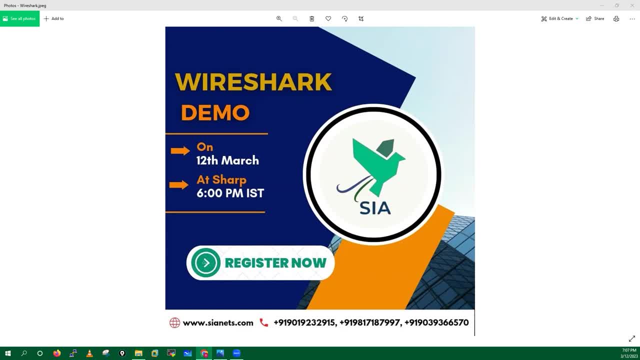 what is the scenario? yeah sure uh so example. so yeah sure uh so example. so yeah sure uh so example. so generally, generally, generally, yeah, yeah, yeah, in the enterprise right, so in the. in the enterprise right so in the. in the enterprise right, so in the enterprise people, you know what they do. 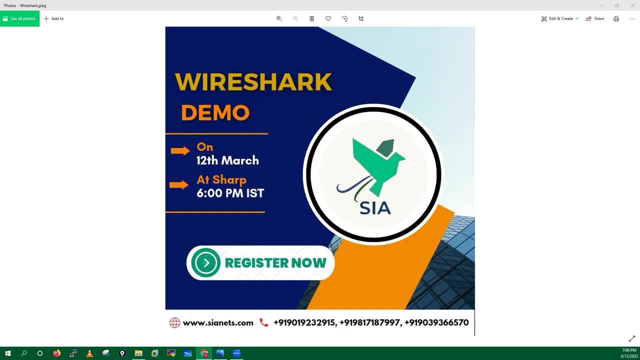 in the enterprise people. you know what they do in the enterprise people. you know what they do generally, if generally, if generally. if this is your switch and they say dhcp, this is your switch and they say dhcp, this is your switch and they say dhcp- relay agent, you have some. 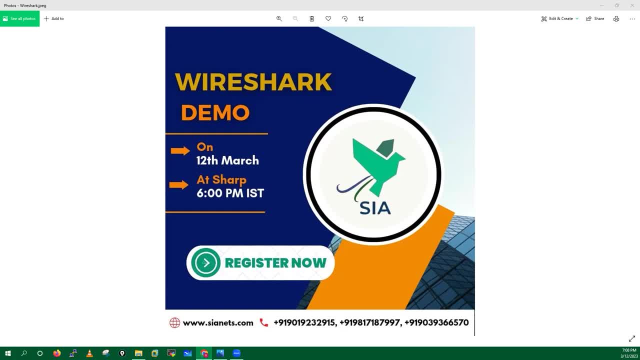 relay agent. you have some relay agent. you have some uh. you know you have a fair idea about uh. you know you have a fair idea about uh. you know you have a fair idea about how this uh dhcp relay agent works, how this uh dhcp relay agent works. 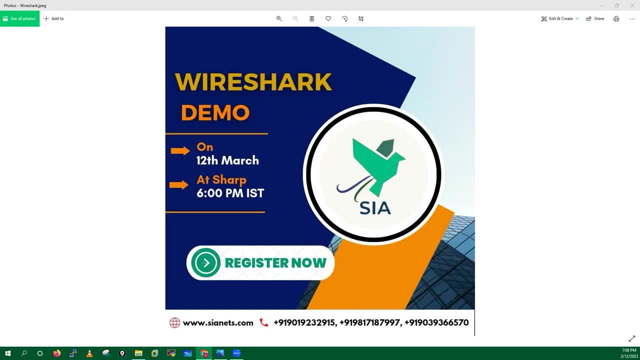 how this uh dhcp relay agent works right. so example: this is your right. so example: this is your right. so example: this is your dhcp relay agent and the ideology is dhcp relay agent and the ideology is dhcp relay agent and the ideology is something you might have one common: dhcp. 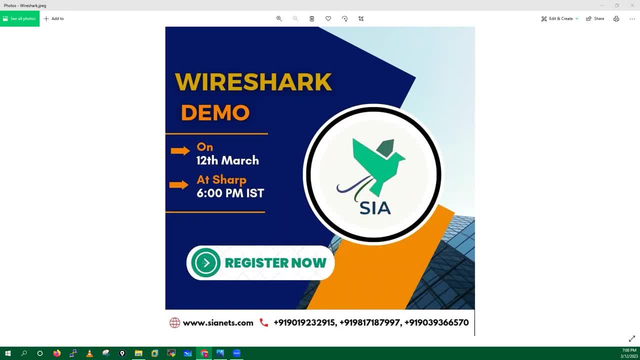 something you might have: one common dhcp server. so that is ideology for every server. so that is ideology for every server, so that is ideology for every vlan for every network and for every vlan for every network and for every vlan for every network and for every site. to have a dhcp server is not a good. site. to have a dhcp server is not a good site. to have a dhcp server is not a good practice. i mean i'm not saying it's a practice. i mean i'm not saying it's a practice. i mean i'm not saying it's a good practice, it's for. from the good practice it's for. from the good practice it's for. from the administration standpoint it's very hard administration standpoint. it's very hard administration standpoint. it's very hard to have multiple dhcp servers. when there to have multiple dhcp servers. when there to have multiple dhcp servers when there is a problem, there is something like one. 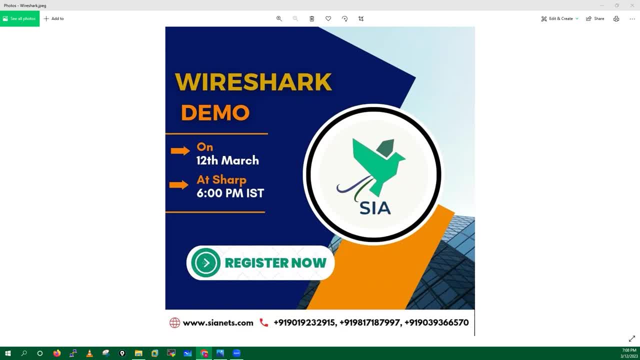 is a problem. there is something like one is a problem. there is something like one common, common, common dhcp server for the management dhcp server, for the management dhcp server, for the management perspective. it's pretty simple to manage perspective. it's pretty simple to manage perspective. it's pretty simple to manage in troubleshoot. so 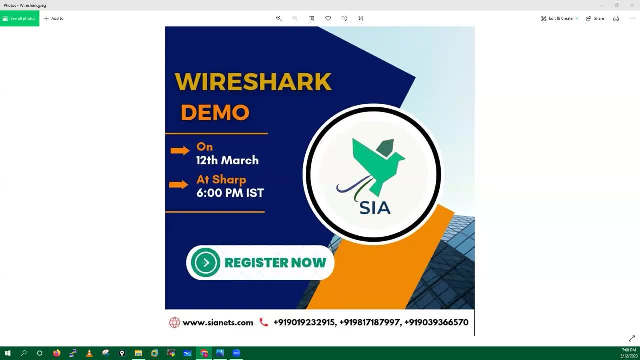 in troubleshoot, so in troubleshoot. so here you got your pc example. your pc is here. you got your pc example. your pc is here. you got your pc example. your pc is on 10 network, on 10 network, on 10 network, right, right, right. so what exactly happens? you know dhcp. 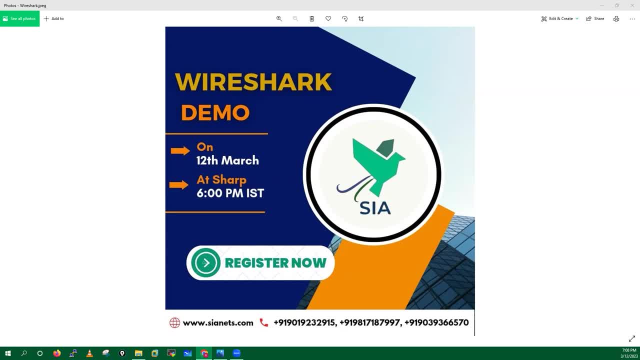 so what exactly happens? you know dhcp. so what exactly happens? you know dhcp is a broadcast. are you aware of it? so dhcp packet is a broadcast. so inside the local land, that's something inside the this particular network. if it is a 10 network, it's going to broadcast to all the ips, right, looking for the 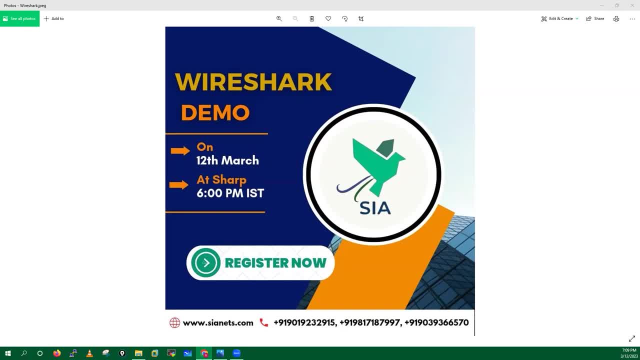 dhcp response. but since i got the dhcp relay agent somewhere here in the data center that that can be in any subnet example- here let it be 15001 example- this is your dhcp relay agent. so if this, for this particular broadcast, it hits your gateway for sure, right, because it will send to every pc. that's a. 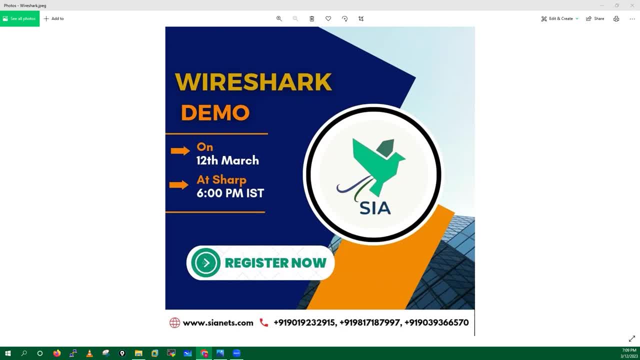 broadcast. so when we get this broadcast packet, so inside this you you configured your dhcp relay server. your relay server is configured and you have given the ip address. something like 15001 is my relay server. so what happens from the pc to the gateway? it is a broadcast, yes, but whereas from the gateway to 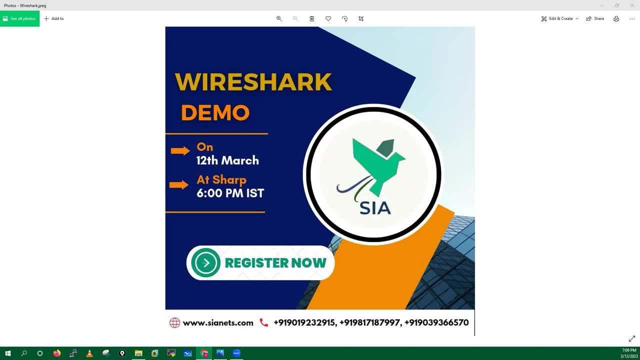 the dhcp relay agent is a unicast. so here in the unicast, what is the information it's going to send? it's going to send this gateway address. what is this gateway address? so i, this is my gateway address, 1001. so what happens when it goes to the dhcp server? it got multiple pools and it's going. 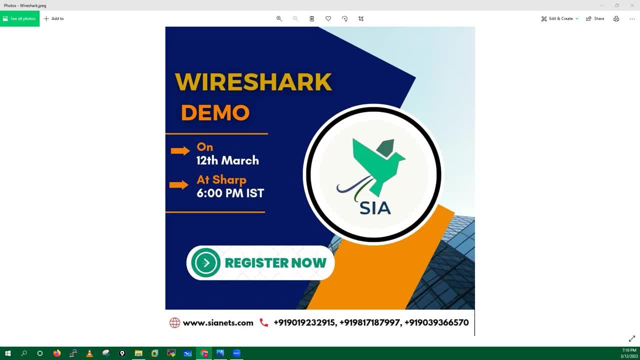 to look for this particular pool. if there is a match, it's going to look into the scope. okay, i got an ip range from 1002 to 100254, so i got this many ips and it will replay back again to this gateway and this gateway again. it will replay back to the pc. 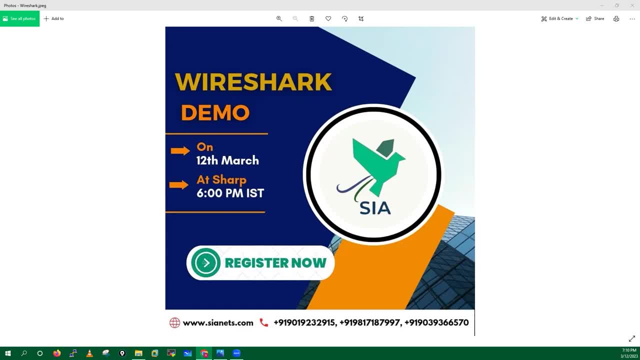 it says: hey, here you got your for your dhcp request i am going to offer this packet offer is just kind of uh, you know, uh it going to say: hey, this is the ip address if you want you can use. okay, until this is no commitment that i am going to use the same ip address but for this dhcp request it's going to. 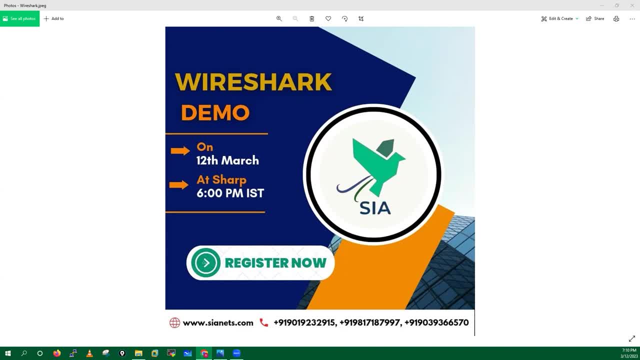 send a dhcp reply back. that is offer. yeah, yeah, so that means uh, inside, means outside the vlan. it goes as a dhcp relay, as it means if it is server, isn't if it's in different vlan. so then yeah, so if my, my pc is in uh 10.0 network, the network will be there, okay, and and the server is. 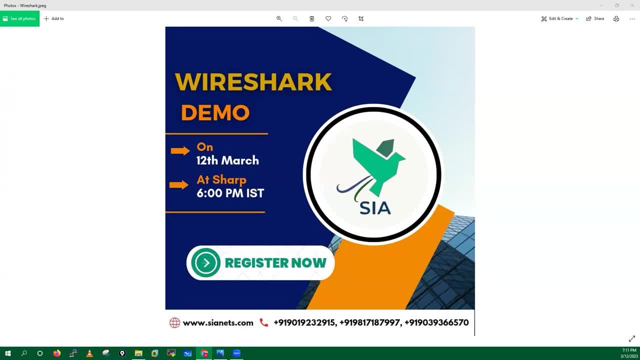 it will get to the uh gateway of the 10.0. suppose it is 10.1 and and from the 10.1 it will, it will unicast the dhcp agent till the server. is it means it is? is that the flow means? no, no, no, flow is. 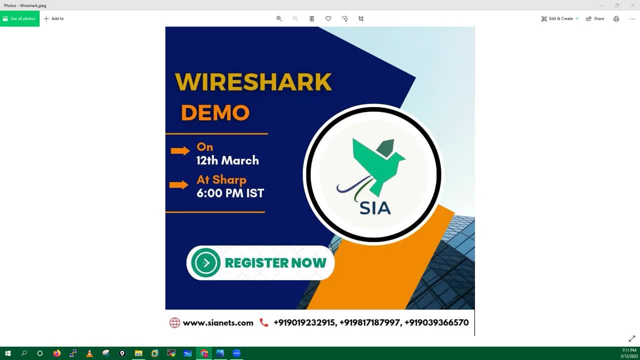 something. it is from the gateway to the dhcp server. it's it's a point-to-point connection. it's an unicast right. it's straight away to your dhcp server because you defined your ip details there in the dhcp relay. so it's a unicast server. it's a unicast server, so it's a unicast server. 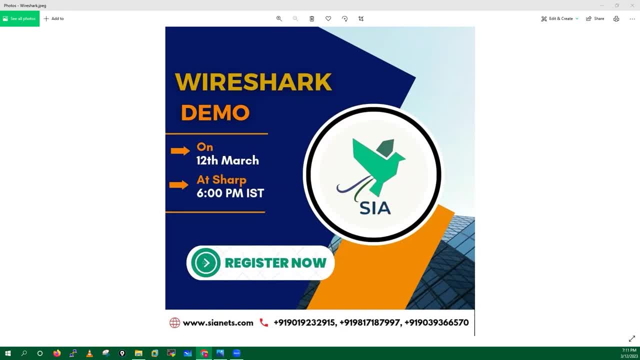 so you have to understand one thing: see here: if your routing is fine, you have to check first: you have a reachability to your dhcp server? yes, then your routing is fine, then happens the unicast. the first overlay is your routing and then on top of that it's. 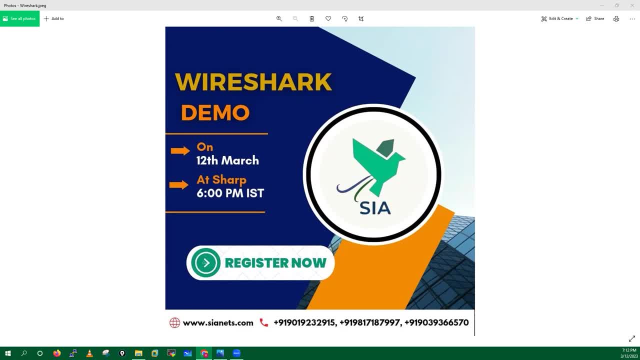 it's an, you know, your underlay is your routing. if you're writing, routing is: uh, you know, if your routing is properly happening and you can reach the destination, then comes this unicast in forwarding. yeah, okay, simply you can just say like this: if your your dhcp server is somewhere in the data center, which 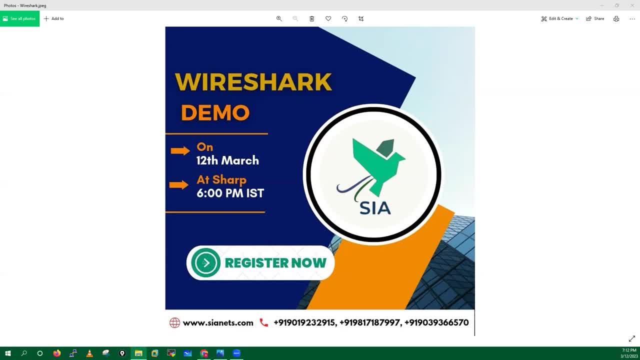 is not in the same network and you you want to get the ip, because in order to get this uh to the client, get to the ip address, they need to communicate with the dcp. yes, you're right, the communication will be there, but only the simple thing if. 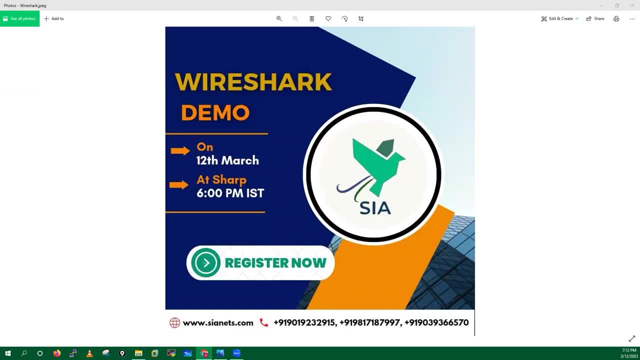 if the dhcp ip helper command needs where you, your uh client is not in the same network, that's. that's that, because uh dhcp is a layer two, isn't it? so it's not, it will broadcast but it will not go after, because if it's not in the same network, i suppose if your dhcp server sit in the 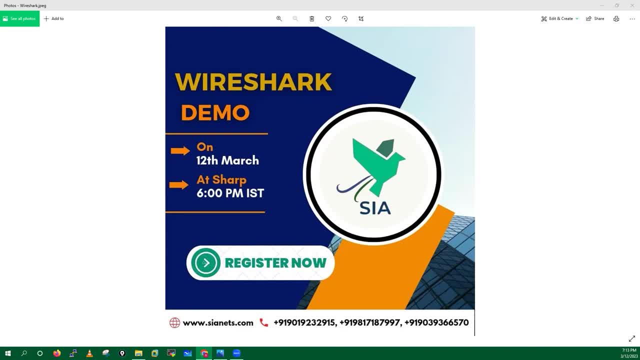 somewhere in the data center and you want to get connection, your client get to connection to the dhcp. yes, you need ips. yes, you need ips helper command. that's the only simple thing, isn't it? yeah, yes, hello guys. so anyone have anything else? otherwise, we can just yeah. 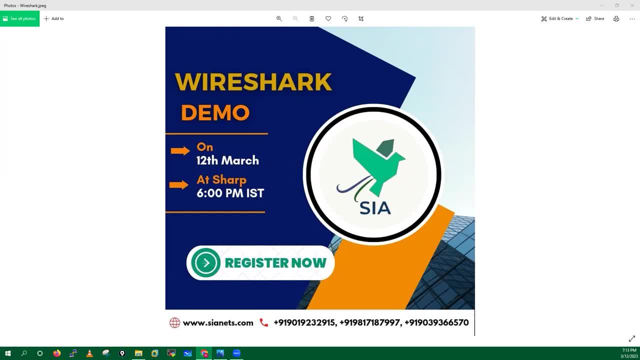 hi arjun people here this side. so first of all, thanks for uh. your session will help. if someone is planning for wcna. it will be helpful for him. uh, what is the wcna? can you, uh, i know, can you abbreviate what is wc? yeah, yeah, that is the. or certified network analyst. 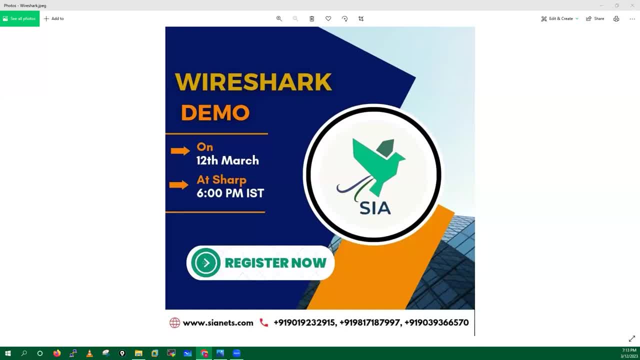 yeah, so definitely this, this particular course, will help you for that, but, like i will not recommend you can go for this particular certification because it's not needed, right? yeah, that is my next, if you are working as a, like, network security engineer or as a network engineer. 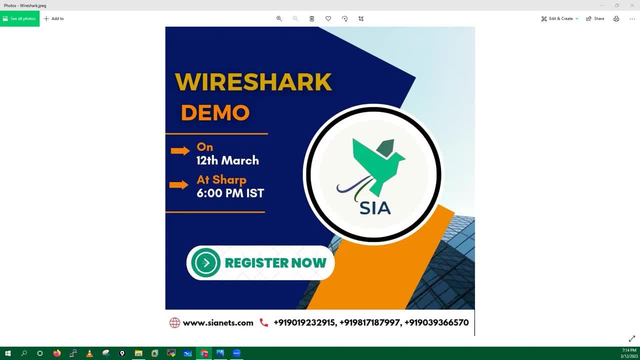 not needed at all, actually. okay, that's right. yeah, okay, i didn't. um, i just have a question like uh uh, since, uh, you know i'm into the security side. uh, so what are the things that you are going to cover when it comes to security part? 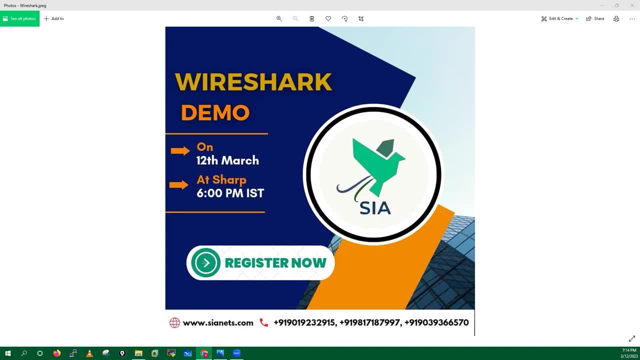 we discuss about tls and various authentication mechanism. how are you working on tacx? so we'll try to you know, find what is why this is talking about this topic, the. in the course content you will see all the security protocols: what, what? what are the security protocols we discussed here? yeah, any malware content or something that you can cover, at least. 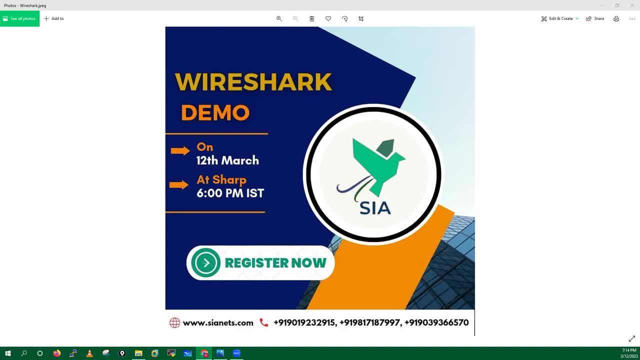 some basics. ddos attack: we have an over topic to discuss about ddos attack and how to prevent it and how the ysh can be configured to find the geo locations where you can find where exactly your traffic is coming from. sure, sure, okay, thank you, ajit. yeah, no problem, any other questions guys? 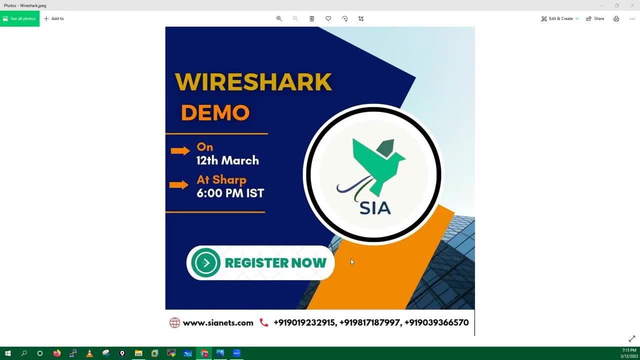 anyone have? it's like somebody interested for this particular training and if somebody wants to enroll, these are the mentioned contact numbers. you have to reach out to us on these particular numbers. okay, anyone have anything? yeah, it's, timings are fixed, because i actually timing is actually. yeah, timing is fixed, okay. 11 am to 1 pm: i used.